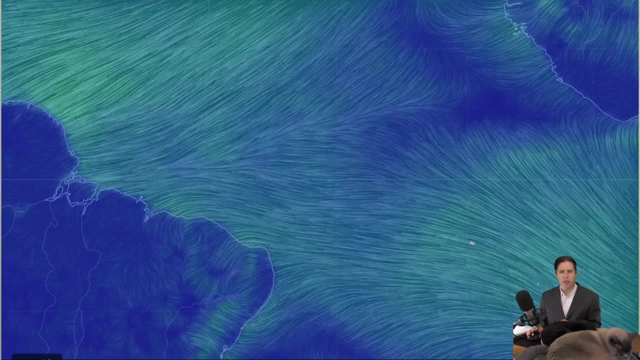 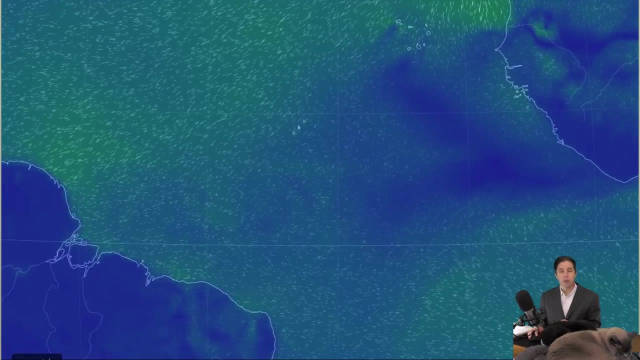 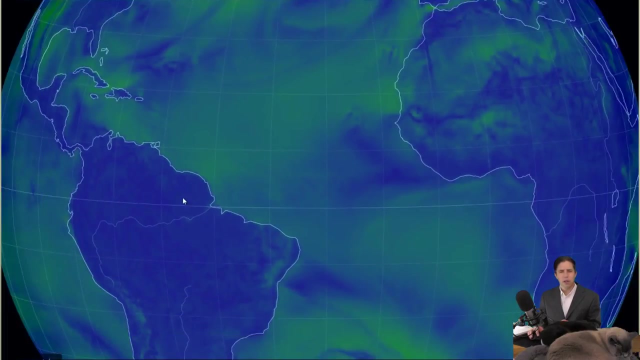 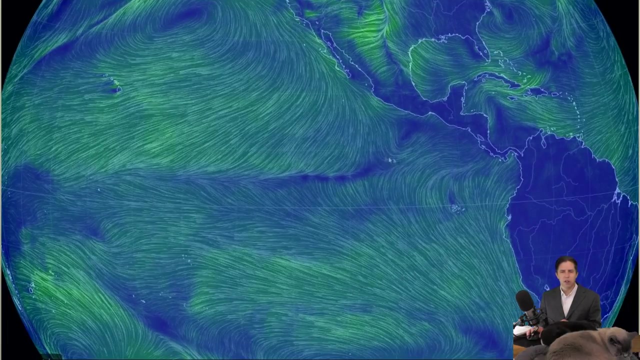 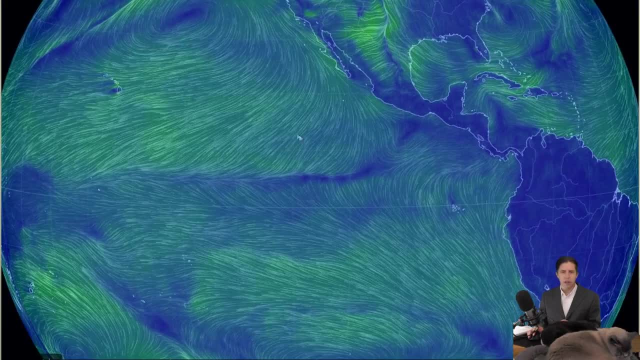 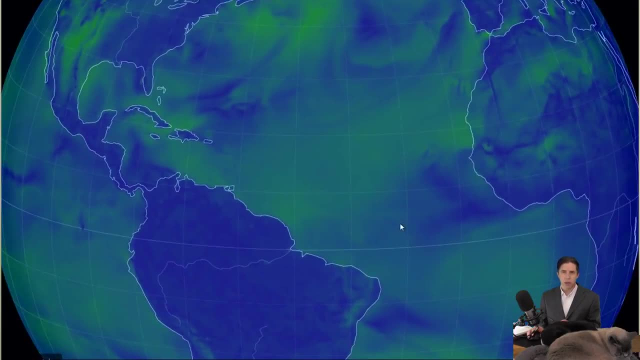 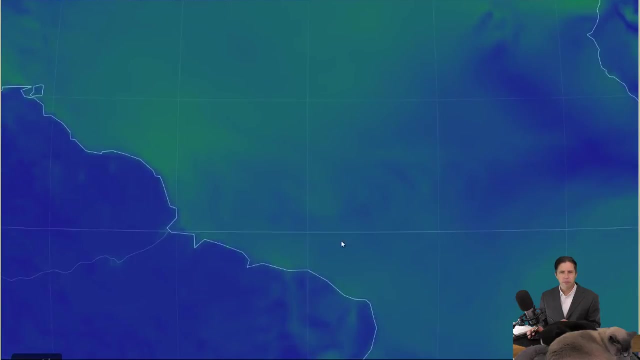 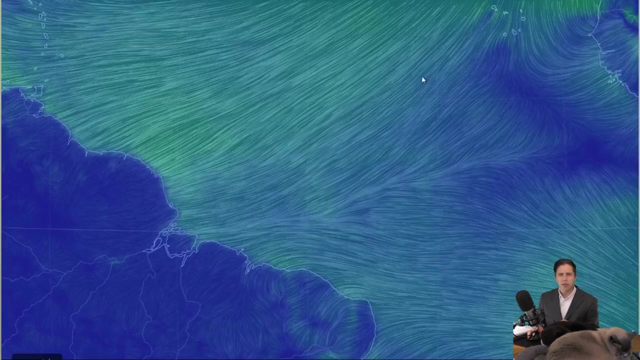 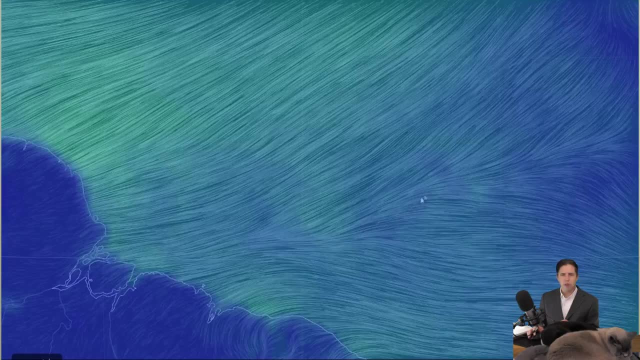 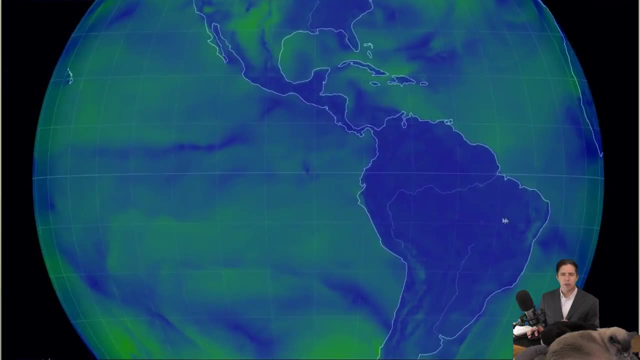 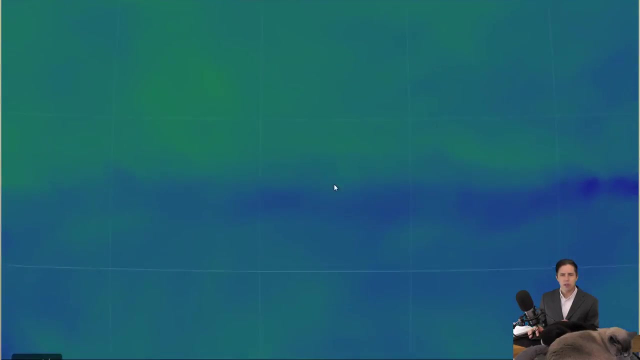 And you can see right in here, right through there, they are running into each other. In other words, they are converging. And if I look over here in the Pacific, I can see something similar. Let me go right over in here. 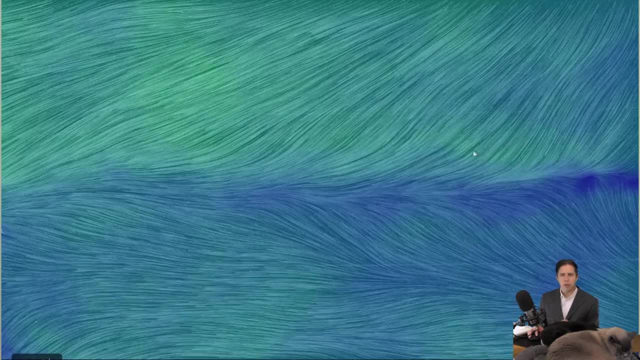 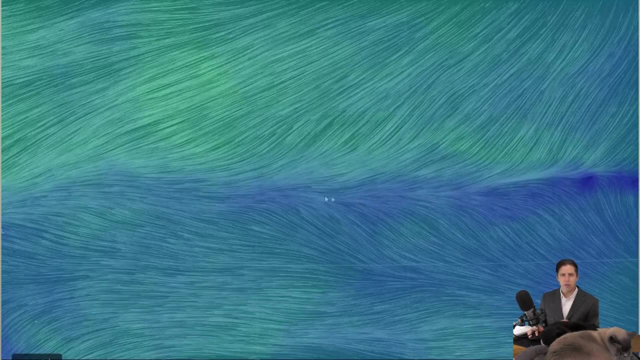 So that line, right there, is our equator, And we've got winds coming down from the northeast, winds coming up from the southeast, And they are colliding with each other along this zone right through here. So that's called a convergence zone. 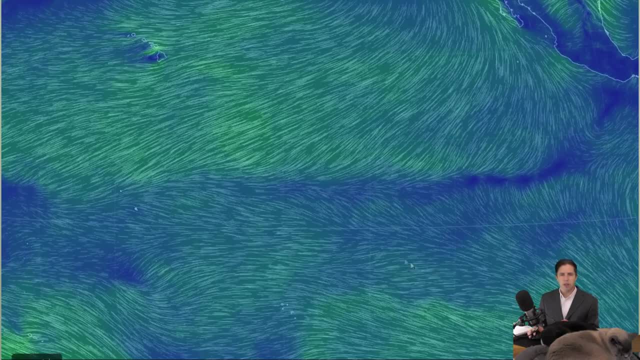 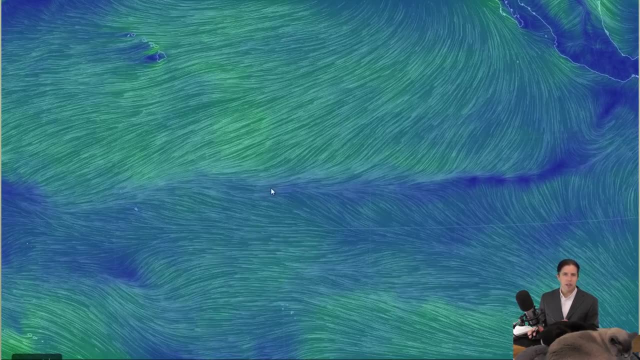 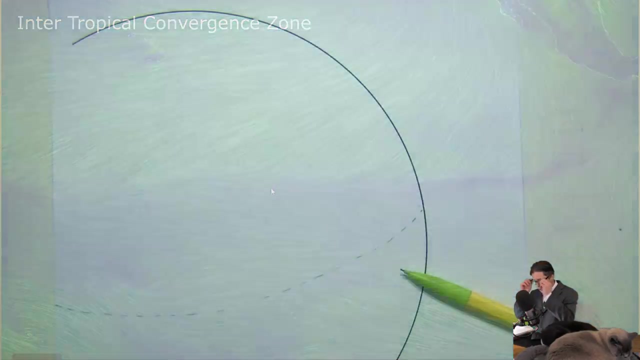 And, in fact, this whole area where winds from the southern hemisphere and winds from the northern hemisphere are coming together near the equator and converging. that's called the intertropical convergence zone. Okay, now I'm going to go back and forth between that animation and this drawing here that I'm going to make. 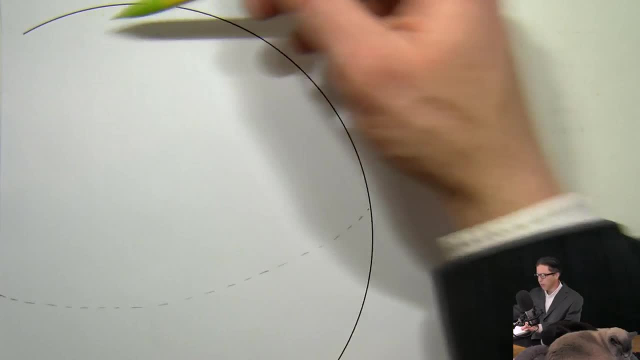 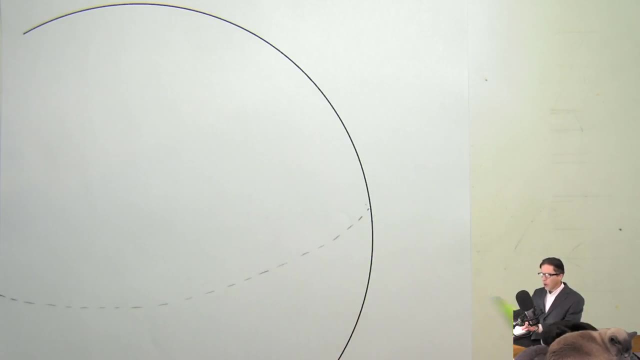 So right now, what I've got is I'm trying to draw the Earth big circle and I've sketched in the equator here. So what I'm going to add to this is what we just saw. So we've got winds that are coming down from the east and they are converging. 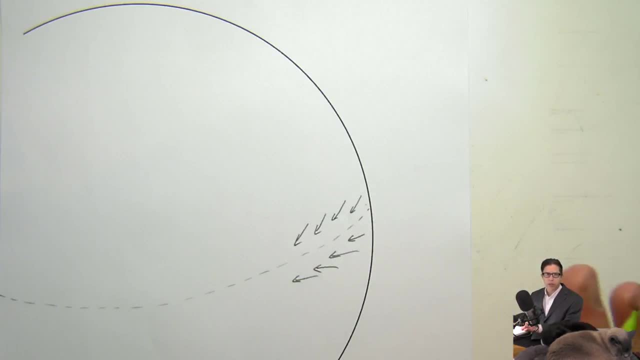 And they're not doing it right on the equator, but we're kind of close to the equator. This zone, It's called the ITCZ intertropical convergence zone. So this is happening all along the equator. I'm not going to draw it all the way across, but you get the point. 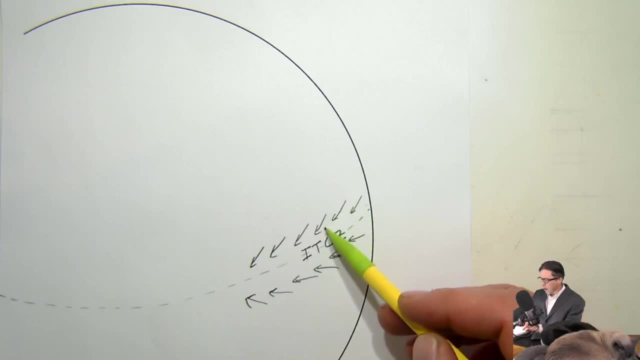 So if you've got winds that are coming from the north-ish and winds that are coming from the south-ish- and they both have a They're coming from the east- then they're going to combine And collide. they've got to go somewhere, right. 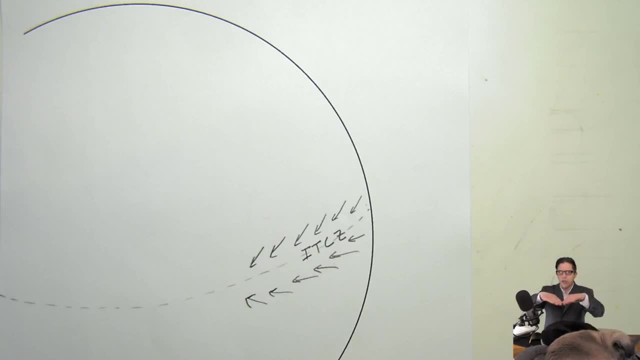 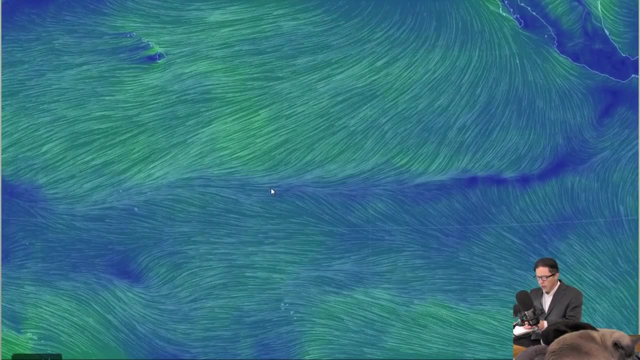 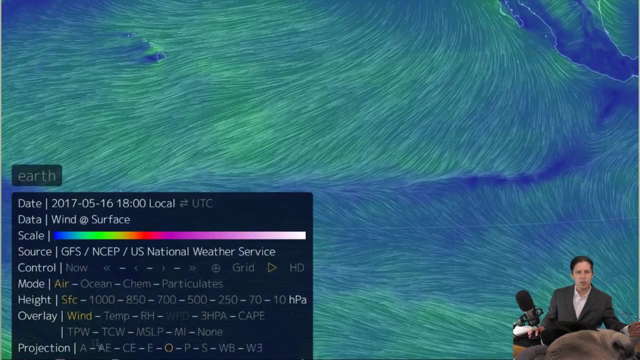 If you've got two sources of wind coming together and they hit each other, they can't go down, So the only option is to go up. Now what that does. Let's go back here And I'm going to change this to temperature. 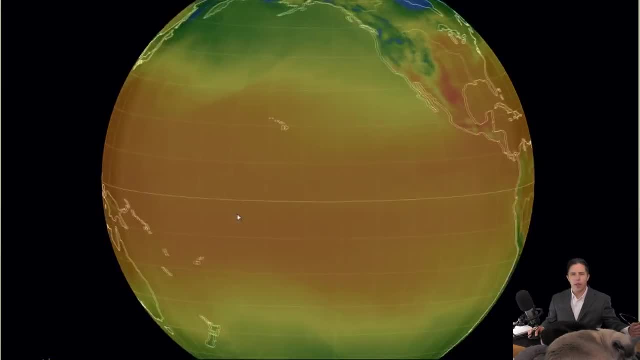 And so now we've. So the colors now represent temperature, And you notice that we have this band of really warm water, which is represented by this orange color, all along this area that we're calling the tropical intertropical convergence zone. 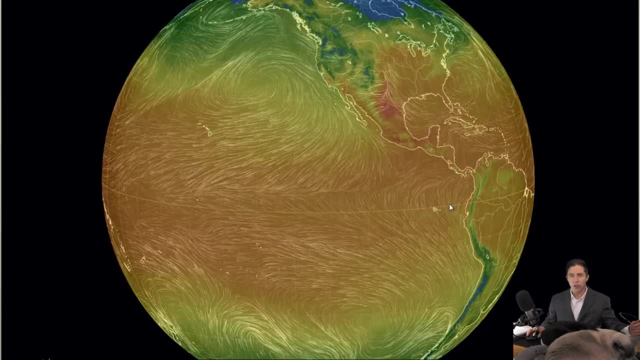 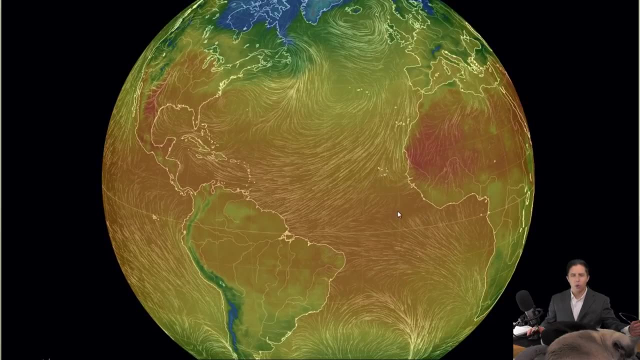 All the winds in that orange zone sort of have an easterly trajectory right. They're coming out of the east And we see this over here in the Atlantic. Okay, So we've got really warm water And then we've got winds that are converging. 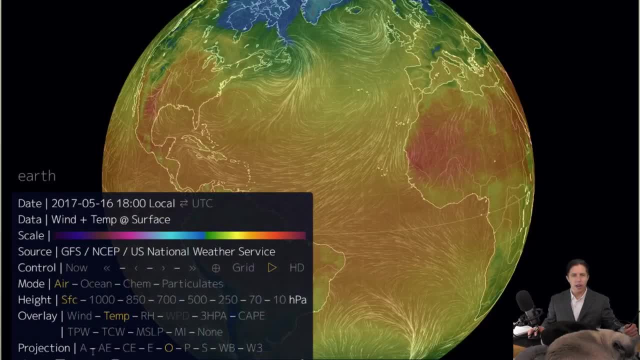 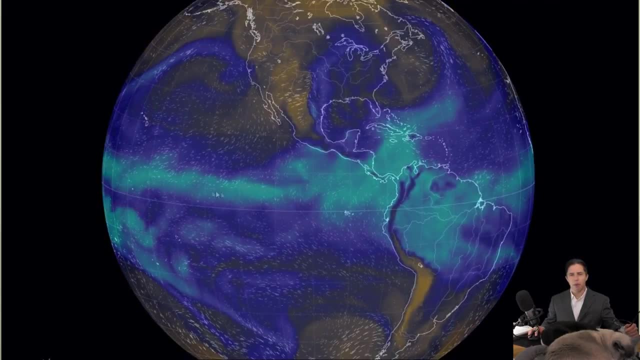 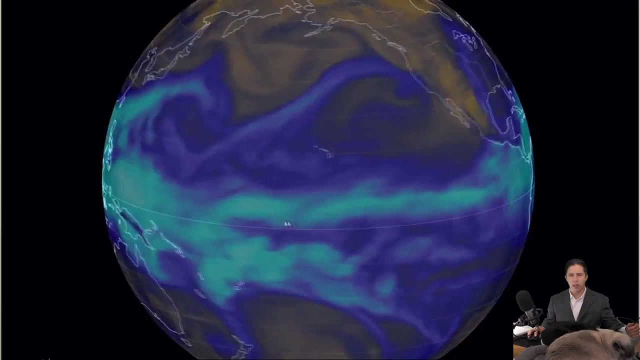 And then if I go and look at total precipitable water- we've done this before in a previous lecture- we see that there is a band of really high dew point air, air that's really high in humidity. So these aqua colors would represent air with really high mixing ratios, or dew points. 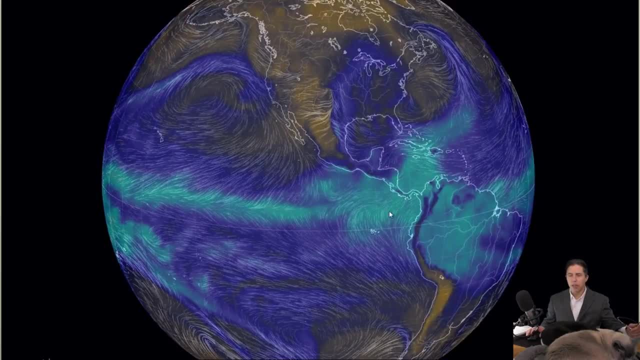 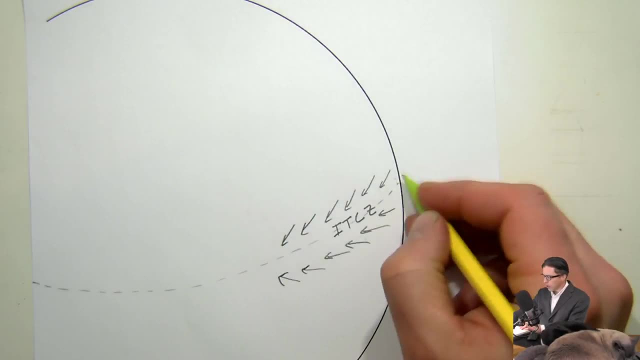 So we've got air that's warm, it's very humid, and you've got converging winds. Okay, So all of those things mean that this wind, when it converges, has to rise, And I'm going to draw that kind of coming off the edge of the earth out into space here. 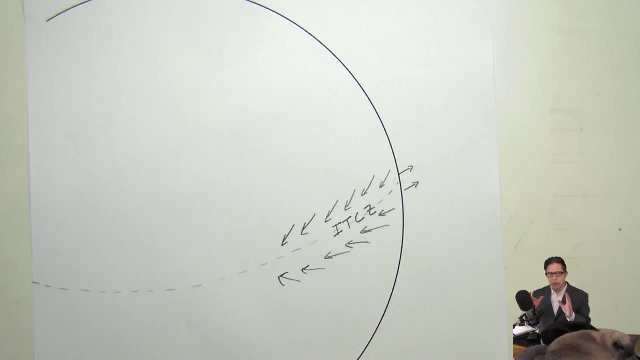 And they're the perfect conditions for making convective weather cumulonimbus. So I'm going to draw a big cumulonimbus Now. I am greatly, greatly exaggerating the size of this thing because, if this was true, to scale. 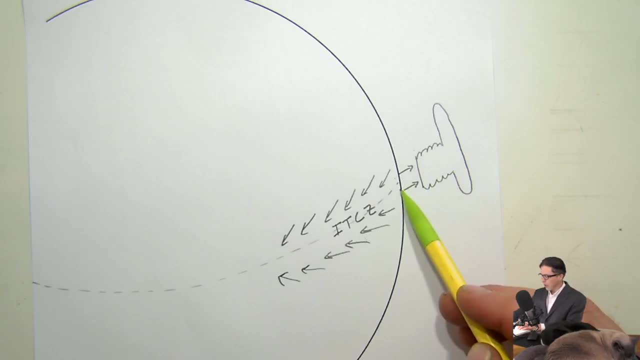 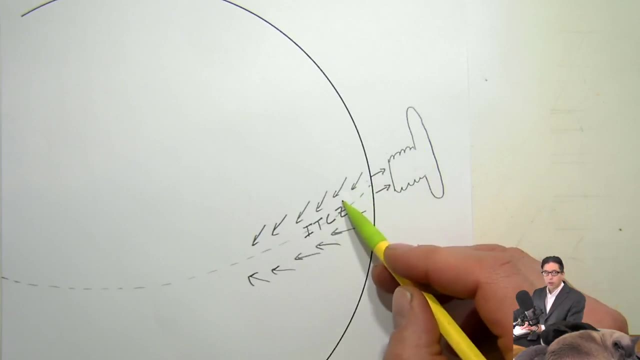 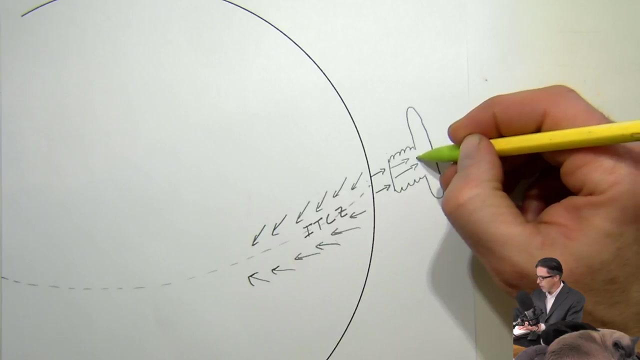 the entire Atmosphere would be the thickness of this line, right? So I'm just doing this for illustration. So when winds come together in the convergence zone, they have to go somewhere, So they go up, and they go up through this cumulonimbus. 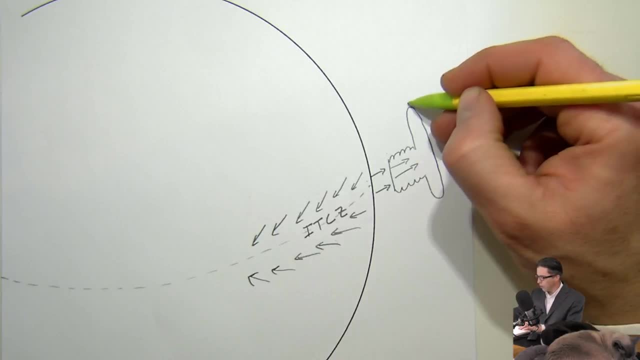 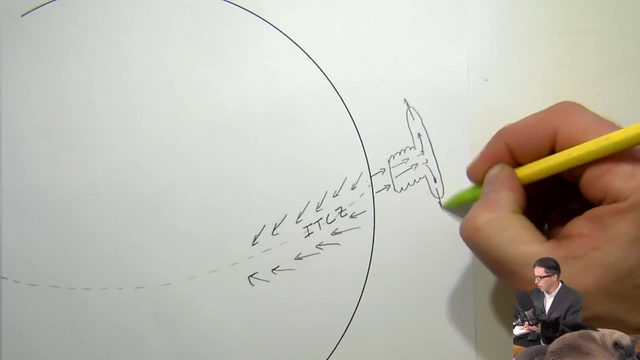 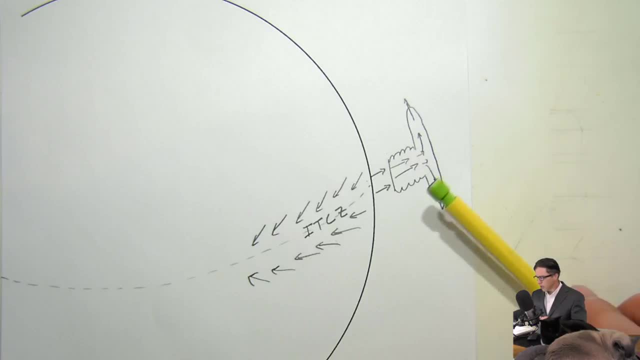 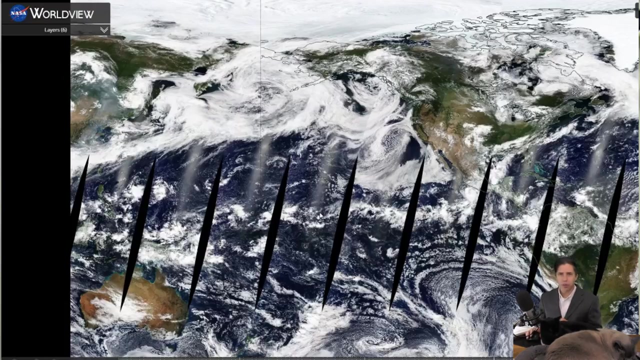 Okay, Okay, Okay, Perfect, Perfect conditions among the ITCZ to form cumulonimbus, And we can see the effects of this in a couple different ways. So for one thing I'm going to go to this is the worldview site that we've seen a couple 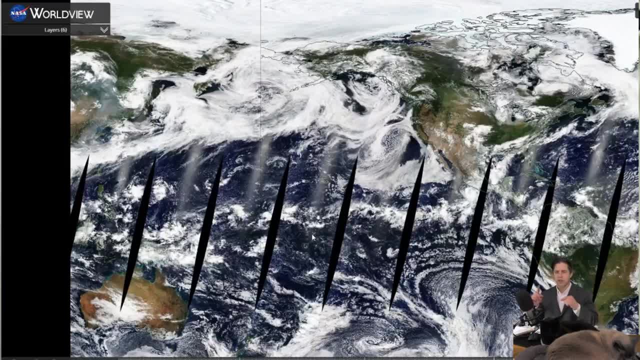 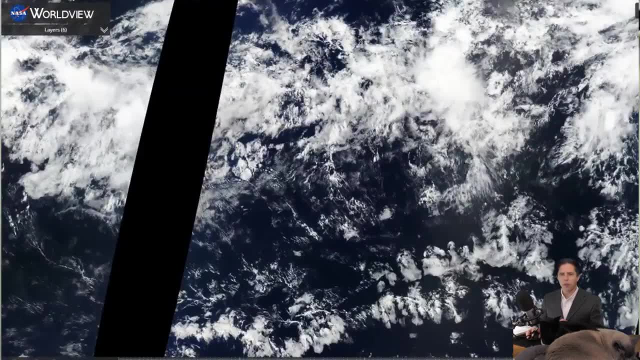 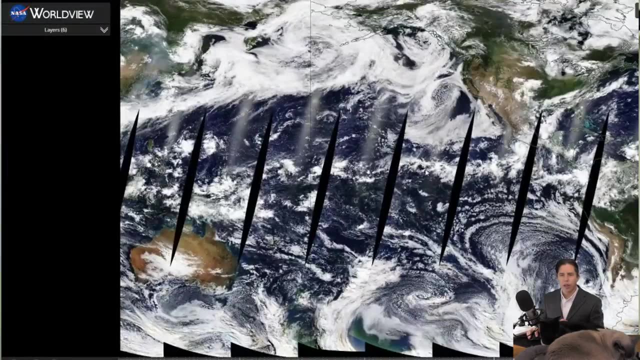 times now, And, just to remind you, there are two satellites that orbit on the opposite sides of the planet at all times and they make these images by taking stripes that each satellite makes and they stitch them together and the satellites miss a little bit. here in the middle that's black, right? okay? so look at the big. 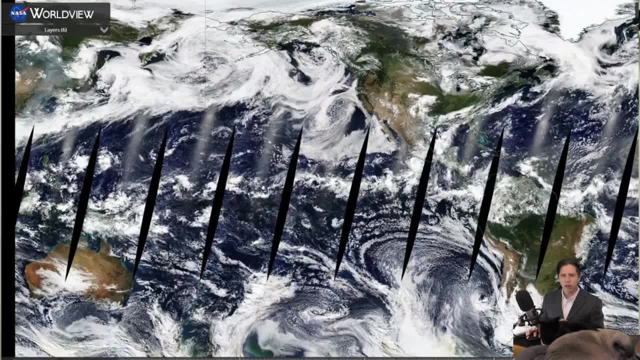 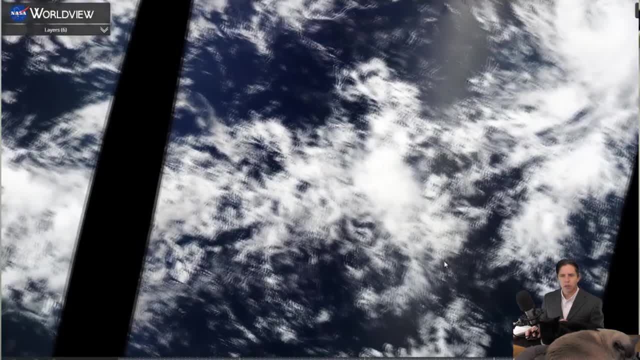 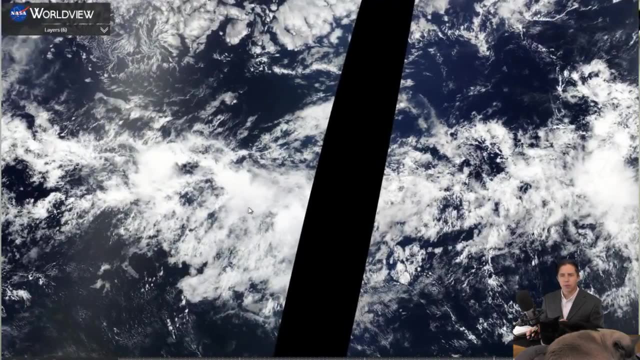 picture here. i see that right here, right through there, there's this kind of band of white. i'm gonna zoom in a little bit. so these clusters that you see, they're kind of roundish. these are all giant clusters of cumulonimbus. this is where the itcz is occurring today and it's occurring right around. 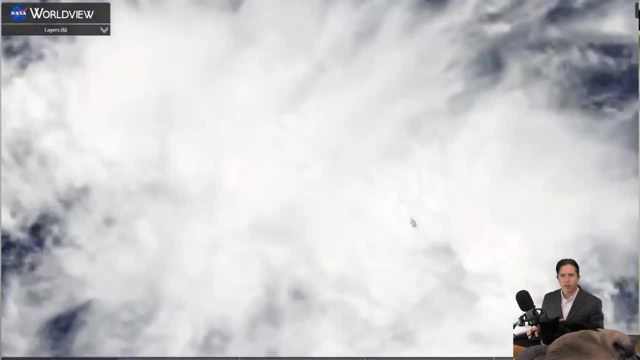 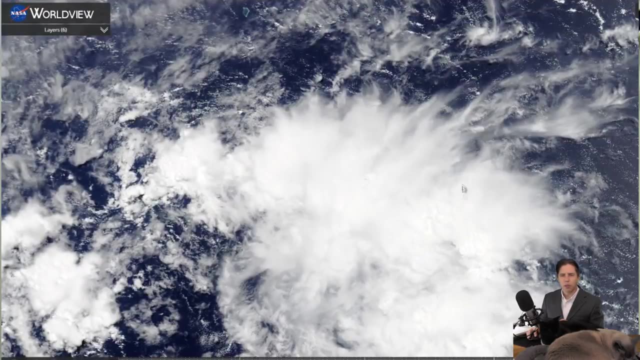 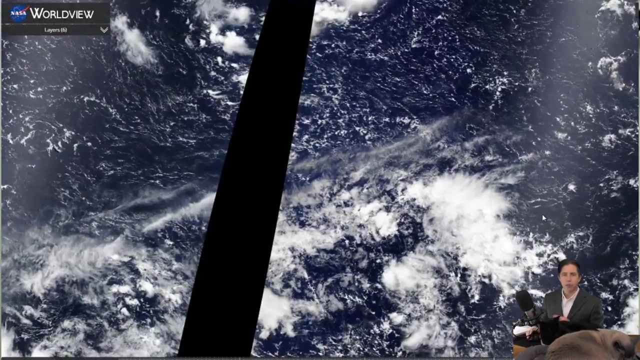 there. i'll zoom in over here and you can see, zoom in a little bit- that's the ice coming from the anvil, right? so you've got a big cluster of cumulonimbus here and the fuzziness is the ice from the anvil. that's kind of floating off, okay, so that's one way we can look at it. i'm going to 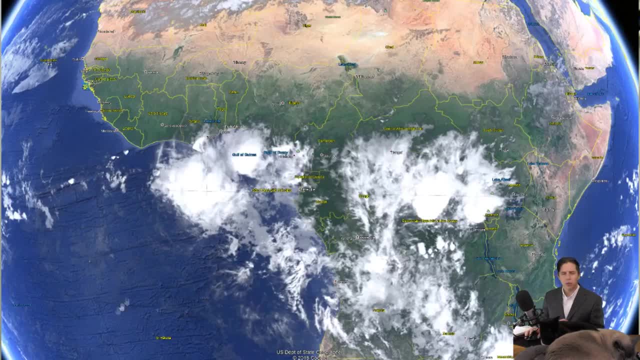 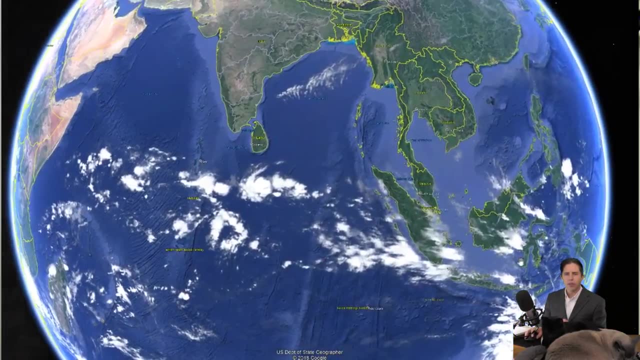 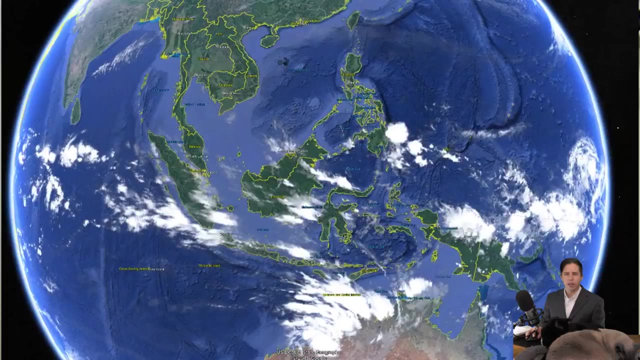 change my tool, you, you, and right now i'm going to look at google earth, and i'm looking at the google earth cloud layer, and this uses a different type of technology to show clouds and, for one thing, there's a lot less clouds here to look at, and so what we're looking at here is something called an infrared. 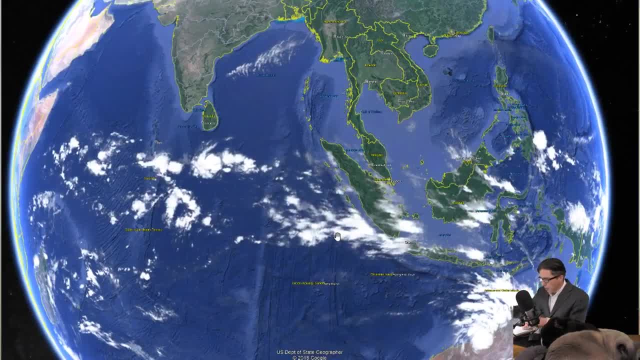 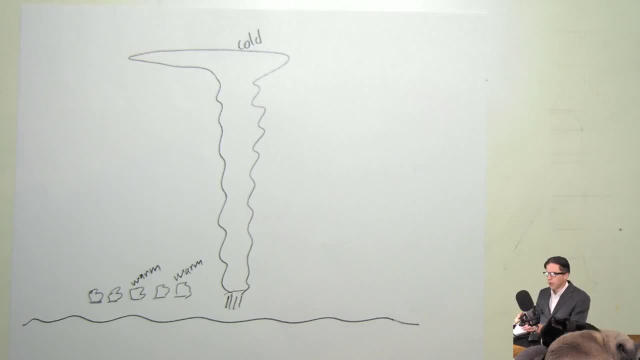 image. so let me explain what that means. what that means. so clouds, imagine we've got the ocean and we were thinking, if we think about the temperatures of the tops of the clouds, okay, we've got a bunch of stratocumulus. let's say, maybe we've got some fog. 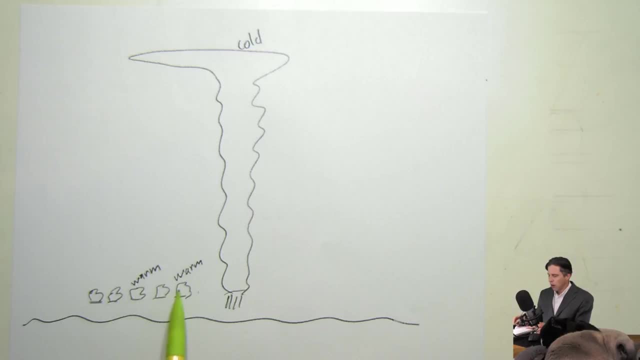 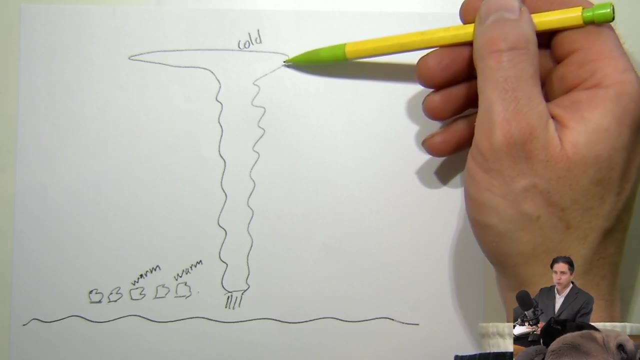 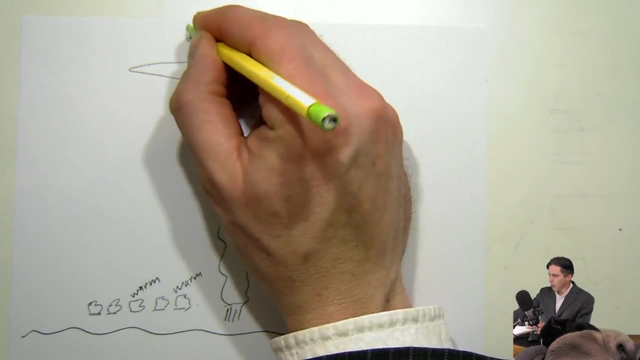 the tops of the temperatures of those clouds are going to be fairly warm compared to the tops of really tall clouds like cumulonimbus, right, so if you had a satellite that's up here and circles around the earth and these clouds and so on and so forth, so this way we can see. 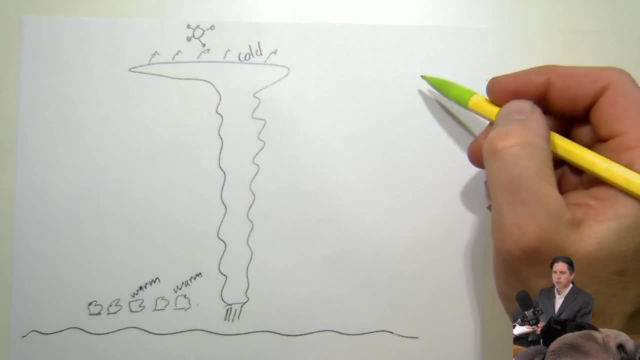 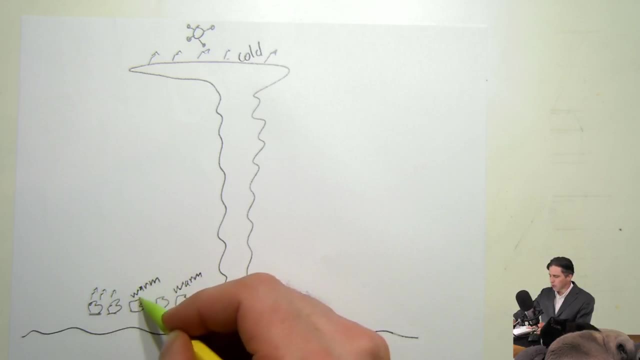 if we're looking at the observer on what we're looking at, it's going around the earth looking for temperatures and it's measuring the temperature, say, of this cumulonimbus, it's going to see a very cold temperature, whereas if it looks at the bottom or, i'm sorry, the tops of the stratocumulus clouds, it's going to see a much. 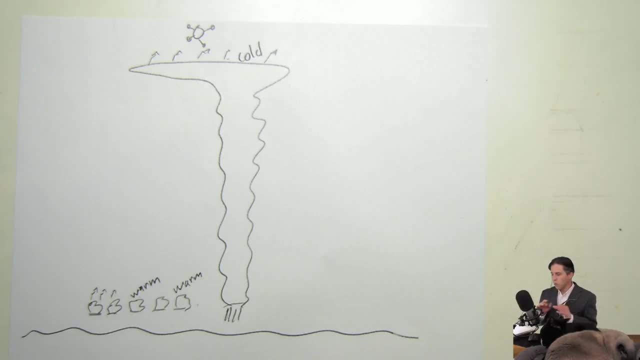 warmer temperature. so these satellites as they're going over, they're actually just measuring. taking pictures of clouds in the infrared is that you don't need daylight so you can see them in the dark, and the other advantage is that if you're just interested in the cold areas, that means you 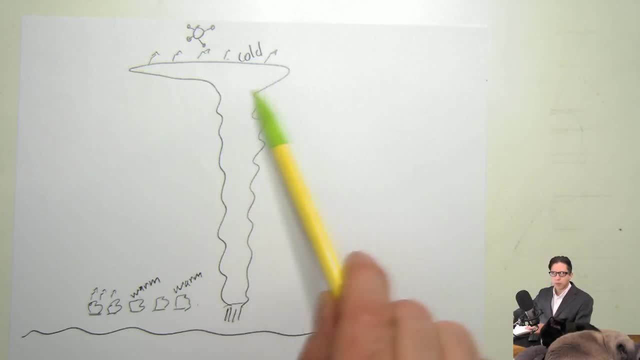 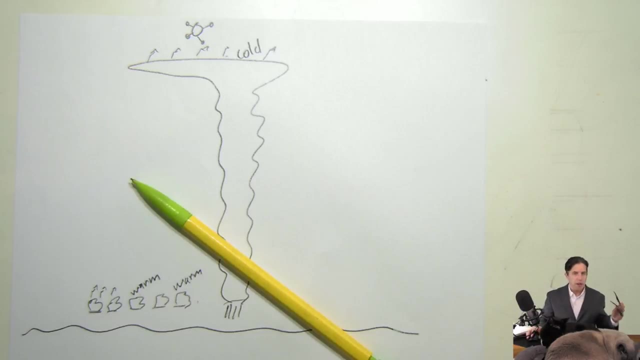 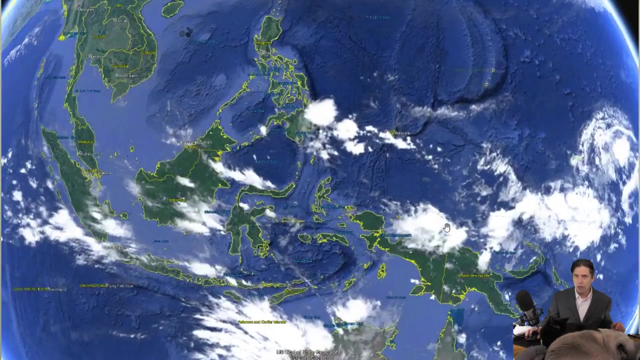 will only get these cold cloud top temperatures, and the satellite will ignore all of this stuff. okay, so that's what's happening here in google earth. uh, what we're looking at are places where the clouds are very cold, which means they're very tall right, so we have managed to filter out. 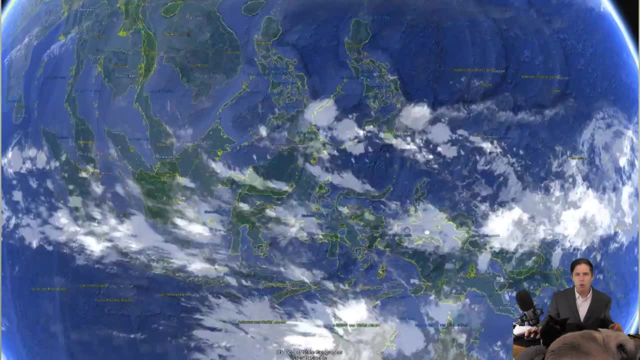 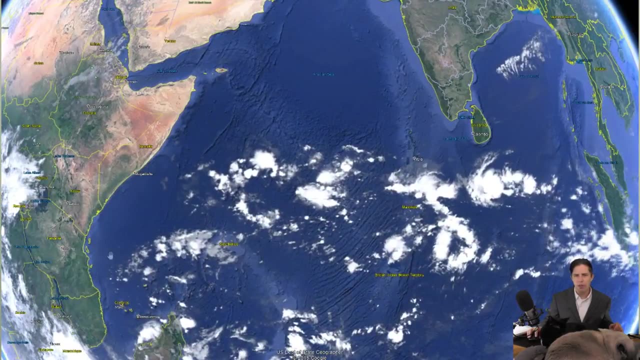 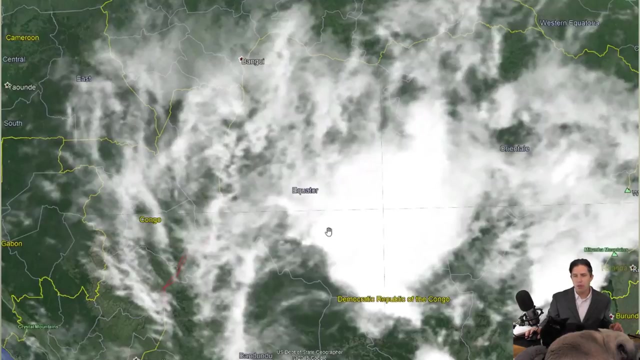 all the low level clouds. so we kind of see here there's a band. so we're going across the indian ocean, here we see a band of these white blobs, a bunch of them here in central africa and these are giant clusters of cumulonimbus along the itcz and you have to realize how big these things are. 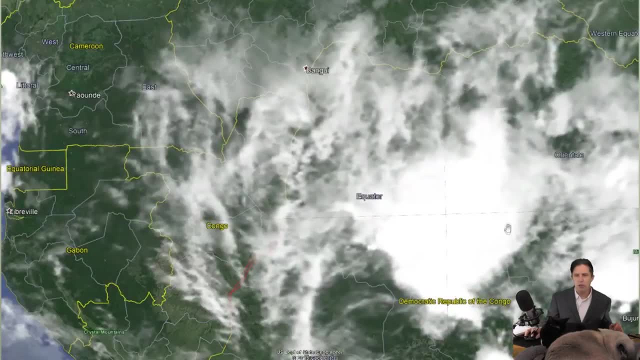 like this thing right here would be the size of several large us states. right? if this thing was on- let's say we just pick this up and put it over the middle of the country, united states- it would be breaking all kinds of precipitation records. i mean, they're going to get several inches of rain out of each. 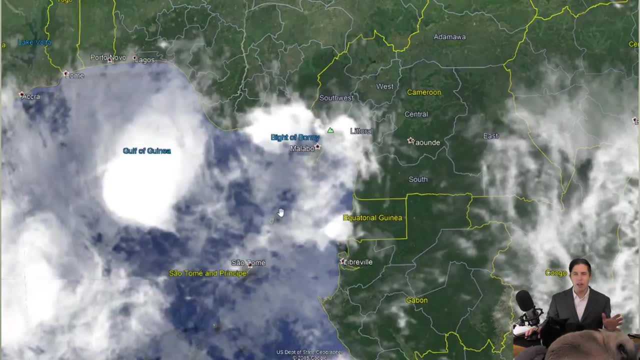 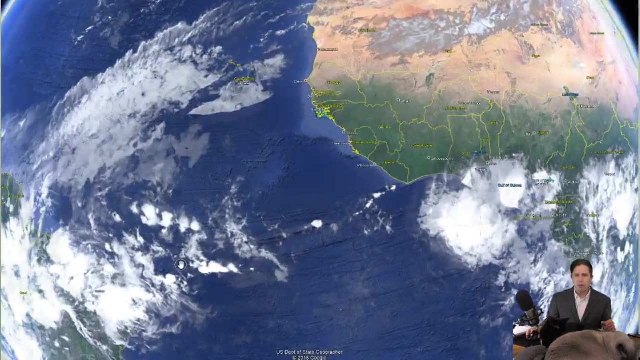 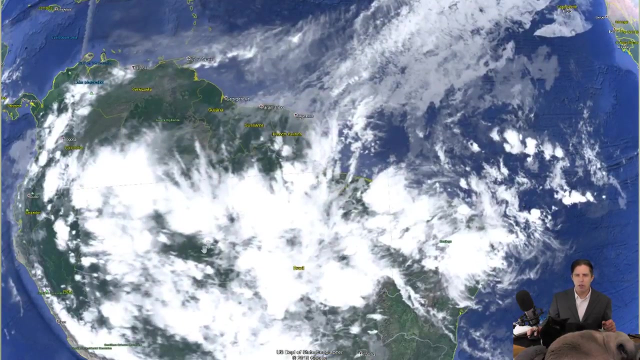 one of these blobs that you see here, and this is happening every day along the equator, along this itcz zone, and i zoom out a little bit, okay, so i kind of fall apart there, but then it comes back a lot of activity here over central south america and 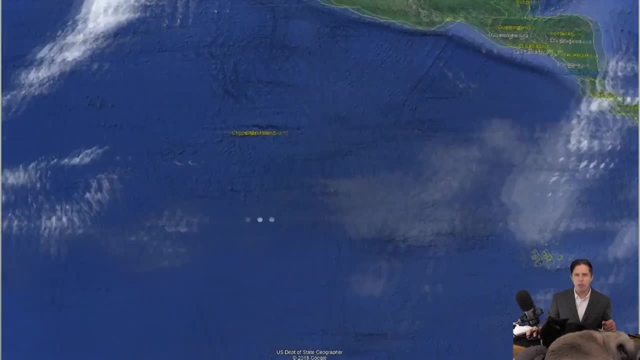 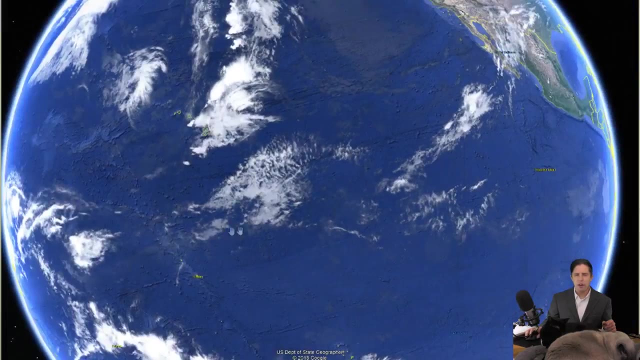 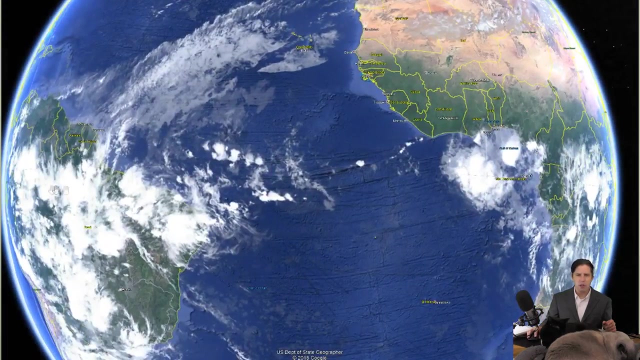 we don't have. it's not very well established today, but many days you'll see a string of cumulonimbus across the pacific, kind of right in here, and it varies day to day. so the actual activity, the itcz, varies day to day. so today it looks like you can see it quite a bit over there. 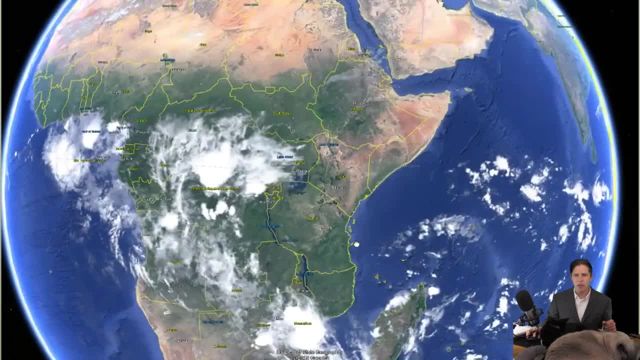 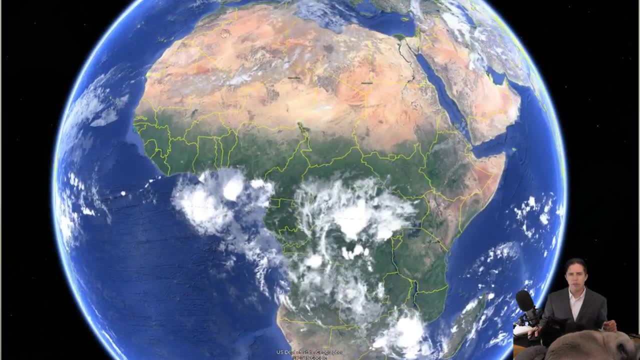 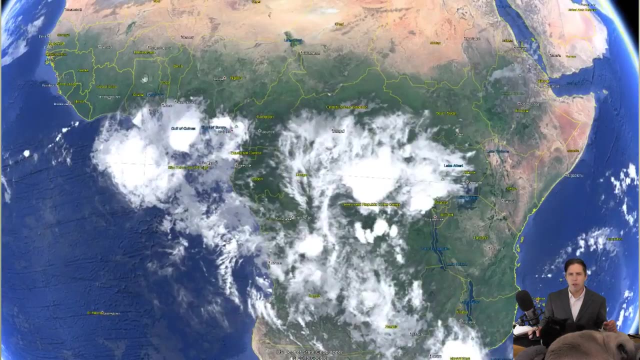 central south america, central south america, and then you have a string of cumulonimbus across the central africa also. notice why i've got africa up. notice that northern africa very, very dry, very brown. south tip of africa very dry, very brown. central africa very green, and the reason is that 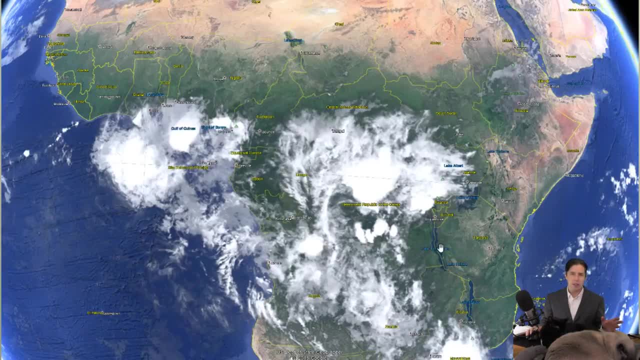 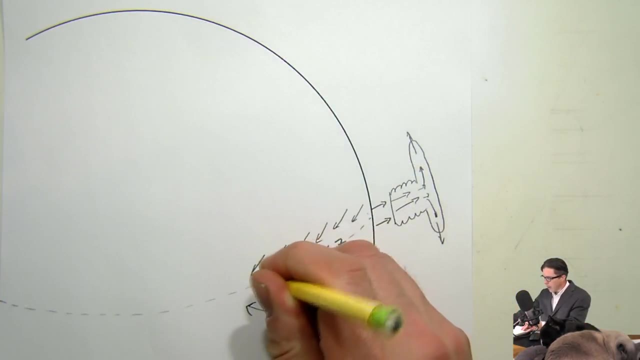 it's the central part of africa, resides in the itcz, so they get these tremendous thunderstorms. you know, like i said, almost every day, where they get inches of rain at a time. so let's return to our drawing here and we can add in- i'm going to add in a bunch of 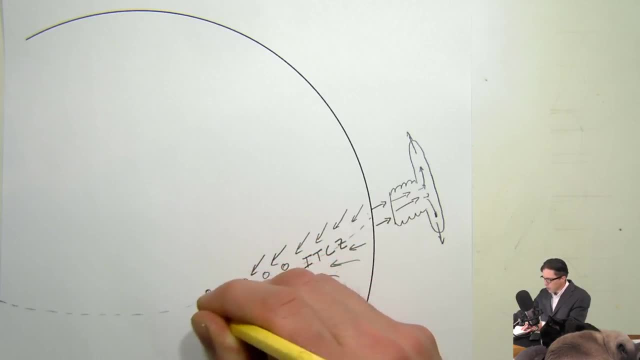 circles to represent these cumulonimbus right all along the equator here in this endotropical convergence zone. so these again extend all the way around the equator. i'm just not going to draw them all. we can also see some other evidence from the central south africa and we can see that the central south africa is. 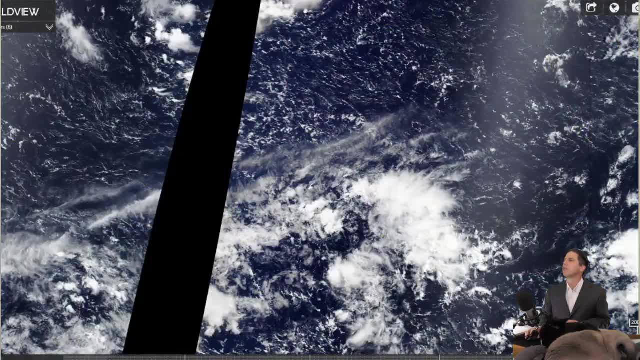 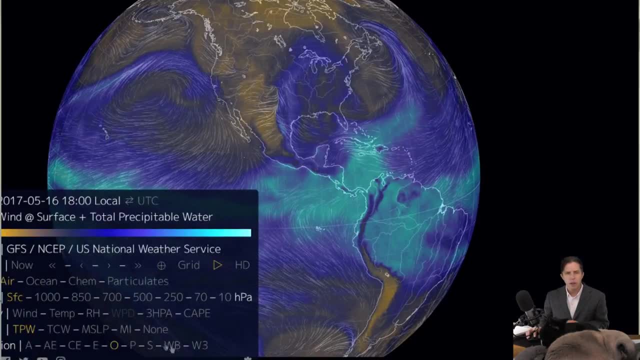 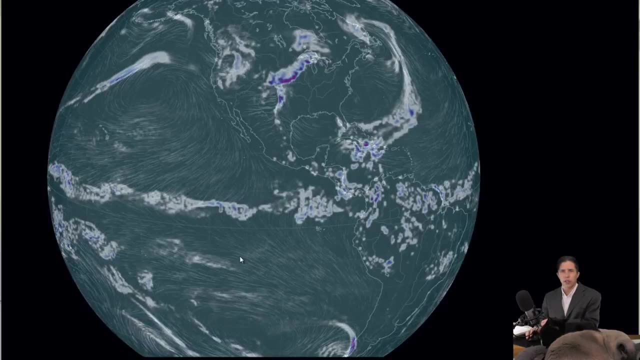 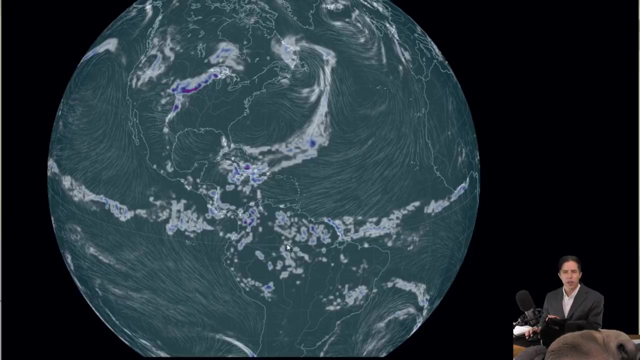 here, right located in the east west hand delta, that each of our throwing from this, so we can see that it's a well- hot constant and you see that pretty clear flammability within one still surface area. so you can see that it's all enough's left for a fundamental type of footage. but really i singled out that. 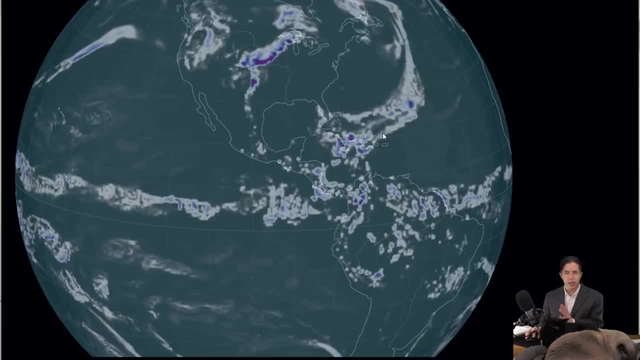 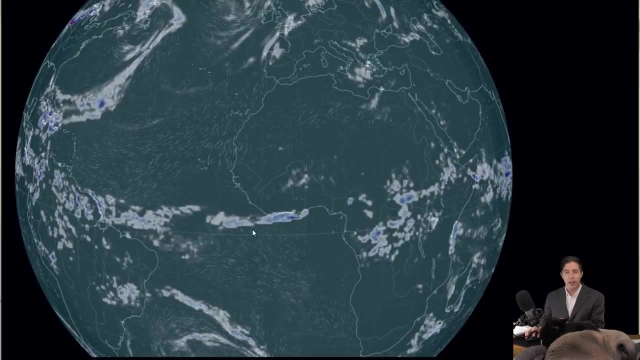 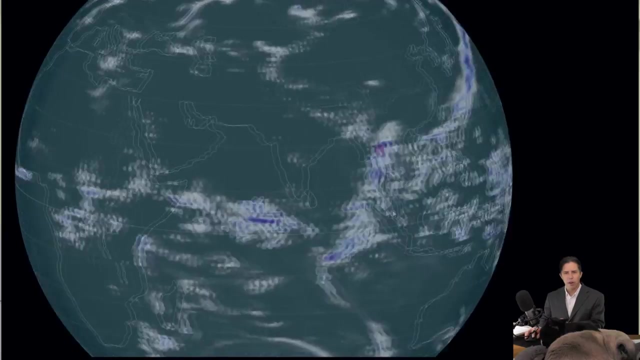 one to to talk about is what we were just looking at: the ITCZ. see this band right here, going right through the right kind of along the equator. that's the ITCZ. those are all blobs of precipitation that are from cumulonimbus. here it gets, uh, it gets pretty broad here and there's a kind of splits. 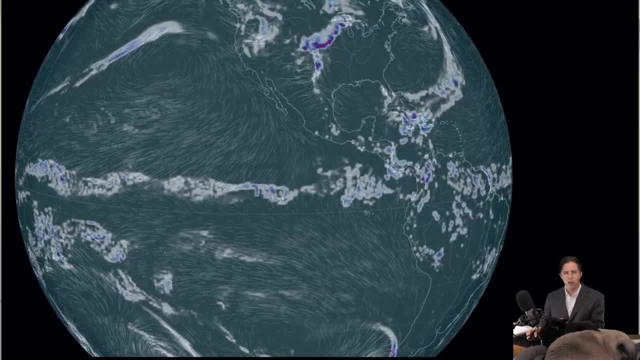 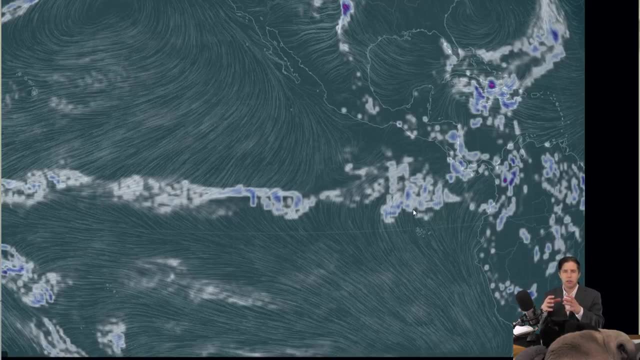 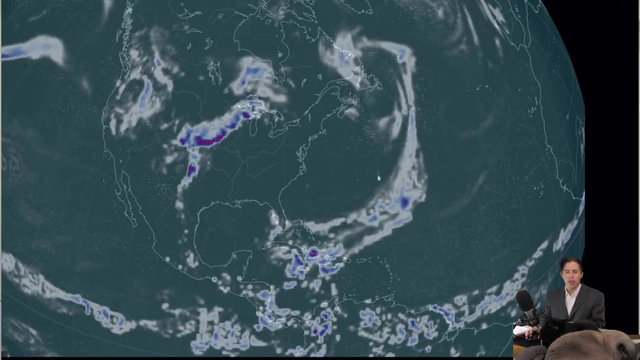 into two. but then if you go back pacific ocean, there's kind of a narrow band there. all those are little little blobs. you know, cumulonimbus makes a fairly uh narrow blob of precipitation right. so that's what we're seeing now. while we're at it, we can see some totally different. 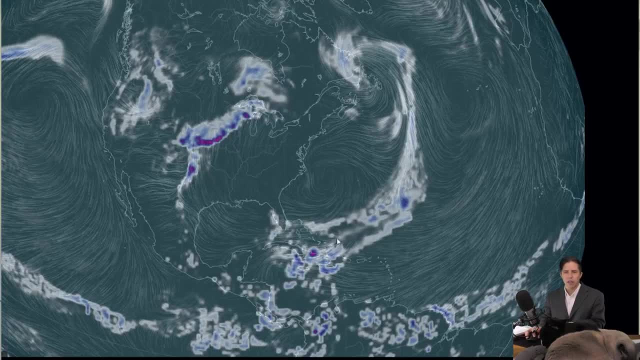 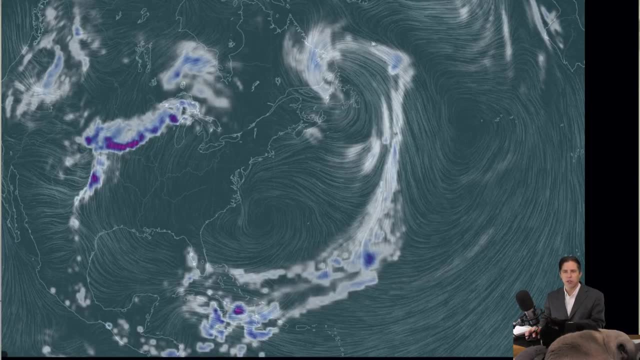 types of precipitation. see that, do you know what that is? so that's that classic comma shape, that's a mid-latitude cycle and that's the precipitation that was produced in the last three hours from a mid-latitude cycle, and you can see the counterclockwise swirling. 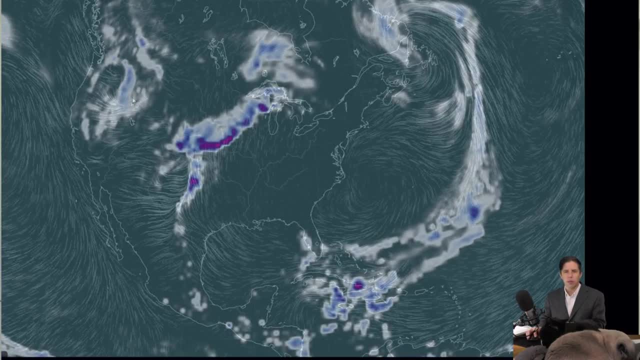 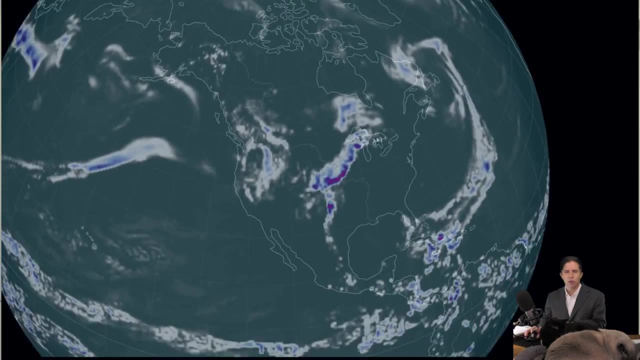 of the wind. there's another one that's a little harder to see, but it kind of has a comma shape. that's a mid-latitude cyclone. this is another one that's a weird shape, and if we go around the world we can see more of those comma shaped things. those are the mid-latitude cyclones, but for now, 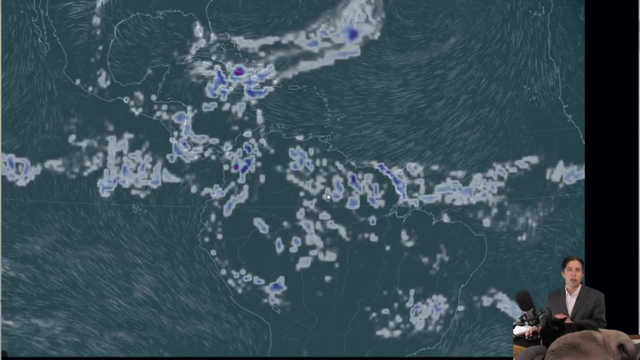 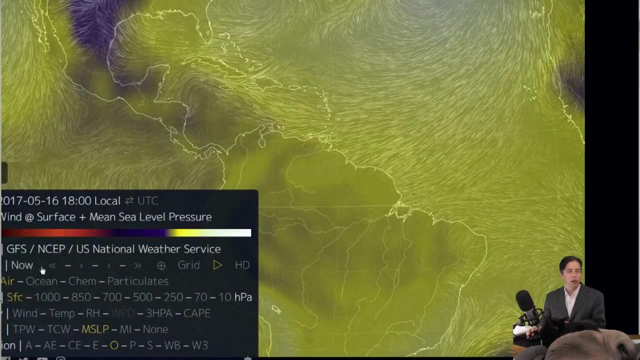 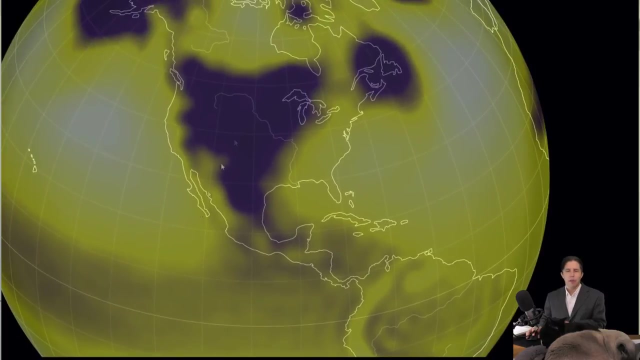 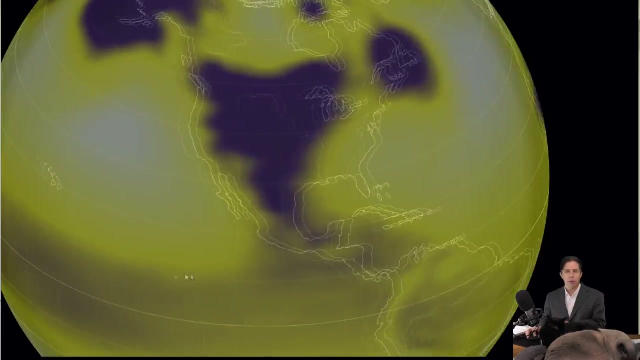 what we're talking about is the, the activity along the equator, along the ITCZ also. I'm going to give you a little bit of record of what's happening. so to remind you, purple means low pressure, the whitish color means high pressure and back. when we talked about this, I did this before when I showed 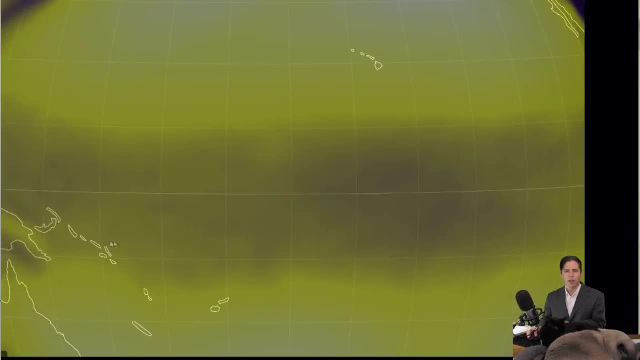 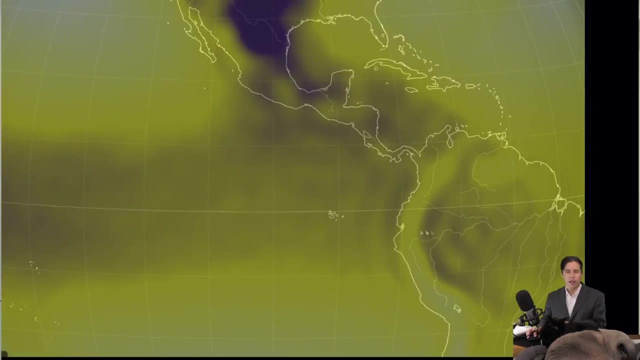 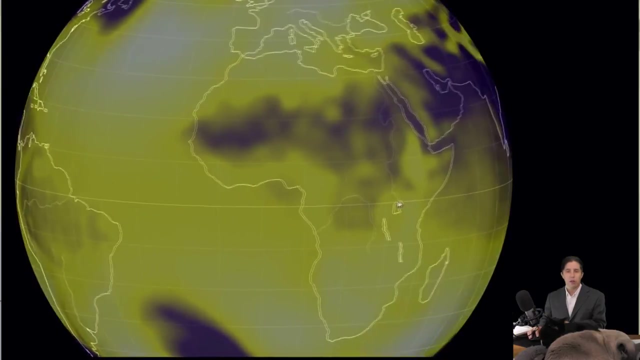 this to you, and I said that. notice that there's a purplish band around the equator, and this is due to the fact the air is rising every day along the equator now- and I use this as an example of a thermal low- and the dew point is so high that you get convection every day and that 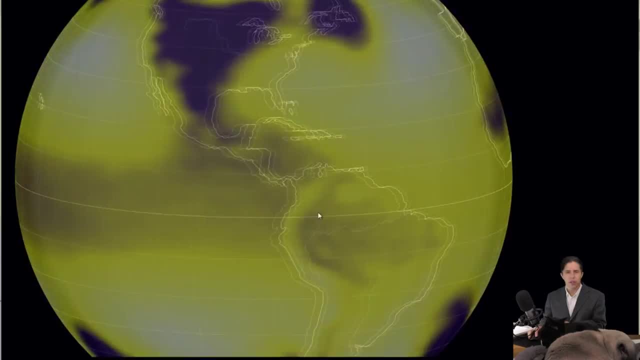 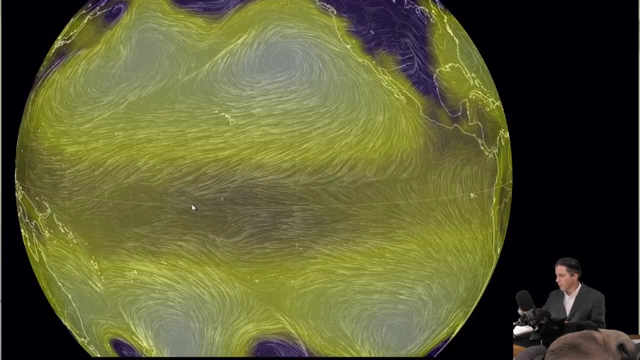 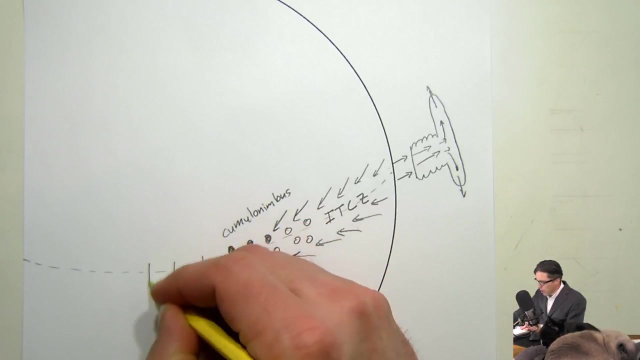 produces lower pressure at the surface. so we can see it on this one pretty well over the Pacific on this day: a big band, a fairly low pressure. so I'm going to add that and I'm going to add some L's here to remind myself that this is a. 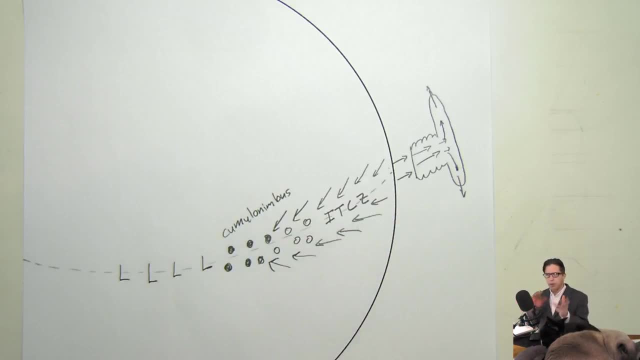 band of low pressure. so again, these features are all the way around the earth. you've got converging winds, you accumulate limbus, you've got low pressure, all these things. I'm just drawing them in little chunks here, but they would go all the way around the earth, okay. so if the air rises, and again this is happening all the way around the earth, where you have these rising plumes of air that turn into cumulonimbus and then that air hits the stratosphere and it can't go into the stratosphere because the stratosphere has this big. 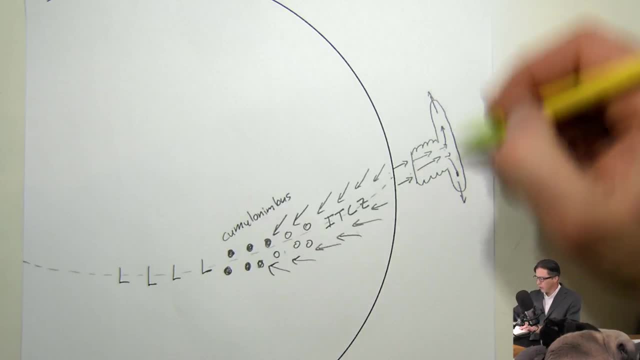 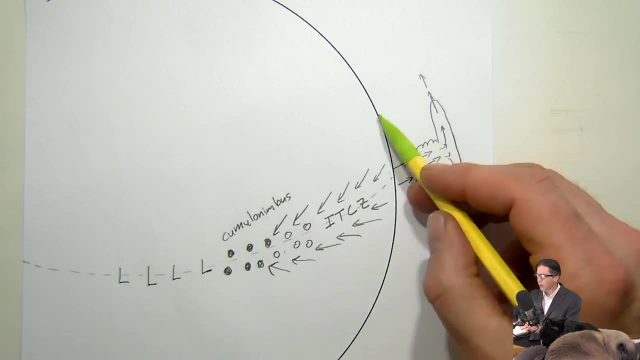 temperature there and then the air can't go into the stratosphere because the stratosphere has this big temperature, and then the air can't go into the inversion. it has to go somewhere. so some of it goes north, some of it goes south. now, as it goes north and south- and again i'm greatly exaggerating the height above the ground- 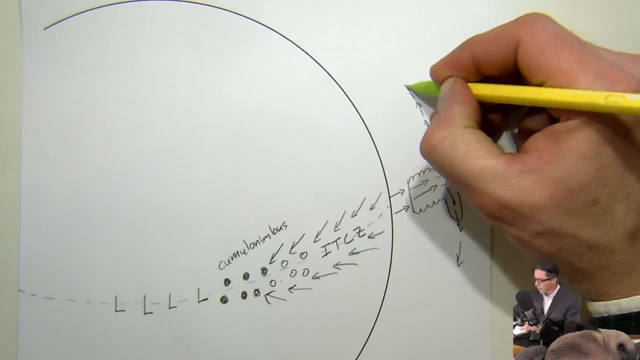 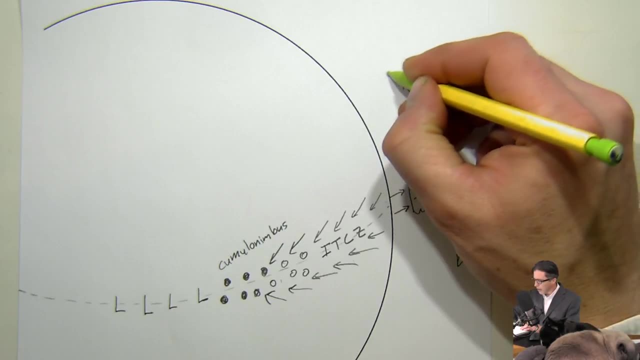 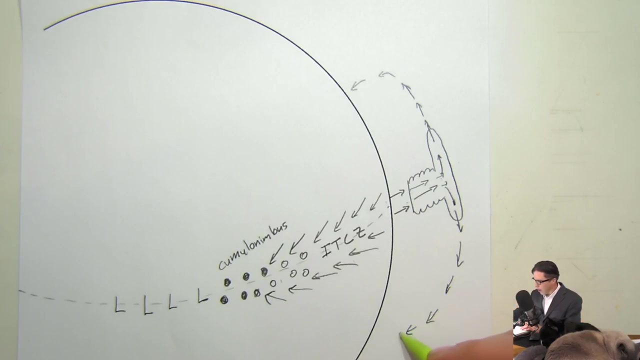 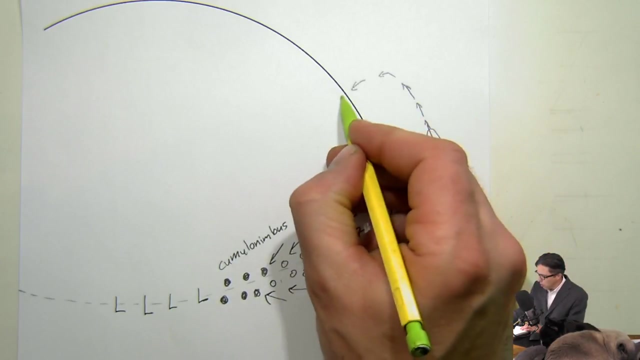 right. just keep that in mind. it travels for a while and it it's cooling. it's radiating energy out into space and it starts to cool and then it starts to come back down, and both north and south count the. the air that rose at the equator tends to come down right around, more or less. 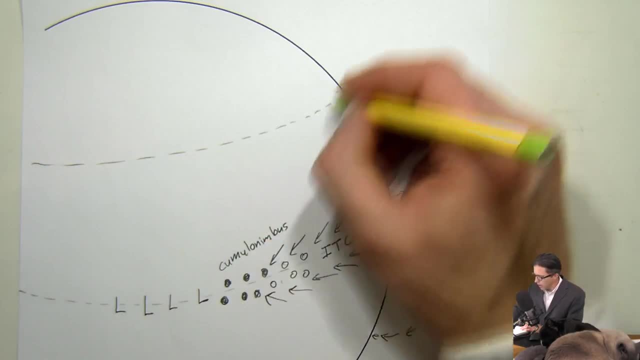 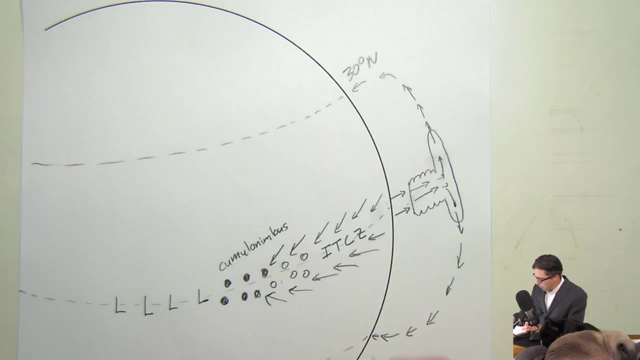 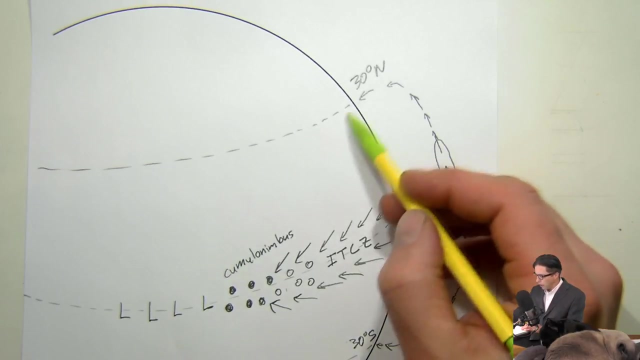 30 degrees north and 30 degrees south, so i'm going to put down 30 degrees, and then there's another zone, 30 degrees south, where this also happens. so let's think about- and i'm just going to basically ignore the- the southern hemisphere, but just realize that everything we're talking about today 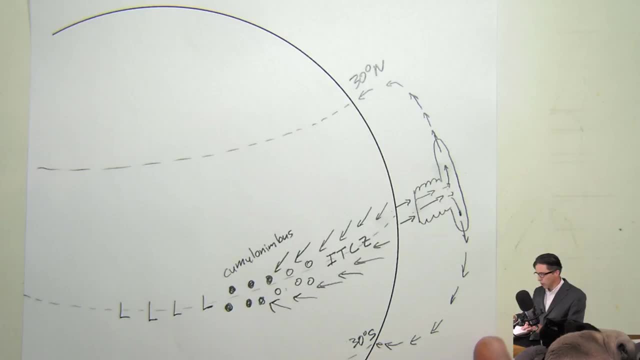 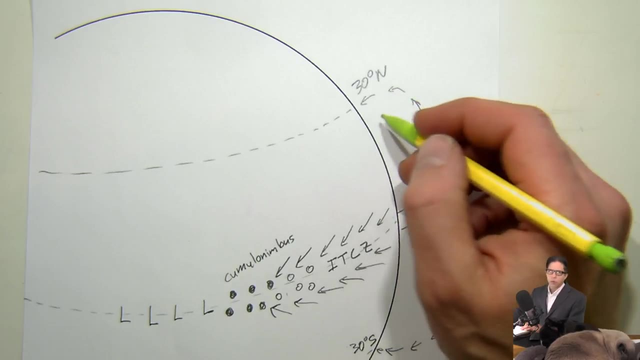 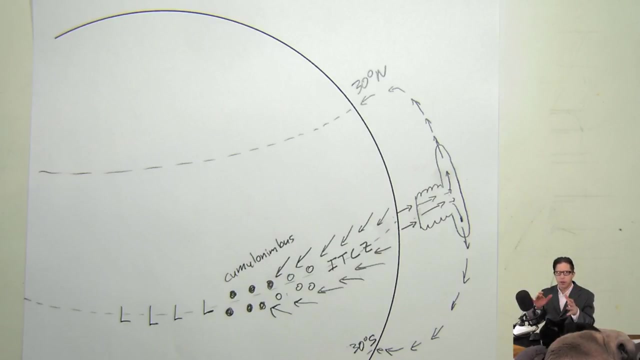 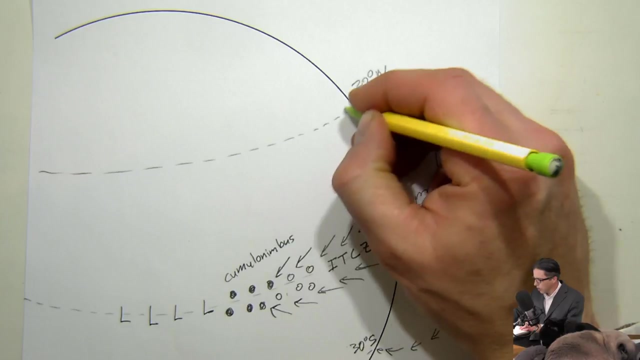 up in the northern hemisphere is happening also in the southern southern hemisphere. so, uh, here we have sinking air. so what does sinking air do? so if you have air sinking down from the upper parts of the atmosphere, that produces high pressure along the surface, right, so right here where this air is sinking, you would expect 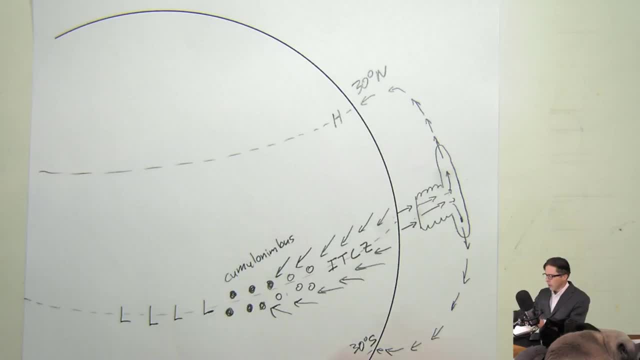 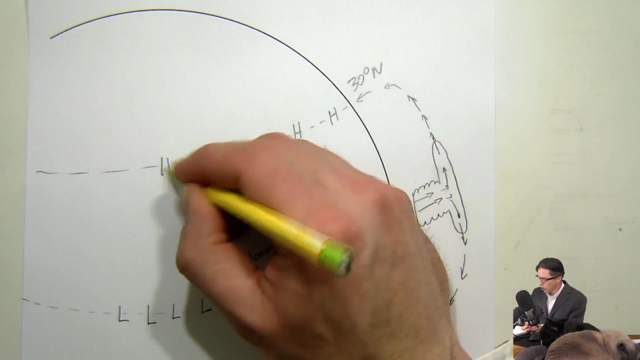 a high pressure and, in fact, if this pattern is happening all the way around the equator, you also have air that is sinking all the way around the 30 degree mark. so you would have a band, you would expect a band of high pressures going all the way across. now we have a name for these. 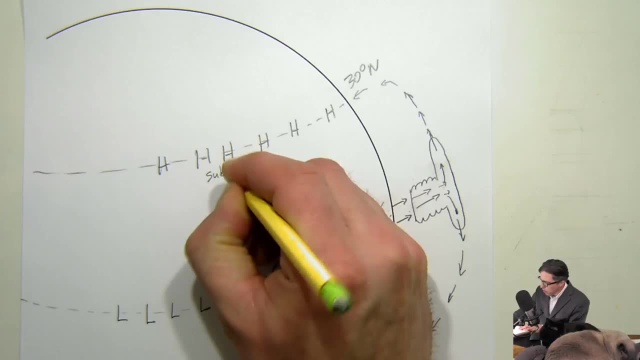 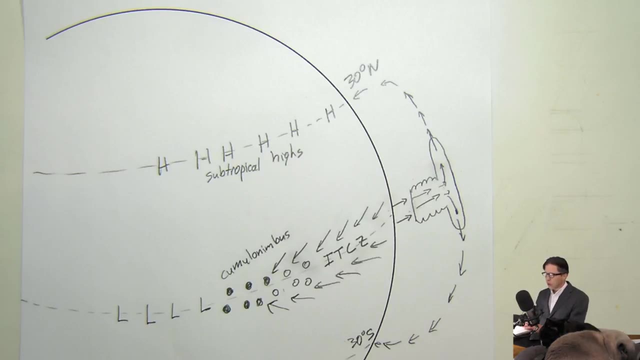 they are called the subtropical highs. okay, the subtropical highs. so if the earth was completely water and there was no continents, there'd be a lot more symmetry to the patterns we're talking about. we'd have a perfect band of cumulonimbus around the 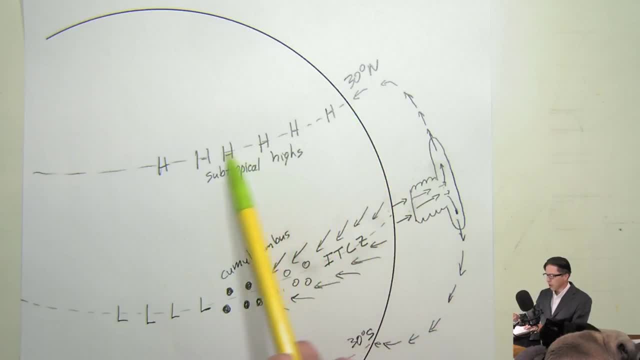 equator every day. we'd have a perfect band of high pressure right around 30 degrees every day. but what actually happens is you've got continents, and the continents heat up quicker during the day than the oceans and that tends to send air up and that tends to fight off, say, this high pressure. so what really? 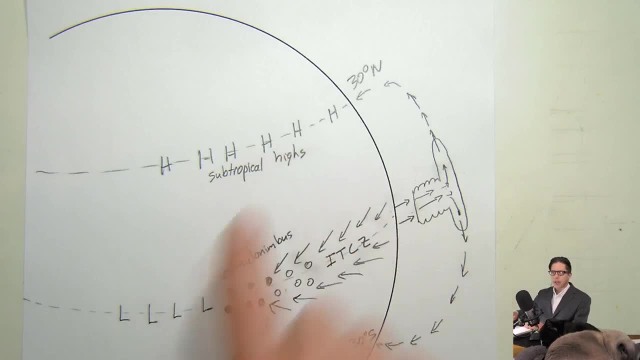 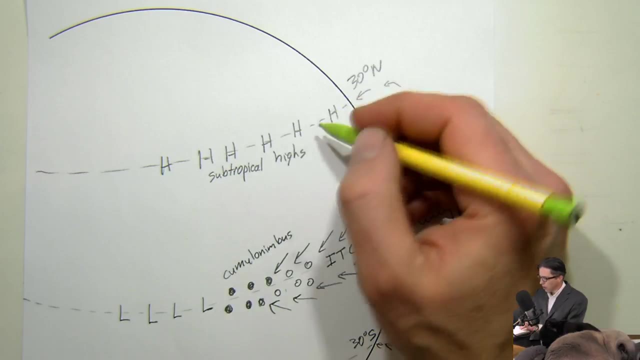 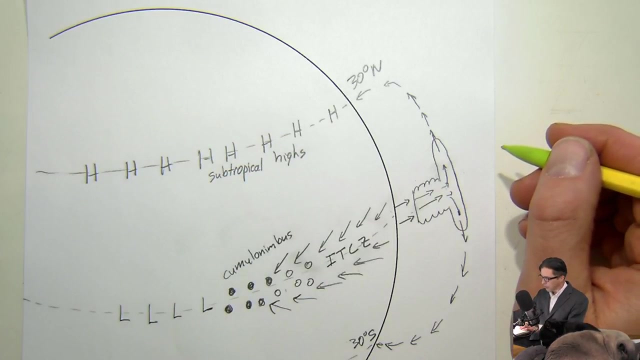 happens is this height that i'm drawing as a band. it kind of breaks up into certain zones over the ocean and i'll show that in a minute, but just for now let's just kind of continue this. we, this band of high pressures, is expected around 30 degrees north and 30 degrees south. so this loop that we 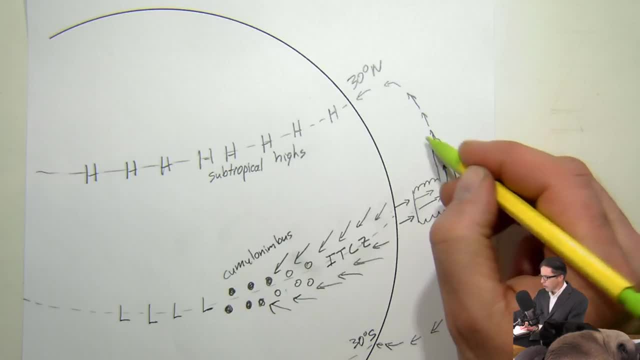 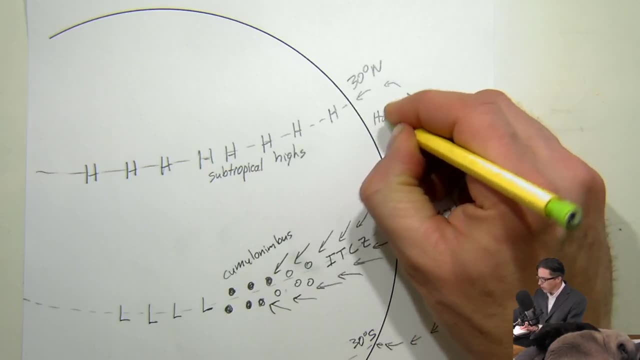 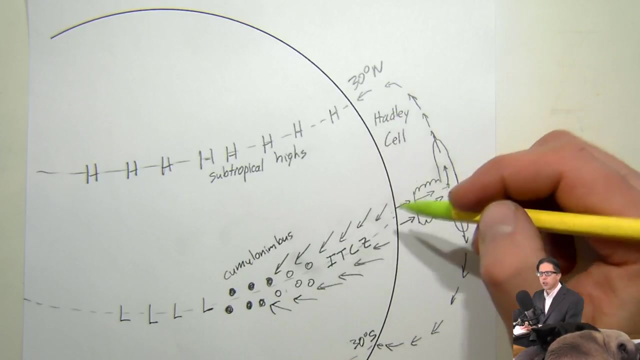 have where air rises at the equator and it goes 30 degrees north and it comes back down. now this loop is called the hadley cell. okay, the hadley cell, and this is one of the general circulation patterns in the earth. that air generally rises from the equator, sinks back. 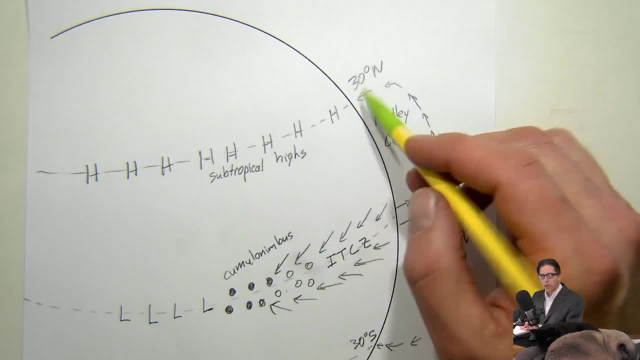 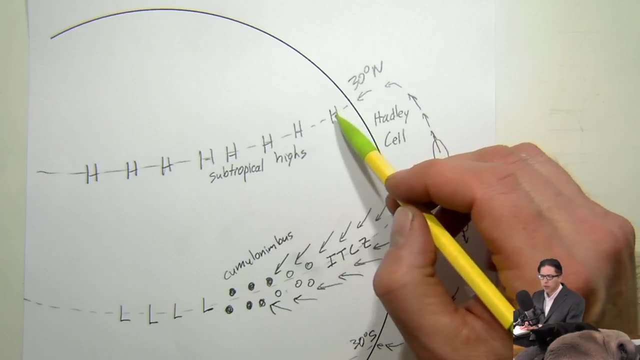 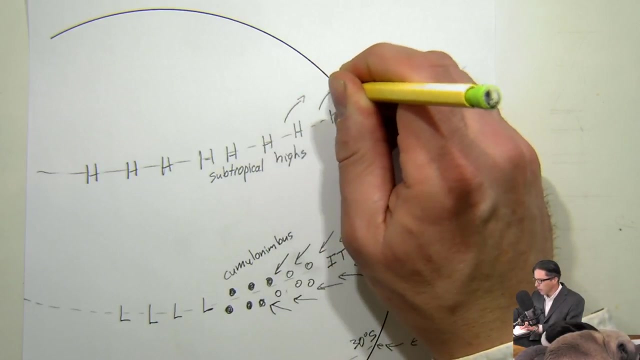 down at 30 degrees north and 30 degrees south. okay, so when air is sinking makes a high pressure. what direction does the wind blow around? a high in the northern hemisphere goes clockwise right. so you can imagine that if i had one single high i would draw a clockwise. 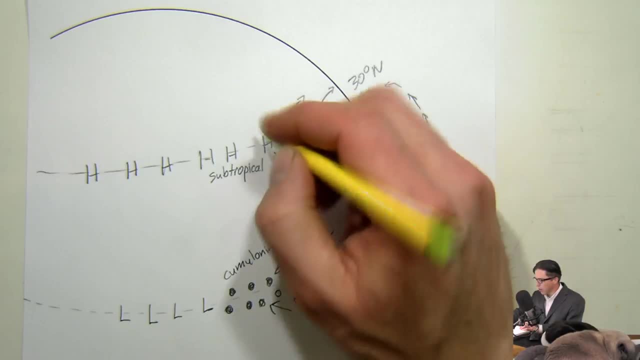 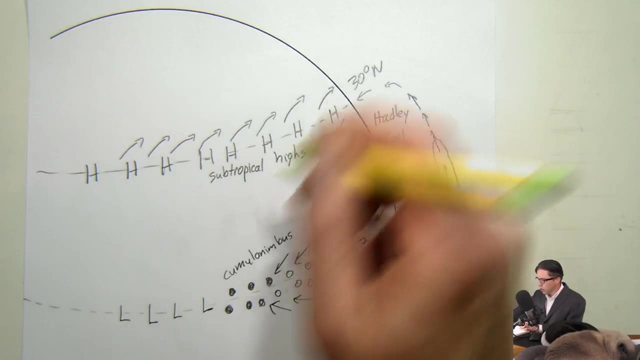 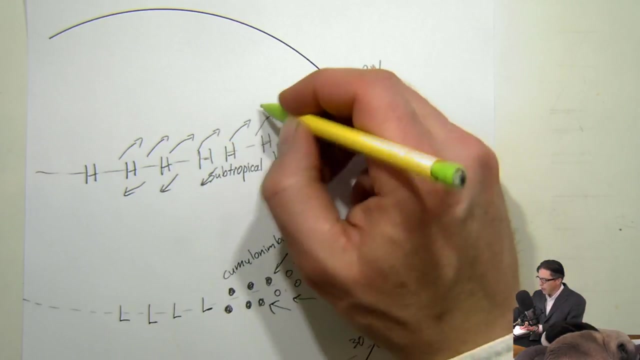 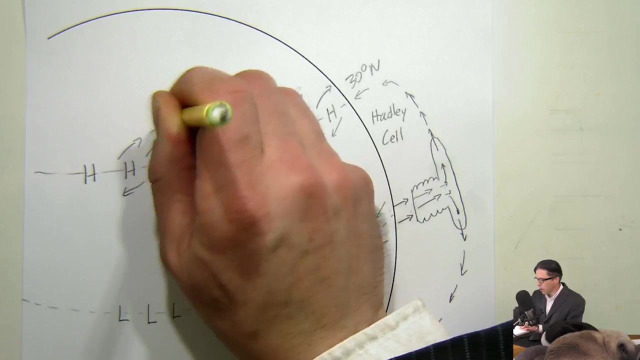 spiral around it, but i have a band of them, so you have to kind of imagine a whole bunch of clockwise spirals like this, and these spirals that i'm drawing to the north of the h combine to form what we winds that are coming primarily from the west called the westerlies. 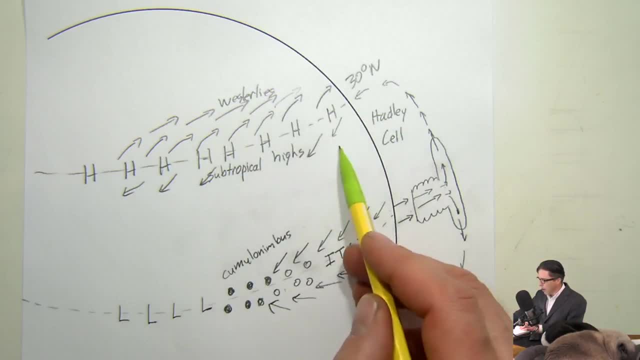 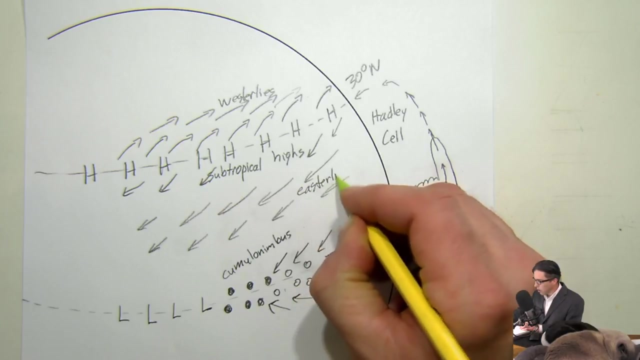 and these are combining to to um, these are combining uh to to provide what we call the easterlies. all right, so we've talked about that's. where we started was with the easterlies. now we can see that the easterlies down here are part of a big loop that formed when the air rose goes to 30. 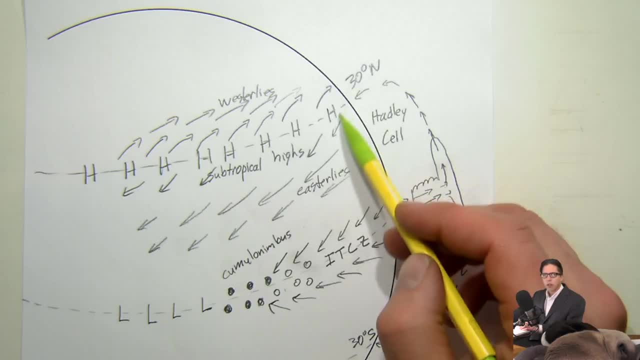 degrees north, 30 degrees south, sinks down in the northern hemisphere, makes high pressure, clockwise rotation around the highs and and the clockwise rotation south of each one of these h's combines to produce a band of wind that we call the easterlies and, to the north, a band of wind that we call the. 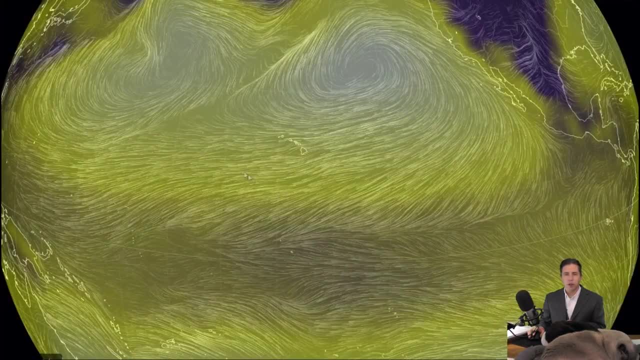 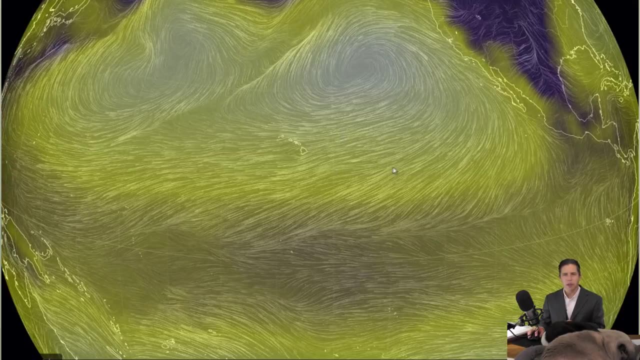 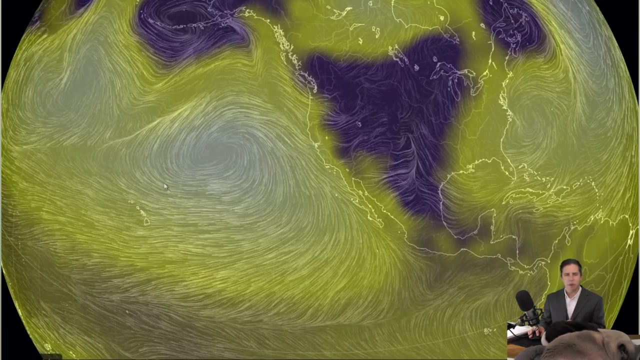 the easterlies, we're going to return to our map of air pressure here. so, where we left off, we were talking about this thermal low around the equator. Now to orient yourself, so there's the United States, there's Hawaii. Notice what's this big spiral out in the ocean here? 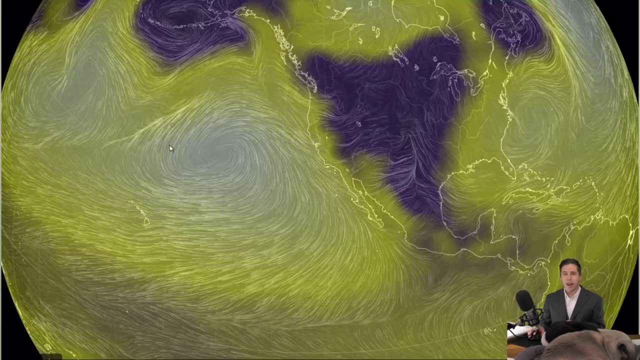 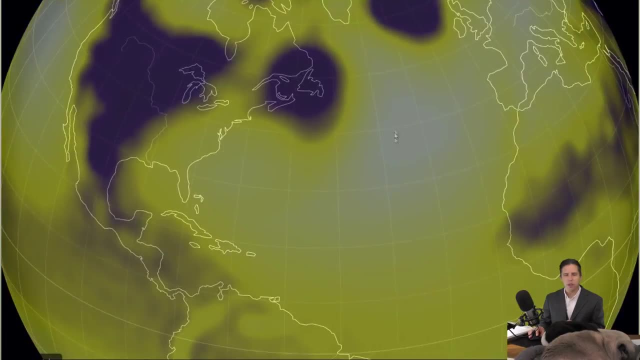 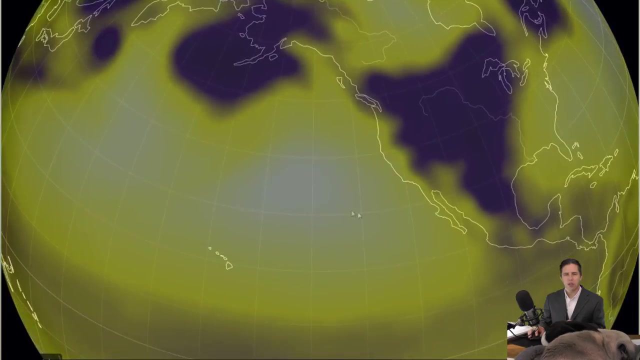 And another one, so clockwise rotation. that's consistent with a high pressure. Here's another one high pressure. Here's another one. right around the same latitude: high pressure, A little one there, Okay, so what we're seeing is we're seeing high pressure, blobs of high pressure. 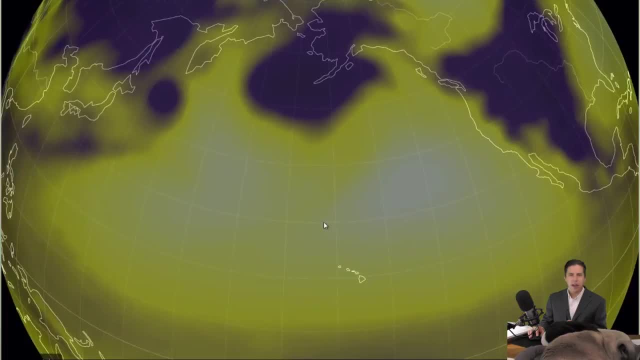 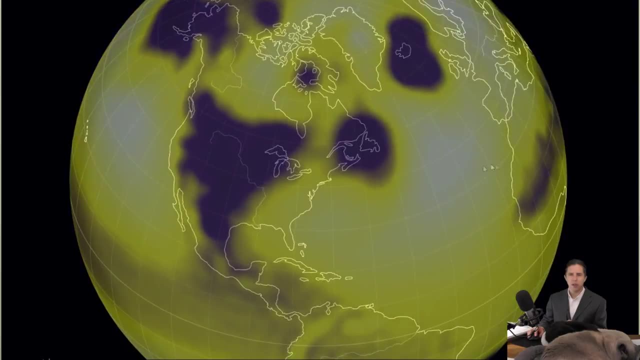 These are the subtropical highs And, again, if the Earth was all water, we would see a band of them all the way across. But what actually happens is they tend to kind of form more over the ocean basins And we see a little bit here in Europe. 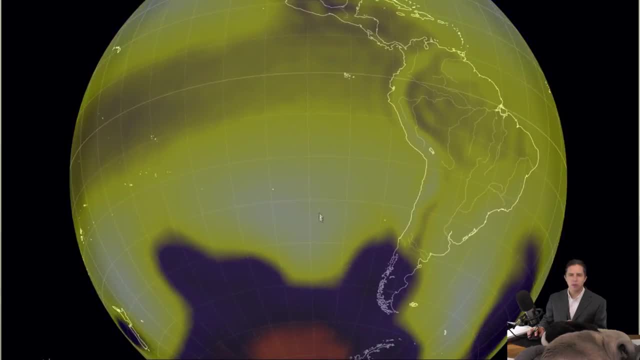 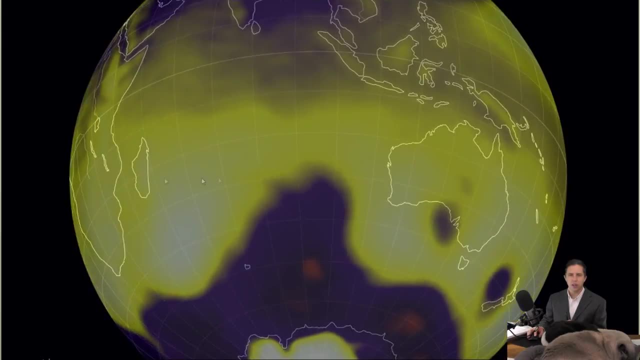 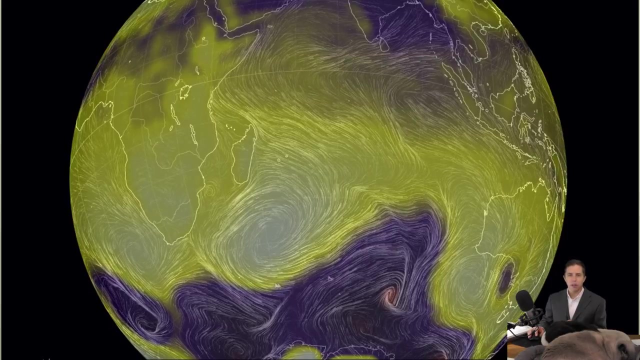 Let me go to the southern hemisphere. Okay, there's a bunch of them in the southern hemisphere. That white blob, that white blob. you know they're spinning in the opposite direction Because of the Coriolis effect down there, But you've got these blobs of sinking air that are, in this case, spinning counterclockwise. 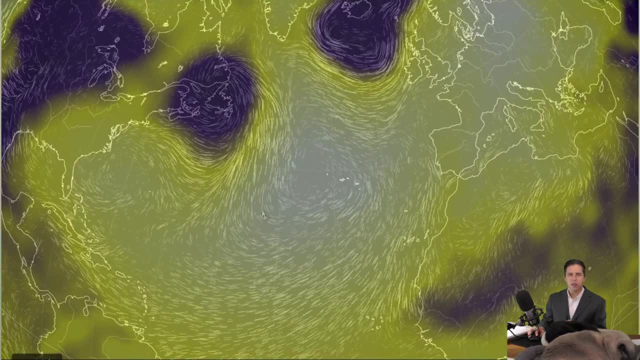 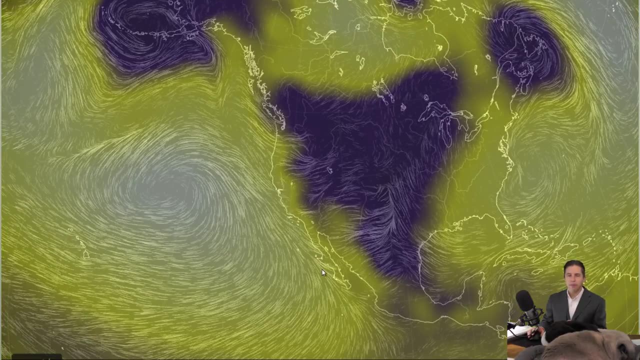 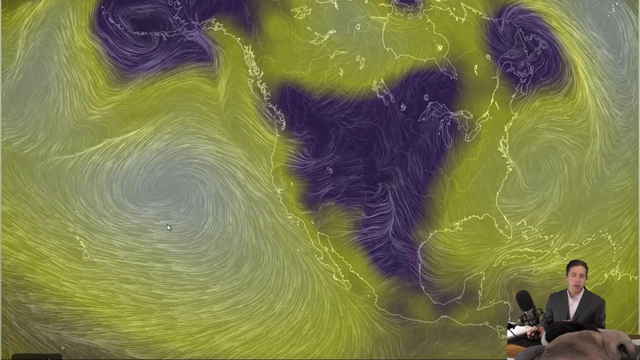 And are the neck of the wood spinning clockwise. These are these subtropical highs. Now, subtropical highs tend to, so they tend to form over the ocean basins And they kind of tend to be found kind of in the same place day to day. 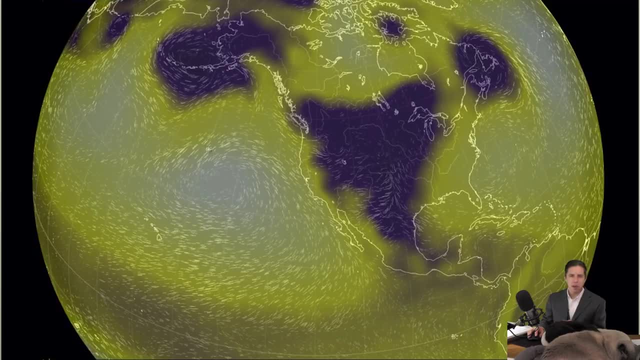 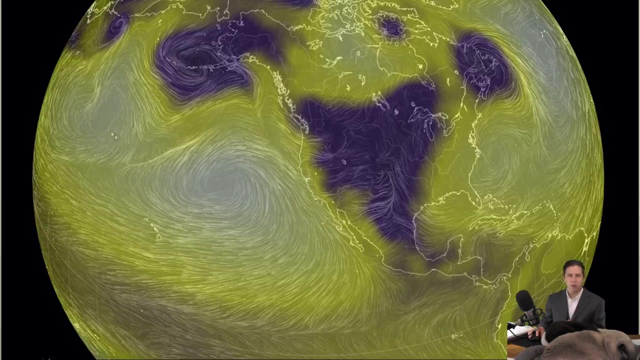 So if we did this tomorrow, we would notice that that big high-pressure blob right there is still there And day to day it moves around a little bit. It might join forces with that one. Then they split apart. This one also kind of moves around day to day. 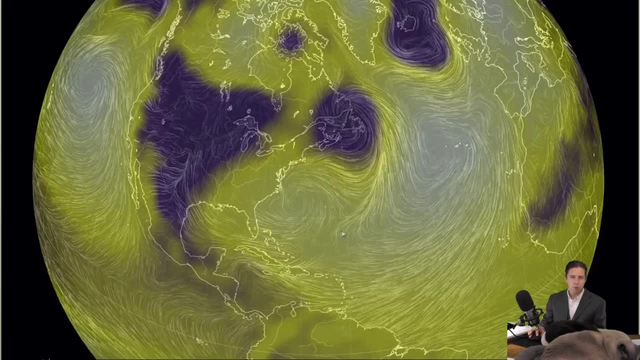 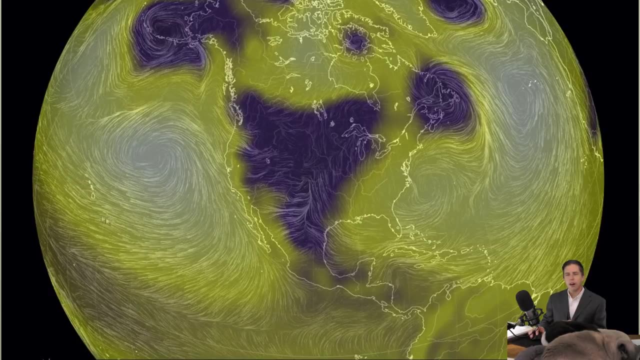 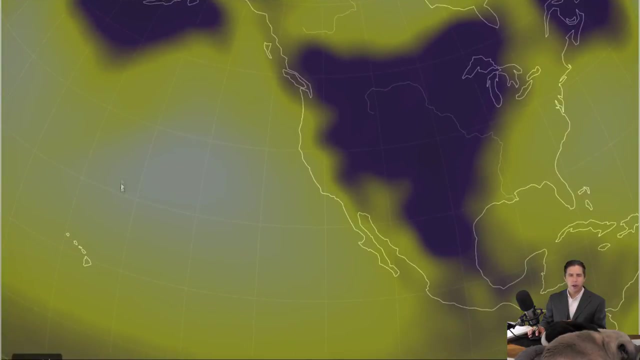 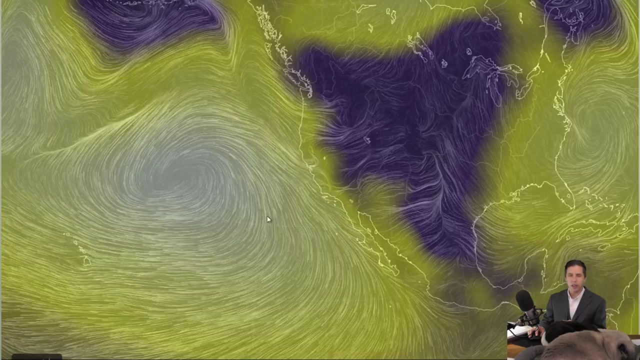 If we compared winter versus summer, we would see that they move quite a bit more in the seasons. But these subtropical highs are very consistent, And so we give them names. This one right out here is called the Pacific subtropical high, So this is the one that's parked right off the West Coast of the United States. 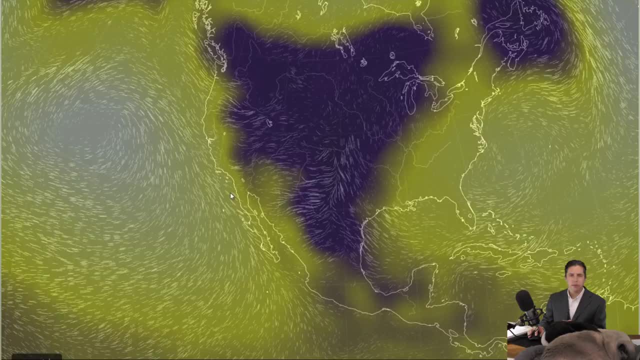 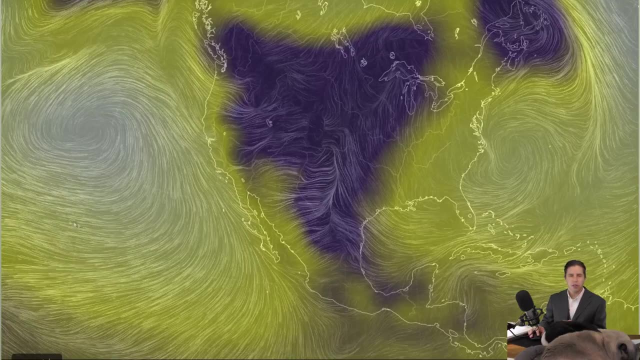 And you'll notice that. So right along the coast, it's actually under the influence of these winds from this big spinning subtropical high. So the presence of this high right out here It's actually under the influence of these winds from this big spinning subtropical high. 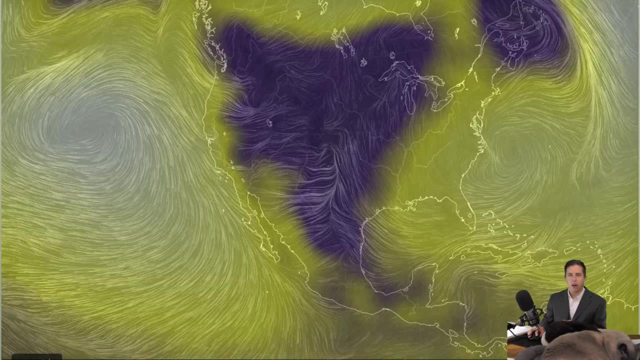 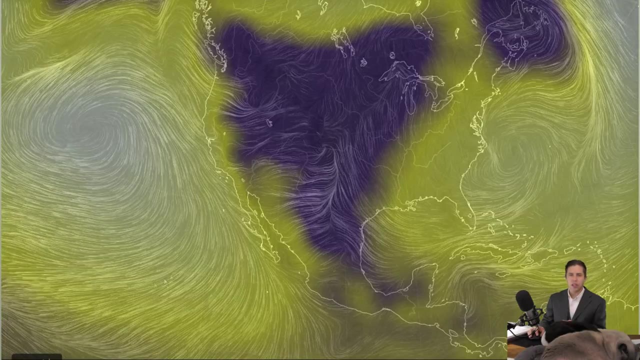 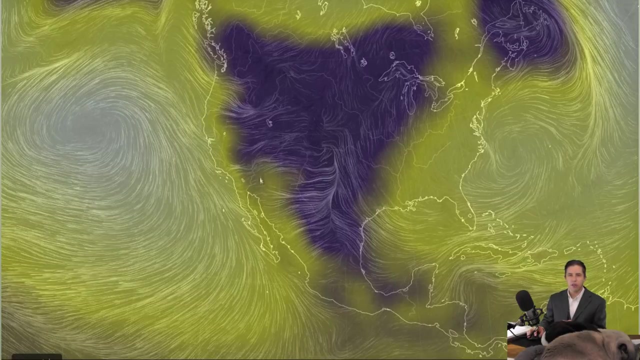 off the coast really affects the weather on the west coast and in fact it includes- that includes- new mexico. this is a big blob of sinking air. if you have a big blob of sinking air sitting right out here over the ocean and it kind of bleeds over to the continent, that means that the west coast 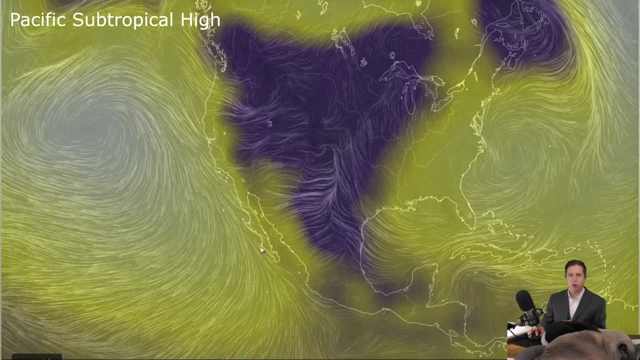 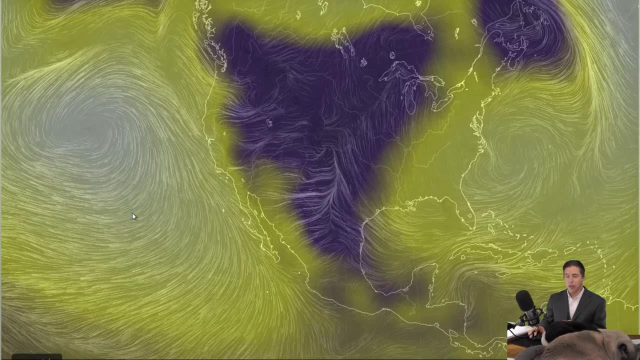 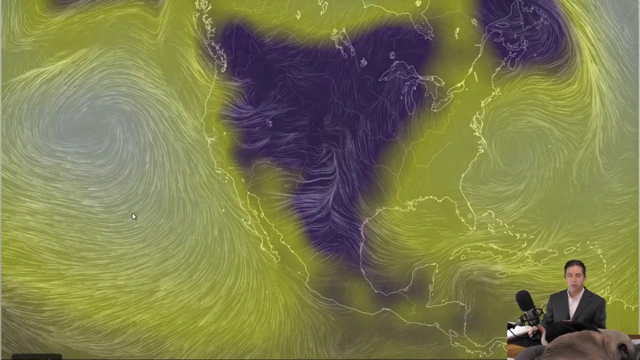 and baja, california and arizona and new mexico are all at times under the influence of this big blob of sinking air, which means if you have sinking air, high pressure that fights cloud formation that tends to make deserts right. so if you think about the climate of what it's like, 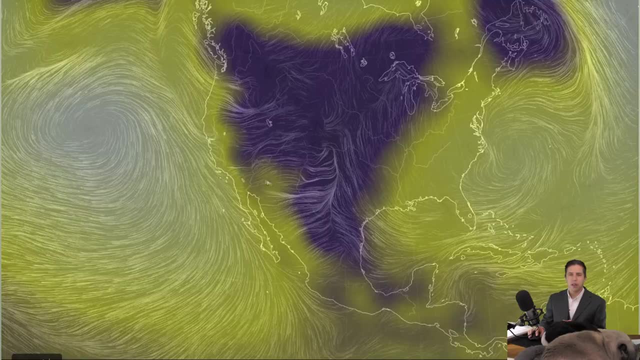 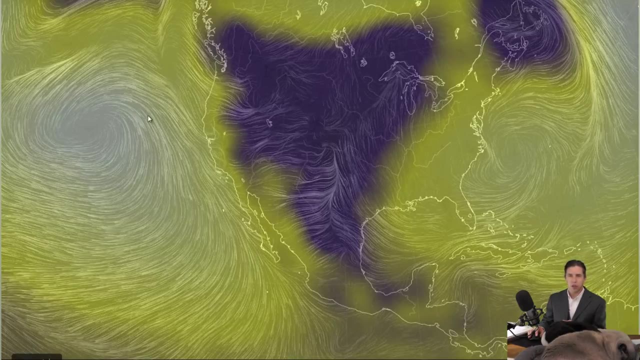 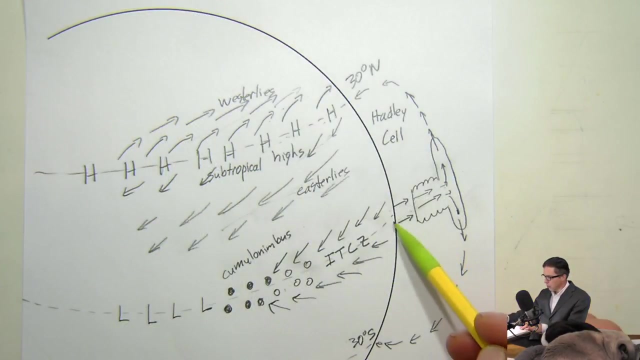 over in here in the mojave desert and the chihuahuan desert, arizona, new mexico. why is it all so dry out here? well, it's due to this pacific subtropical high. so think about the big picture here. air has risen from the equator, makes cumulonimbus you can think of as like squeezing all the water. 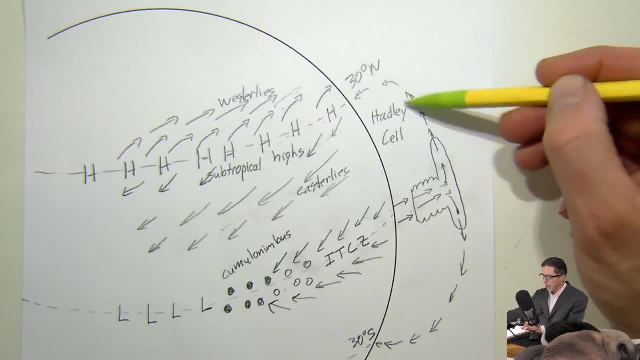 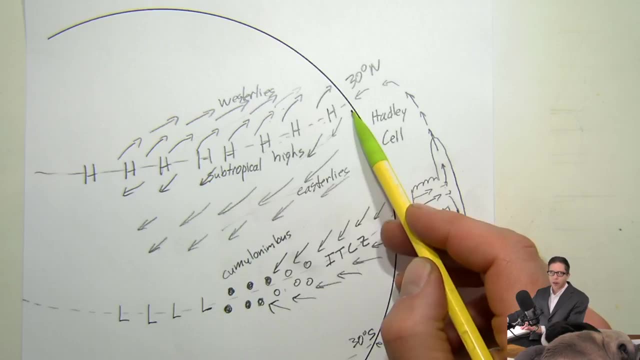 out from the cumulonimbus, so it's dry air. then it goes north, then it sinks, sinking air warms. so now you've got air that's fairly warm and really dry and it then hits the ground and produces high pressure. so so if you live under here anywhere, 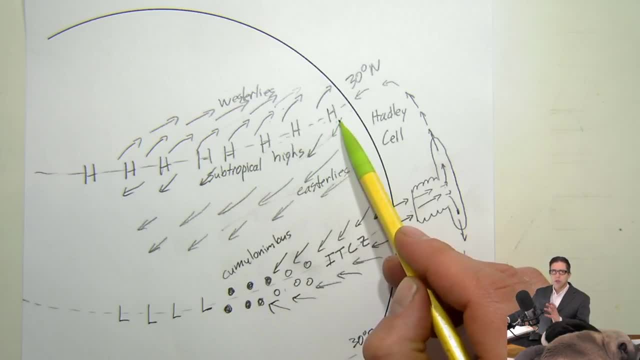 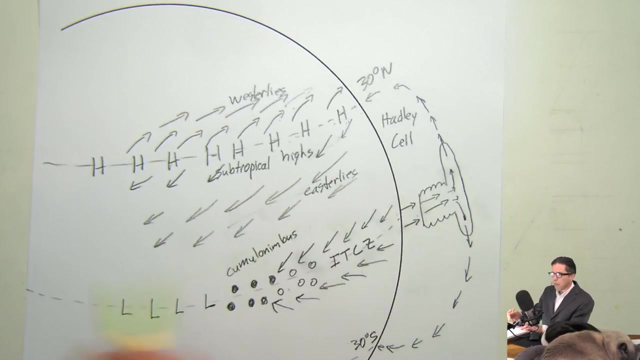 under one of these subtropical highs, you'd expect to live in a zone that's very, very dry, okay, and new mexico is one of those places. new mexico, arizona, southern california- we're all under the pacific subtropical high. so i'm going to add on this with my band of h's. is that i'm going to? 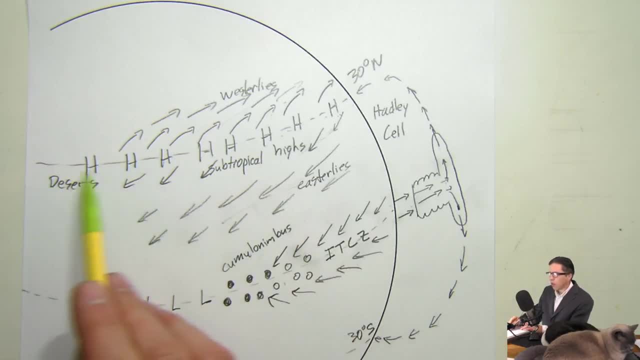 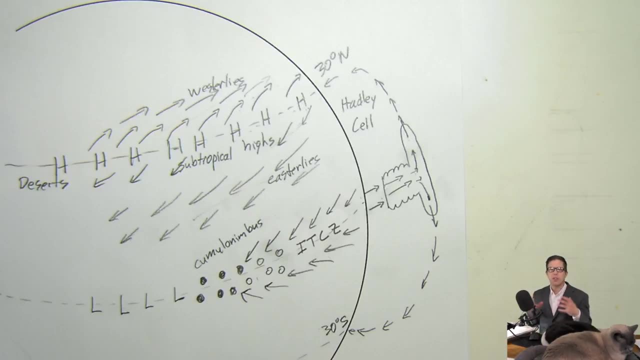 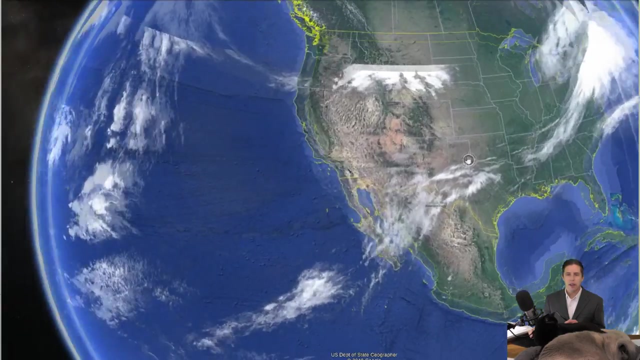 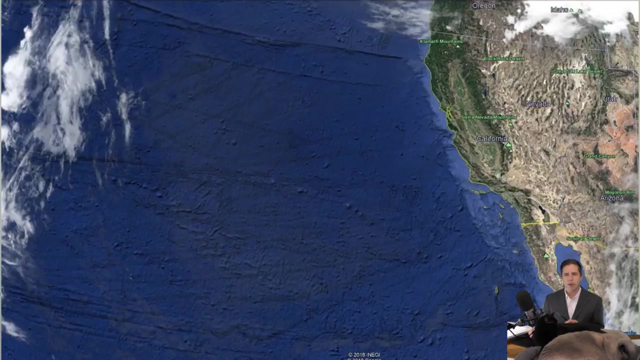 put down deserts. okay, all all along this band, around 30 degrees or so, you'd expect to find deserts because of this. so we can look at the subtropical highs a different way. and i am now back in google earth looking at clouds again and what i notice. so there's california right there. i noticed that. 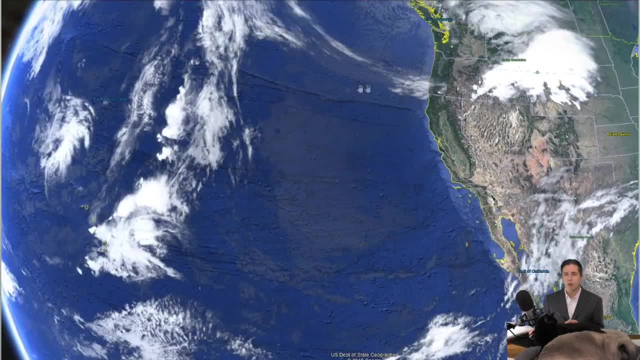 there's this big area out here in the ocean where there's no clouds. now, remember, these are infrared images, so they only show tall clouds. so there could be fog or stratocumulus, something like that, but no tall clouds. so i'm going to put down deserts and i'm going to put down. 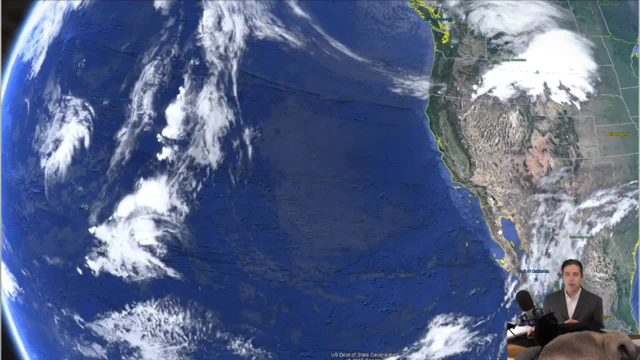 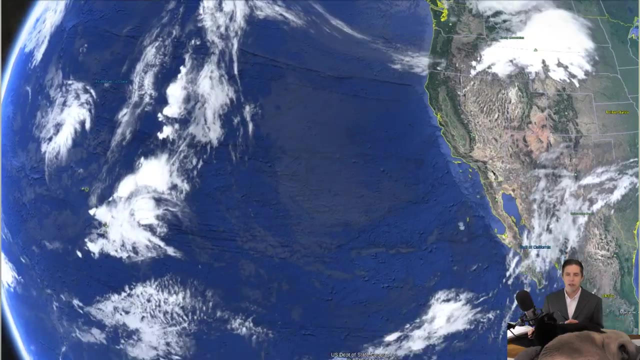 clouds out here. why is that? that's the pacific subtropical high. this whole thing is a giant clockwise spinning blob of high pressure sinking air fights cloud formation. so you see this big area in the ocean where there's no clouds, at least no tall clouds, or i could go to the southern. 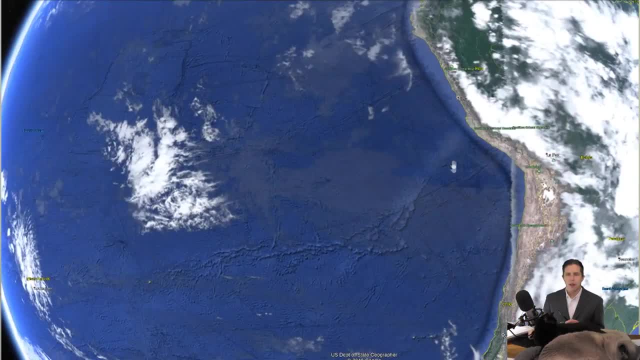 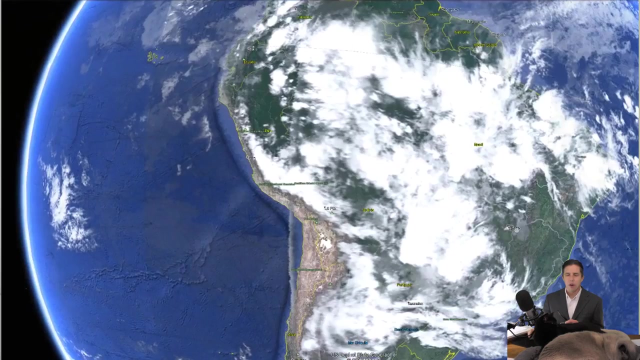 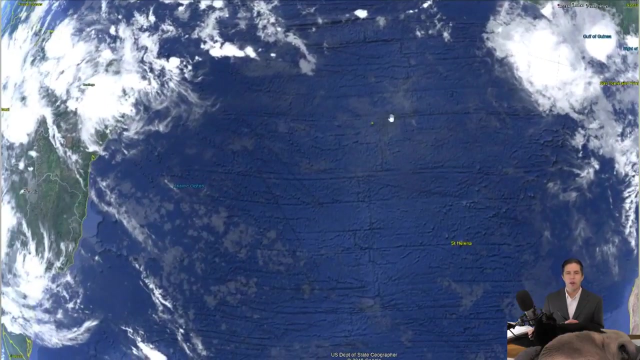 hemisphere and right down here it spins in the opposite direction b. it would be counterclockwise. but right here is another big blob of high pressure sinking air from the subtropical highs and again we see almost no clouds, no tall clouds, or we could go over here. so again roughly in the same area in latitude, big blob out here in the 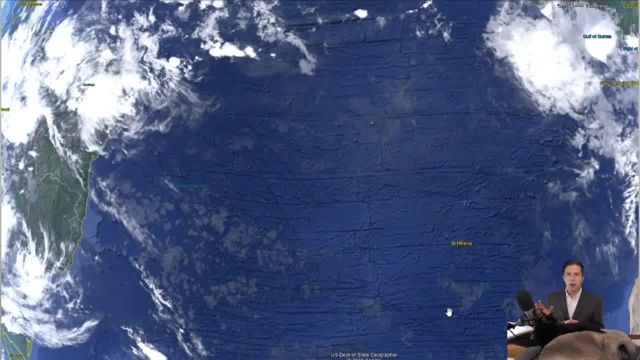 ocean, no clouds. so subtropical highs are areas of sinking air that, originated from the equator, produces high pressure and that, in turn, fights cloud formation. so we can see that there's no cloud formation and if you live under an area, one of these, under one of these subtropical highs, 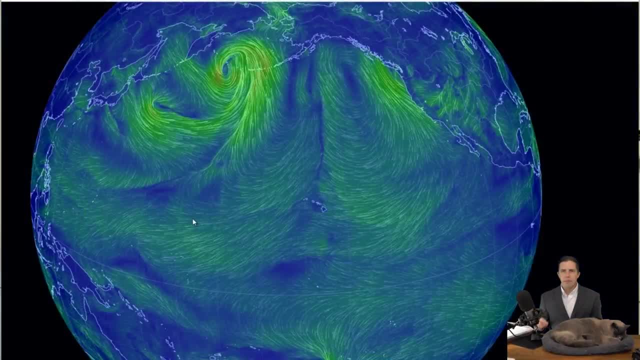 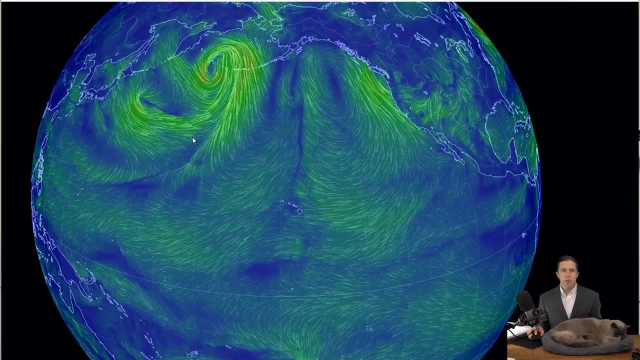 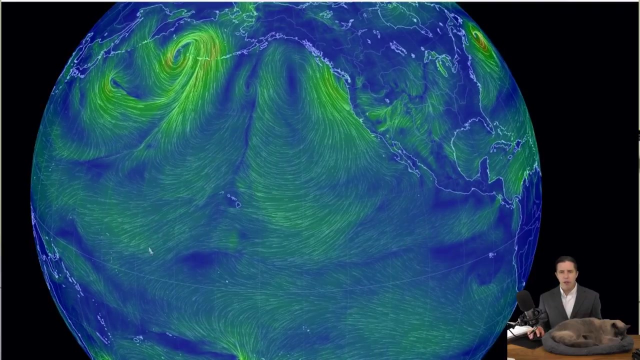 you're living in a desert almost every time, so let's look for some westerlies. now we're back looking at surface winds. the colors represent wind speed, and so here what i see are a whole bunch of easterlies that we saw previously, right through here and, according to the diagram, we've 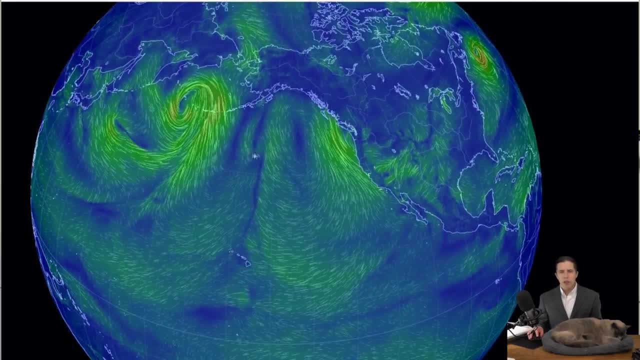 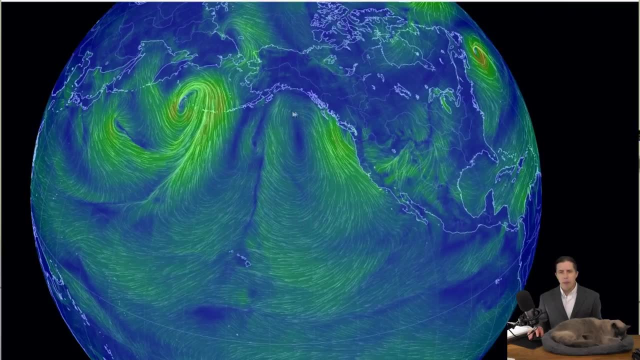 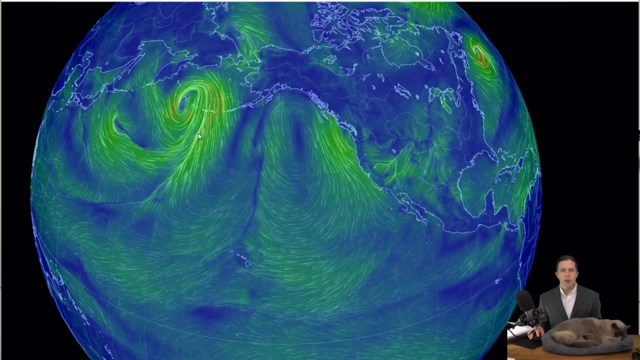 been drawing. we'd expect to find westerlies kind of right here and we're going to look at them right through here, but it doesn't. it's not really obvious. here i see this big clockwise spiral and that is the pacific subtropical high. i've got a couple counterclockwise spirals, those 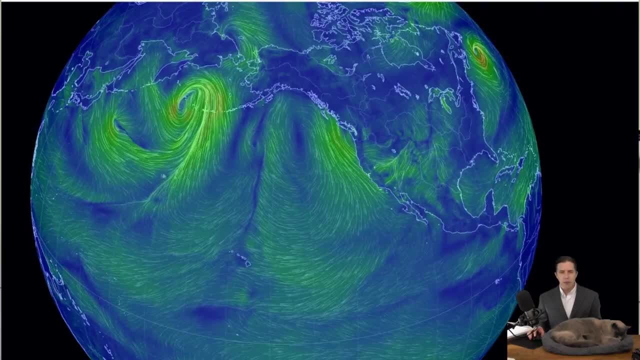 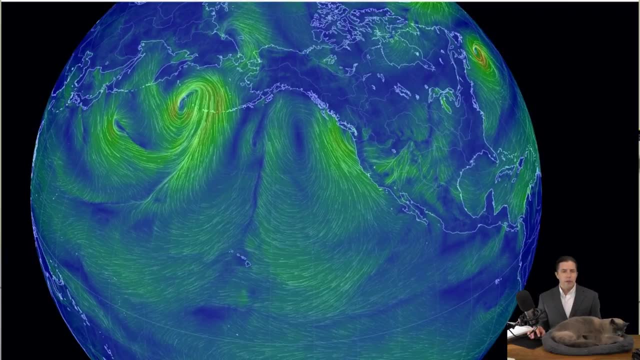 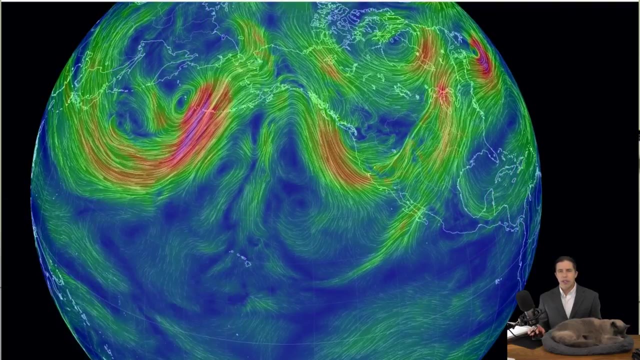 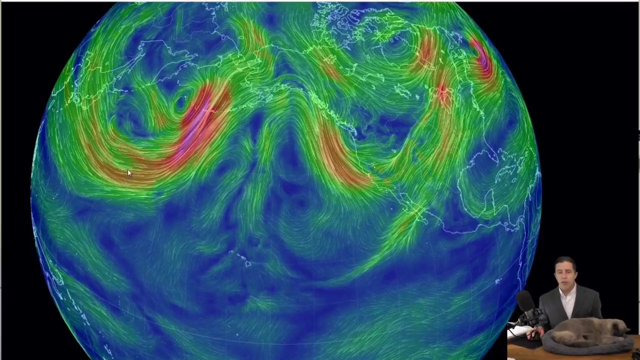 are a couple of mid-latitude cyclones, but nothing really looks like a wind traveling from west to east, like we just drew. so what i'm going to do is change the height, and i'm going to go to 700 millibars again is roughly somewhere around 10 to 12 000 feet above the surface, and notice how different. 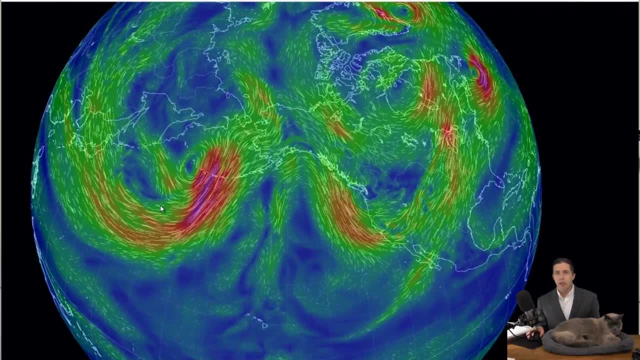 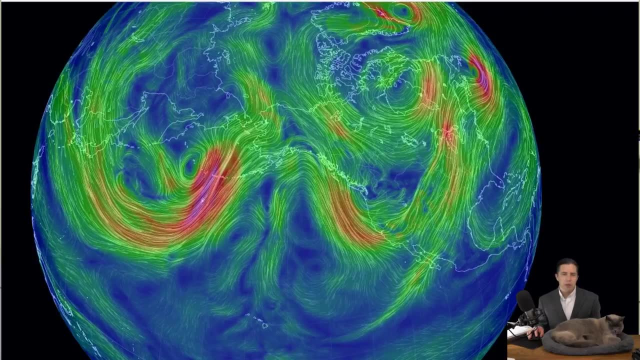 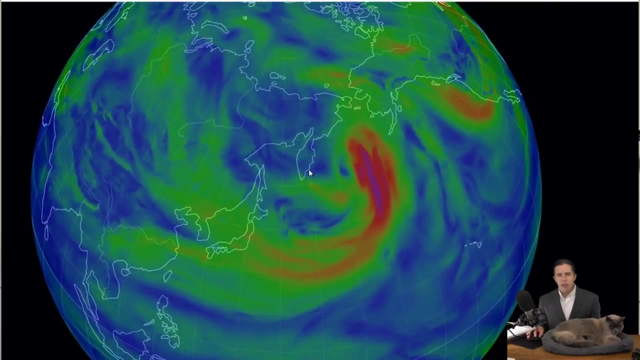 the winds look up there, so the colors again represent speed. so when you see this, those are some really high speed winds. i don't know how high, but i would not be surprised if some of these in here were 100 miles an hour or something like that. so what we see is look around the earth. here we 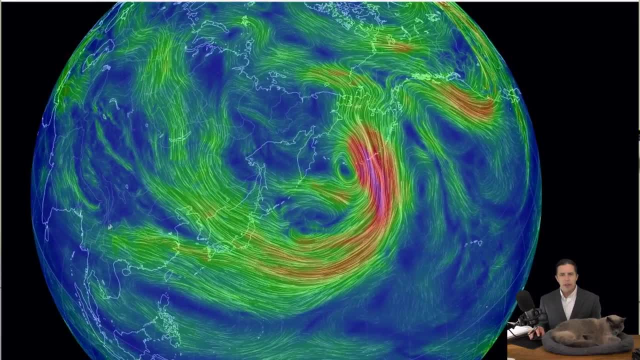 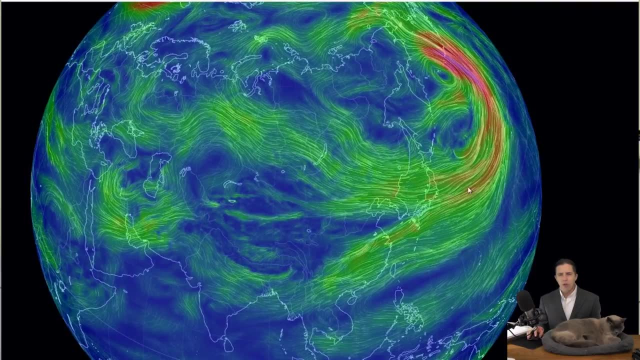 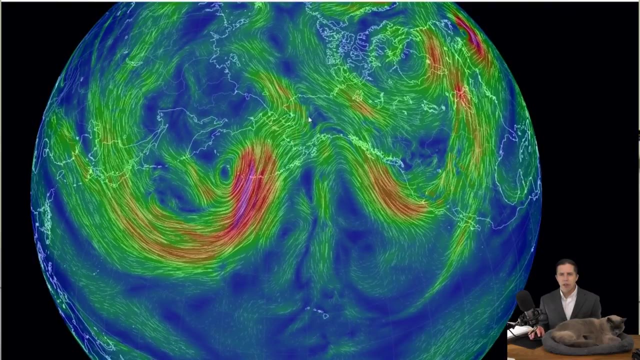 can see that we've got these ribbons of wind that are kind of intermittent right. so over here, over asia, you don't see them, and then they start over the uh as we go over the pacific, and this one goes north, kind of up into alaska, and then back down and 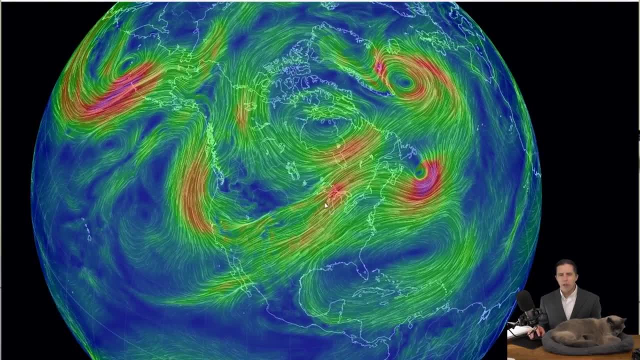 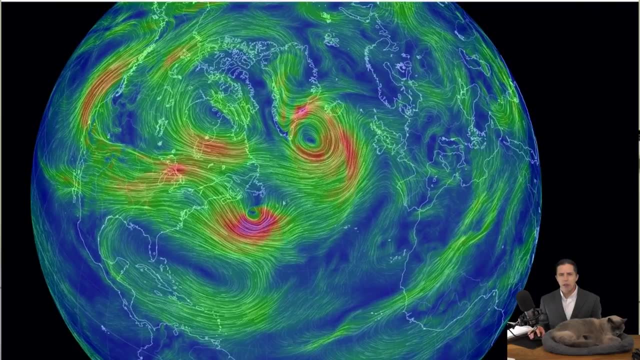 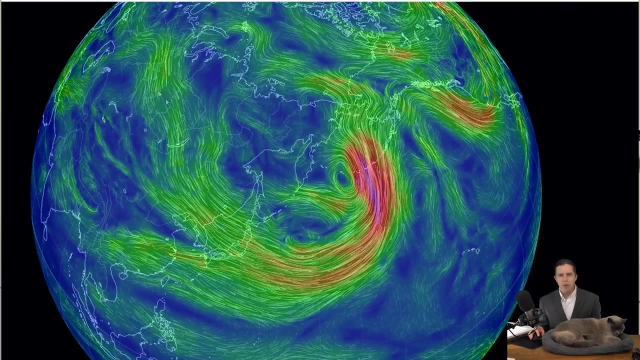 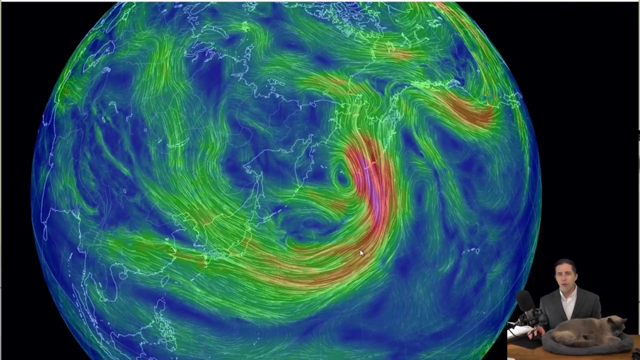 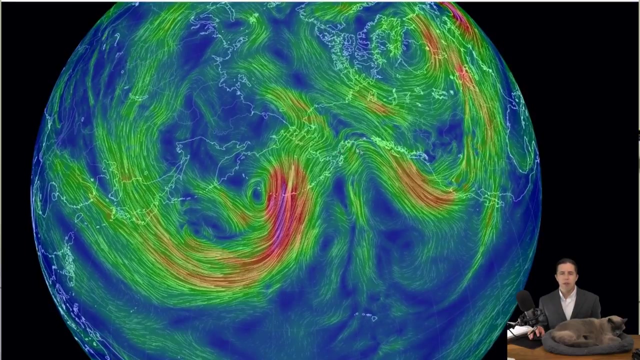 then fades away a little bit, comes back across, uh, north america, and then there's a bunch of little edges, but it'll go through. um, the sarah falls right west of austin, um deep into ciego. so then the how it gets strap to tyrol. 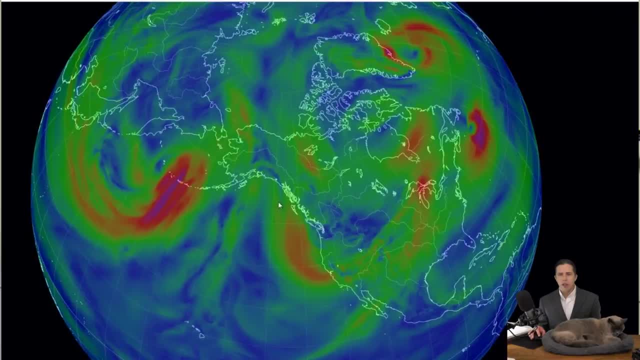 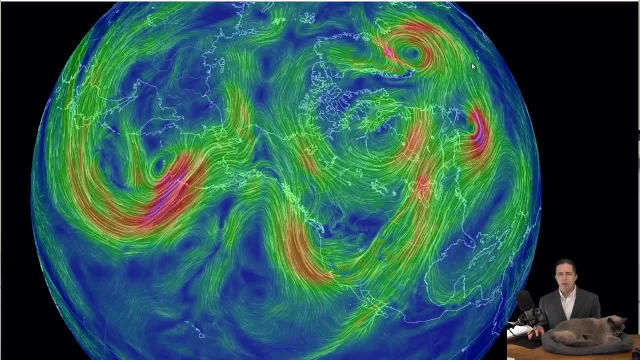 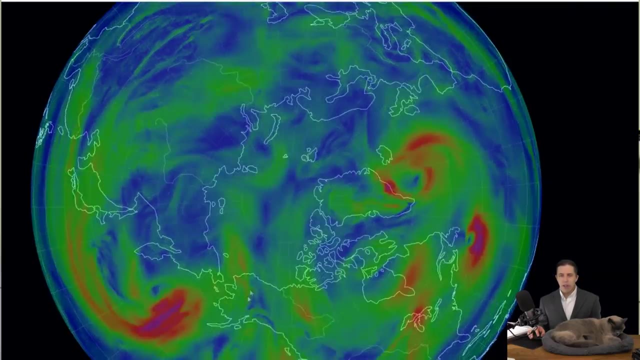 because tightly leaders this river to musa lots 3 years. how there's no, it's always time way all the way around the world back roughly where you started. these are the westerlies. okay, so it looks quite different than what we drew, and every day you look it's it's different. so if i 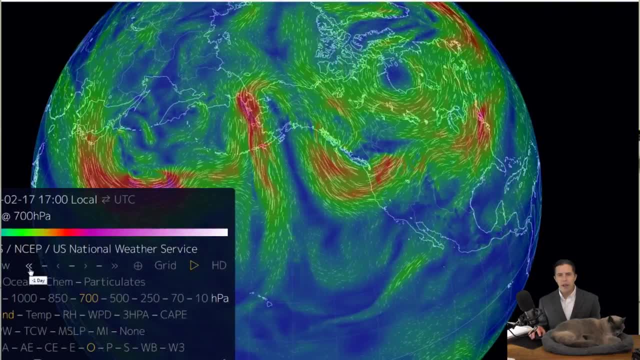 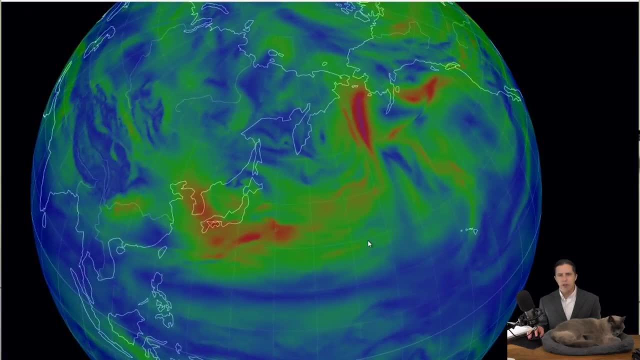 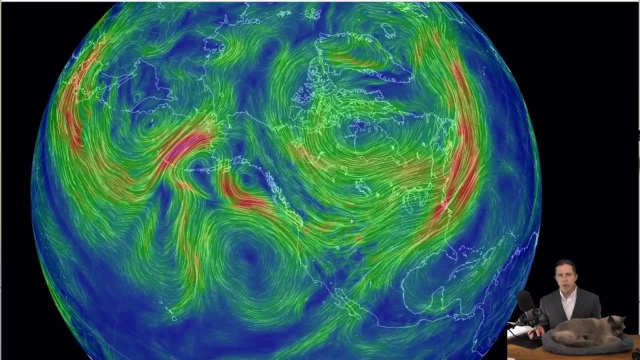 let's just go back a couple days here, so go back a day, back another day, okay, so just i'll stop right there. so now you can see how different it looks here. so there's our stream coming off of asia, and now, right, we have a much thicker band across north america. it's really sped up coming. 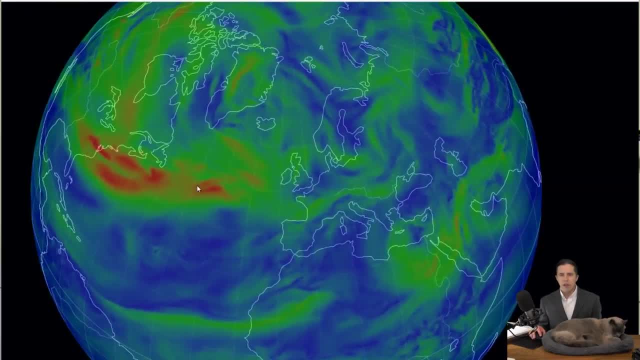 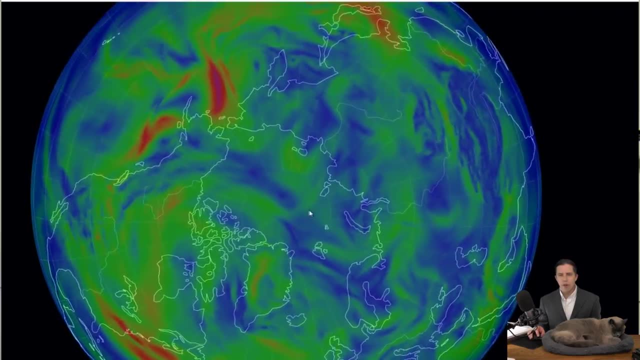 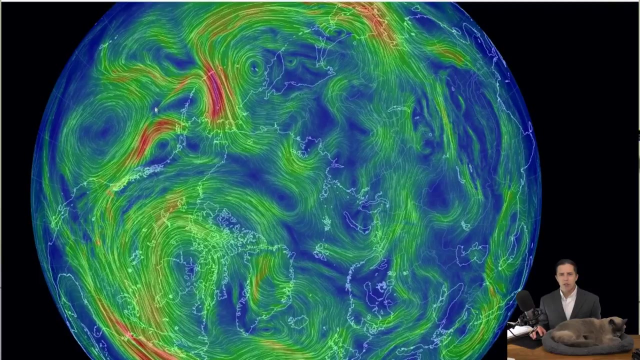 off, uh, north america over the atlantic. you can follow these streams over into europe, okay. so every day it's a little bit different, but if i kind of tilt the earth and look down the north pole in general, what i would see from the north pole is this counterclockwise circulation: you. 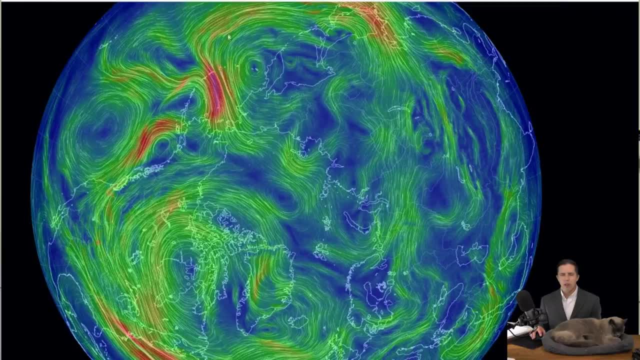 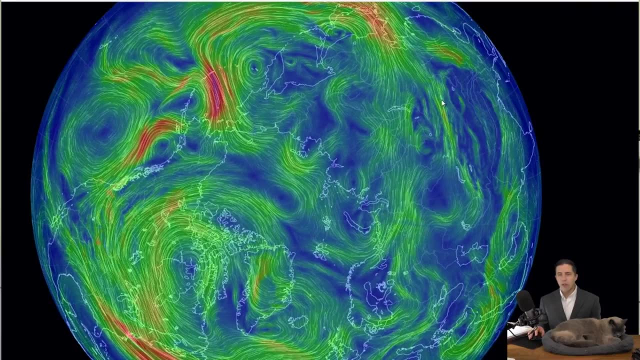 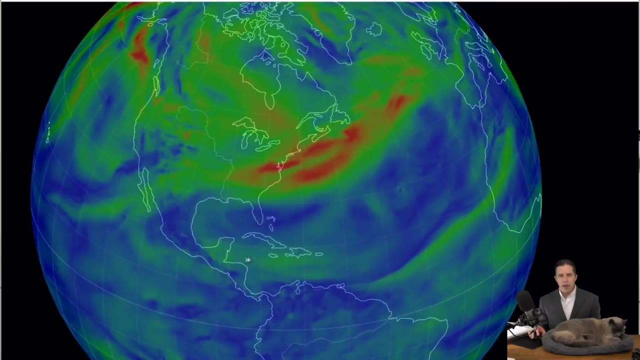 know there's exceptions to this, but again, if i drop you off in a balloon, you go around and around, but eventually you would make your way all the way around the world and through these, following these different ribbons of air, and these are what we call the westerlies. now i'm going to go even a little higher, up to 500 millibars. so now, this is. 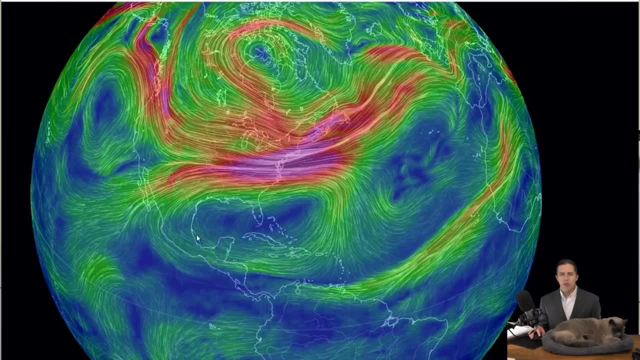 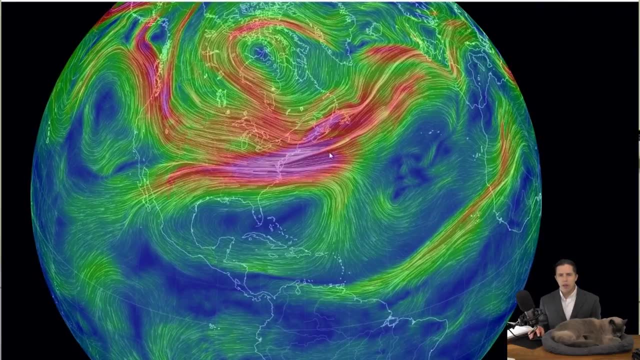 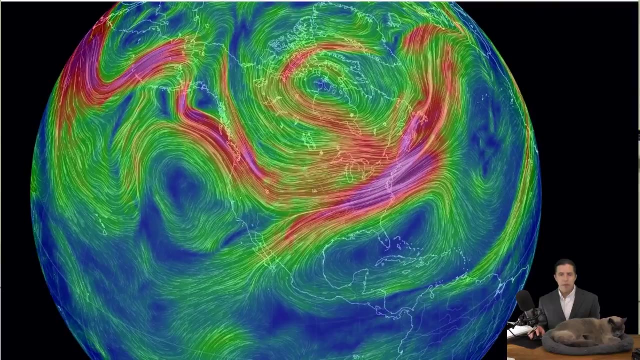 roughly how high commercial jets fly, and so one of the things that you see is that the winds are now much faster, and so you can see this: this ribbon right here, that's really fast. this ribbon right here, that's very fast. if you've heard the term jet stream, these are jets, okay. so these are these ribbons of high speed. 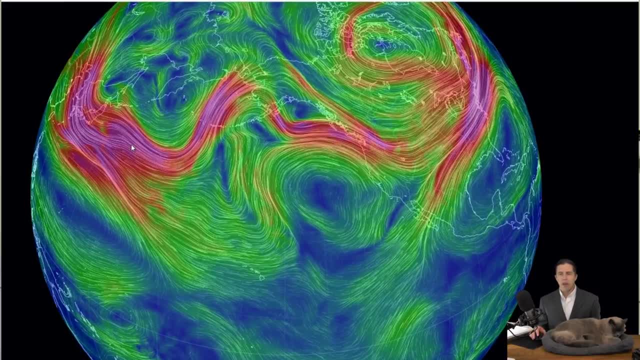 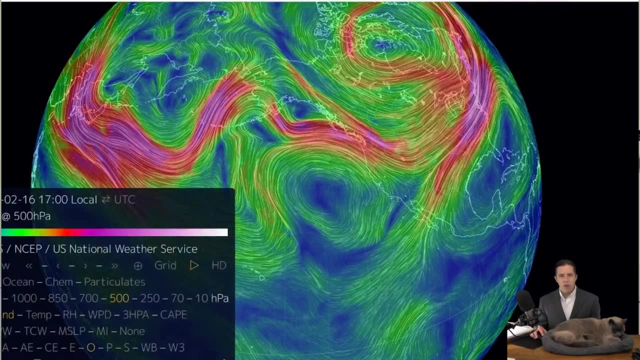 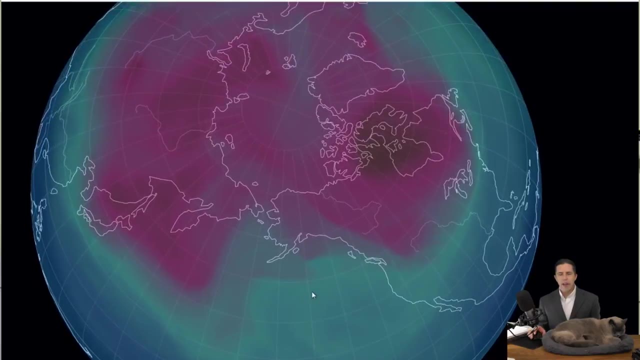 moving wind that are in the westerlies and when forecasters talk about the jet stream, this is what they're talking about now, if i go and change the overlay to temperature. okay, so now the colors represent temperature and if you think back, a lecture we talked about how there's this pool of cold air up here making 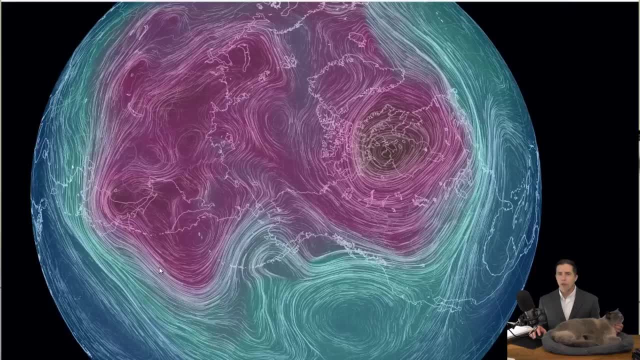 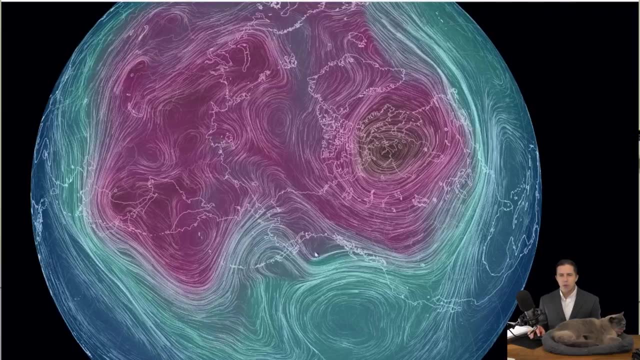 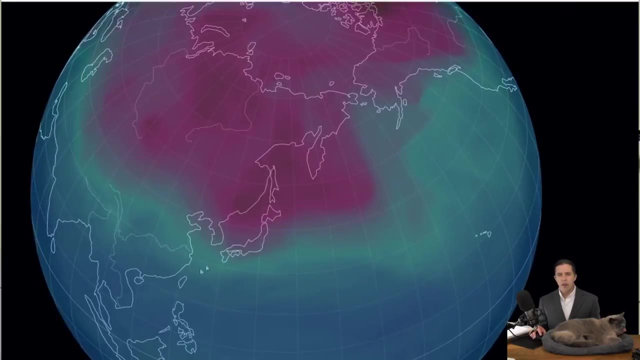 these rosby waves, and we talked about the polar front, and the polar front was this division between the warmer air and the cooler air. well, this high speed wind, this ribbon of westerlies that we're talking about, kind of follows the rosby waves. so, in other words, if i look over here, 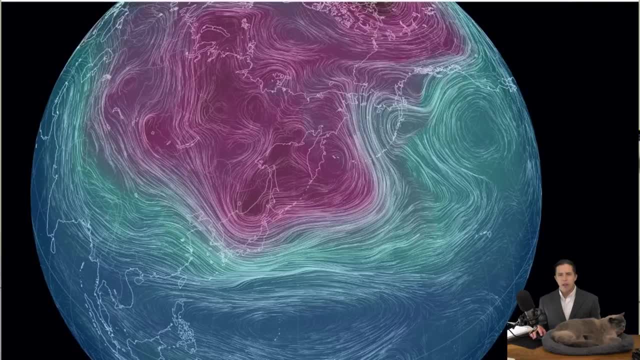 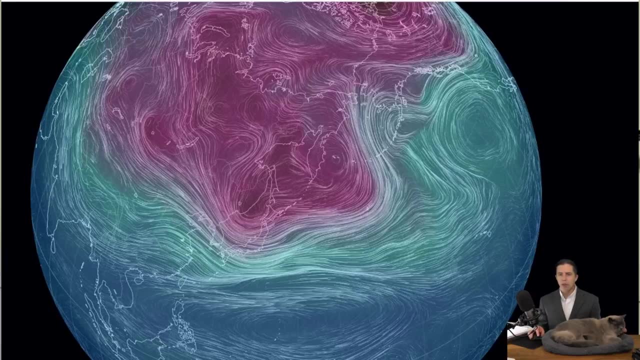 where that one of those jet streams were. right through there it's forming kind of right on the boundary between the warmer air and the colder air. it's forming right along that polar front. so if you, if you um, are watching, say, at weather forecasts and they're talking about the jet stream. 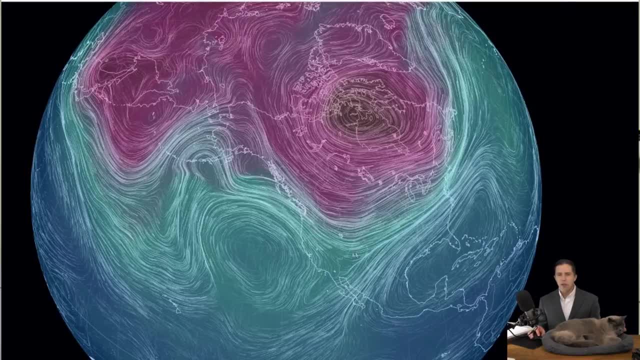 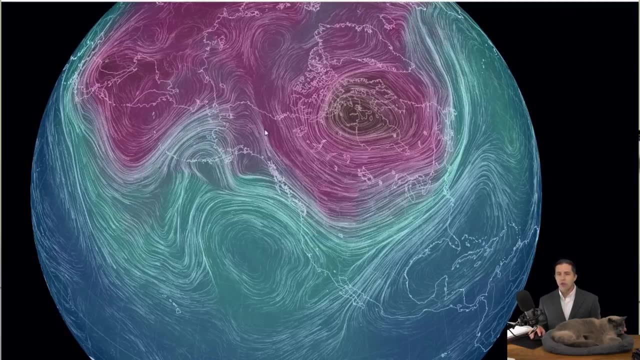 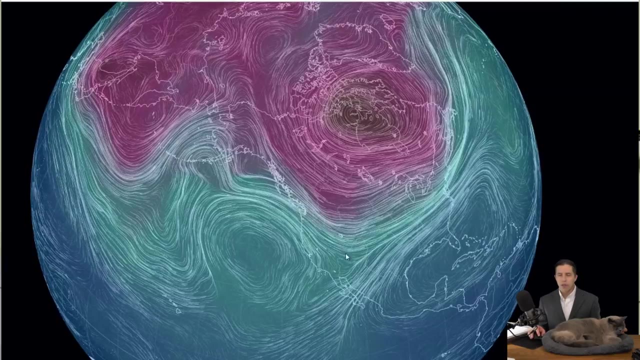 and they say: well, that jet stream, it's coming down into new mexico, okay, well, the reason that's important is because the jet stream typically follows the polar front. so if the jet stream comes down over new mexico, that means this blob of cold air is also dipping down over new mexico at. 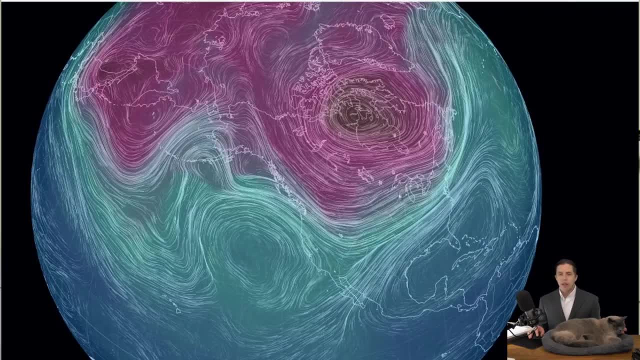 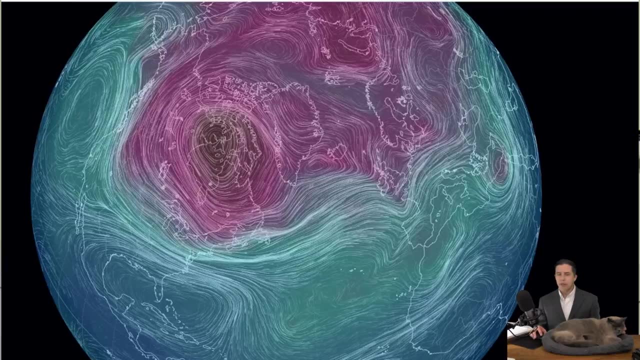 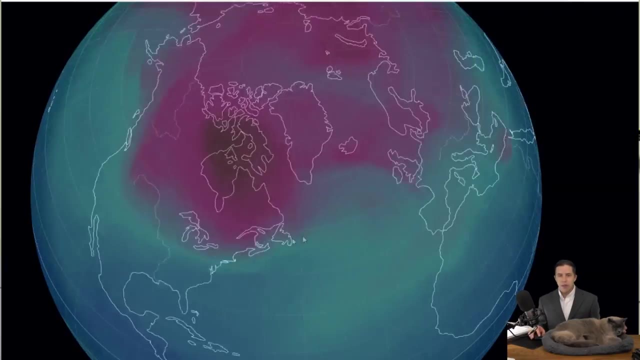 the same time, at least the border of it is. so they'll talk about the jet stream um, from time to time in weather forecasts, mid latitude cyclones typically form along that border, like we talked about last time. so those are the westerlies. now it's also. let's go back to go back to surface. 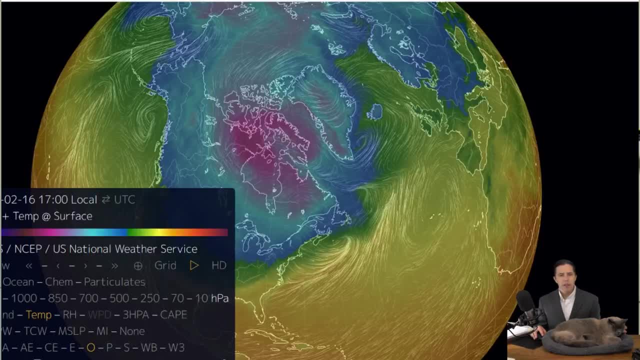 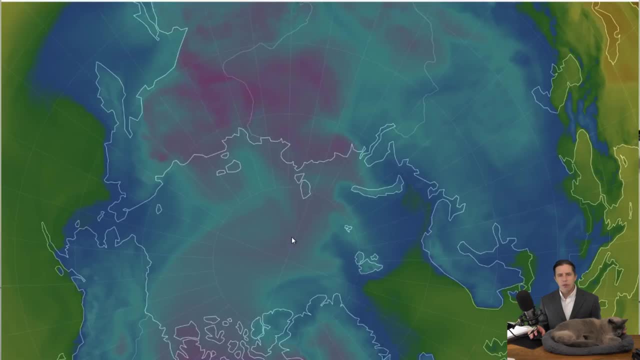 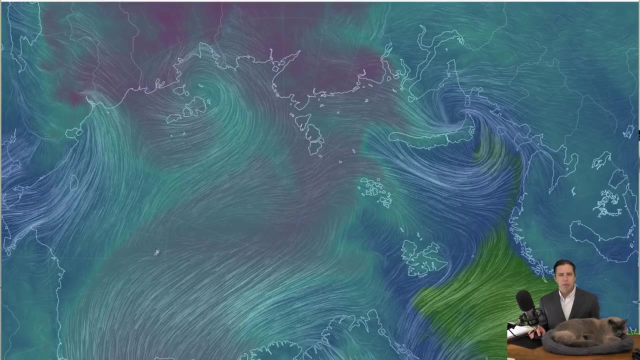 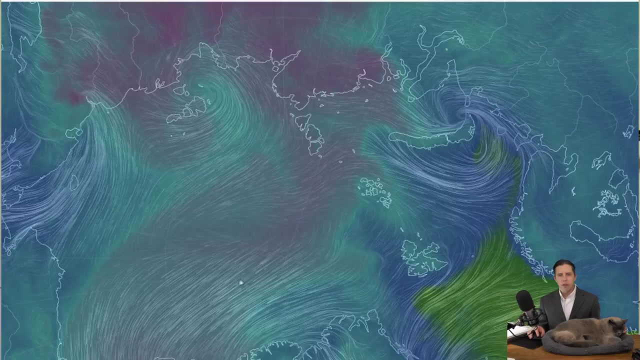 and let's see- let's leave it on temperature for a bit- we're looking straight down the north pole. i'm going to zoom in here. okay, it's not very well developed today, but right here i think you can kind of make out. there's a clockwise spiral here, and usually over the north pole there is a high pressure. 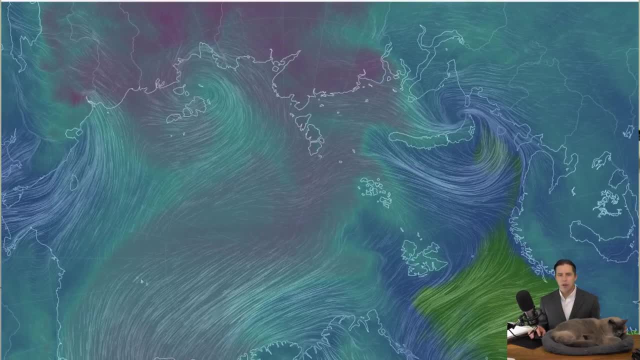 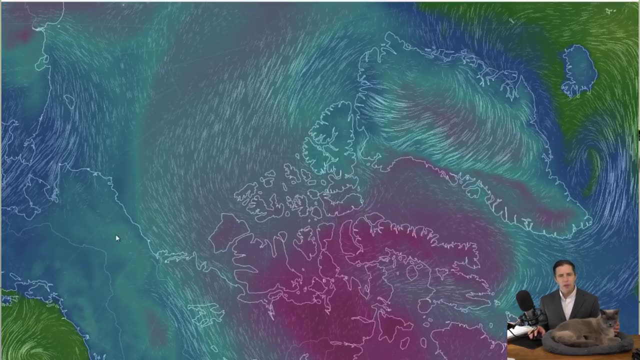 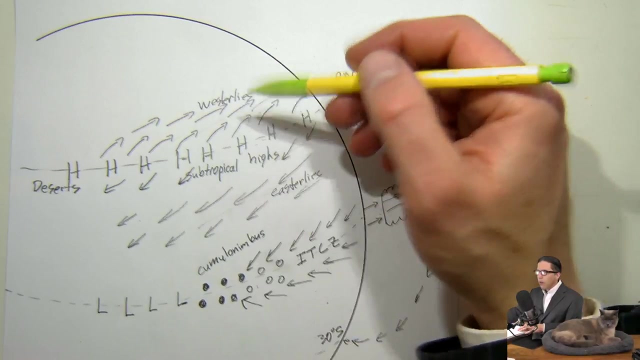 with clockwise rotation right right around there and that forms a band of wind that we're going to call the polar. polar really is. they are not very well developed here, but let's draw a few things on our diagram here. so here's our westerly, so our polar front. we could just kind of say something like this: 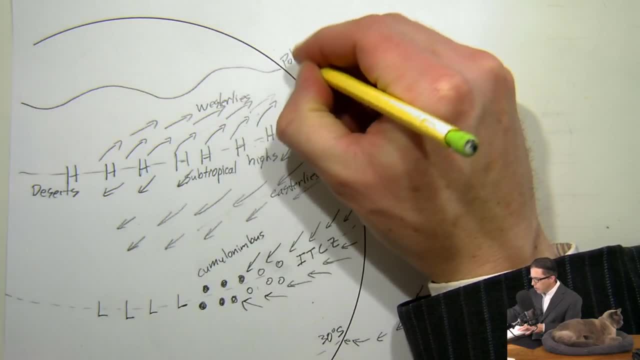 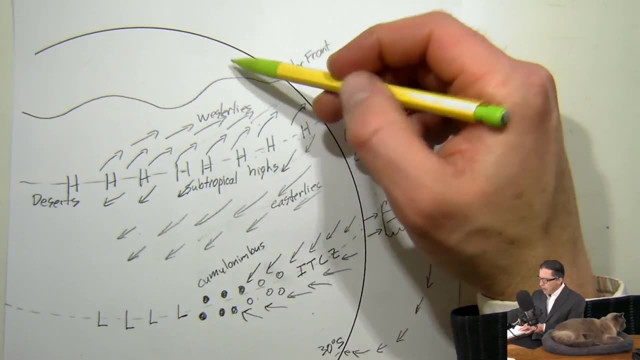 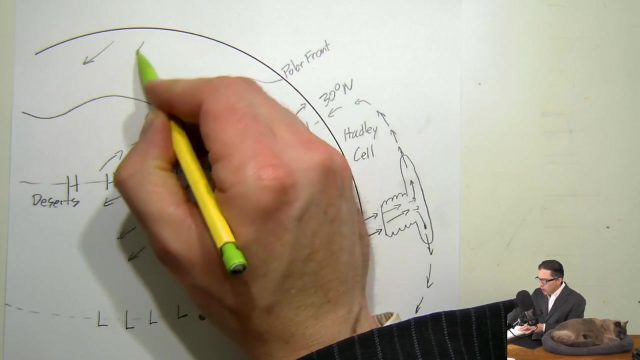 always changing right, but that's an abbreviation or approximation, sorry for where it would be um so up at the north pole. then we've got winds that are spinning quickly, clockwise, and they they're not very well developed in today's animation there, but you've got a high. 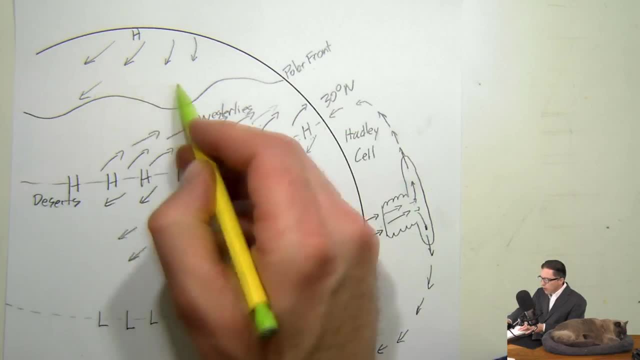 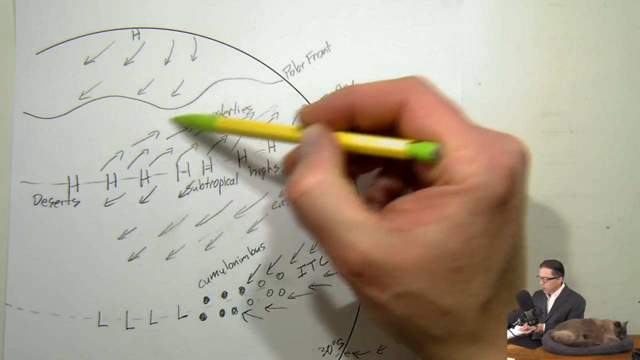 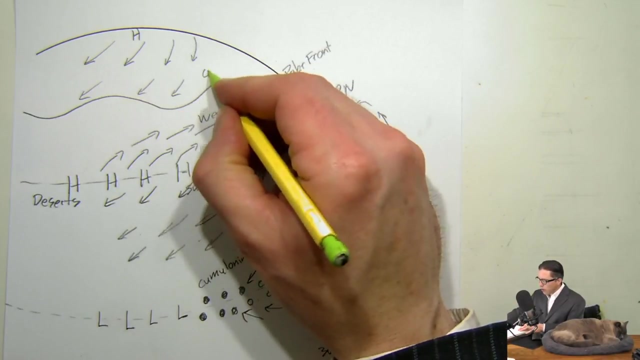 kind of near the north pole with these winds that are coming down this direction, and so right here, right along- here is where we talked about how you get the formation of mid-latitude cyclones right. so you're mixing up this cold air with this warm air and there's a pretty abrupt transition. 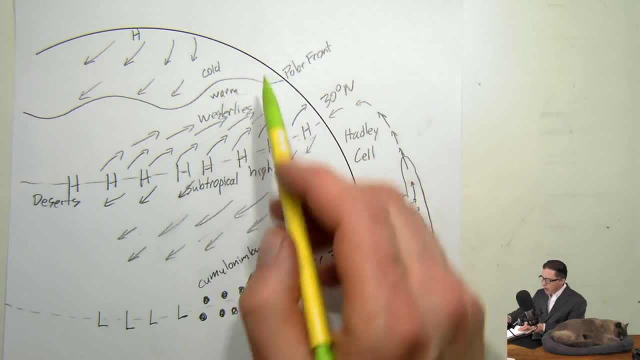 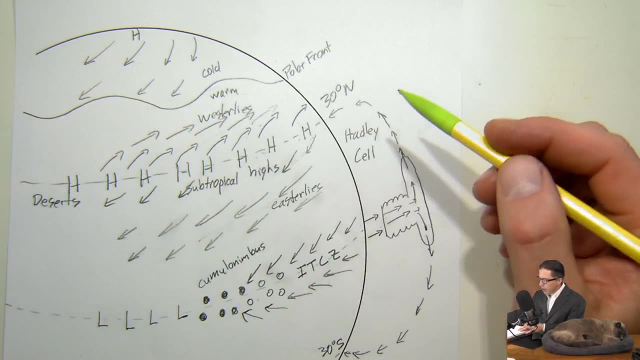 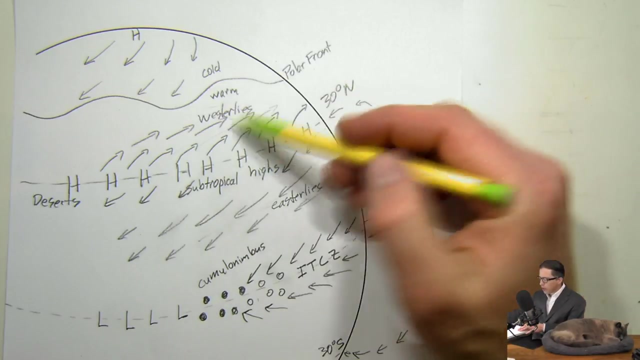 so all the warm fronts and cold fronts, all that stuff we talked about in the past, that's all happening right along that boundary there. okay, so just to kind of fill that out. then warm fronts make air rise because of the ramp. remember that from a previous lecture. 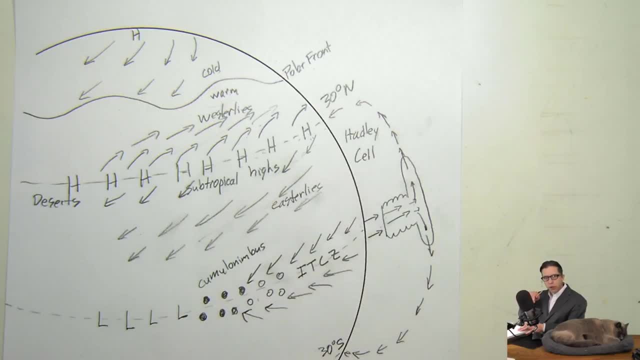 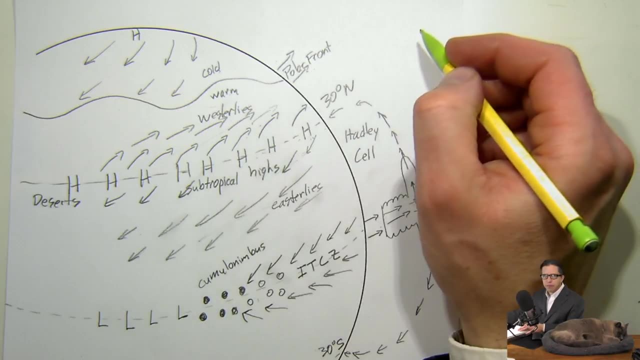 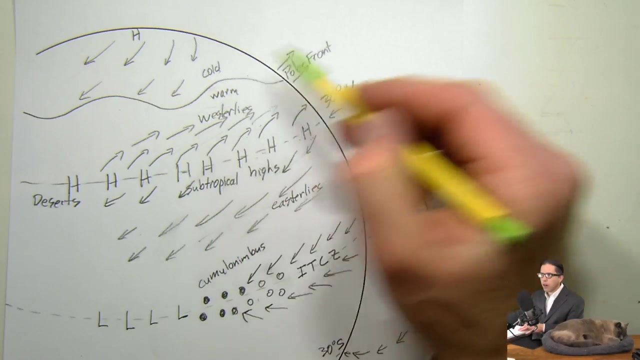 cold fronts make air rise because the cold air tunnels underneath, so you have air that's rising along the polar front. okay, because of those two different types of frontal systems, mid-latitude cyclones, which is what you get when you mix up these two types of air, cause air to rise. so some of the air rises and then kind of 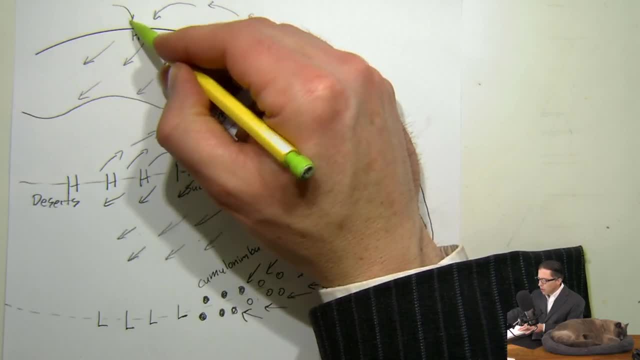 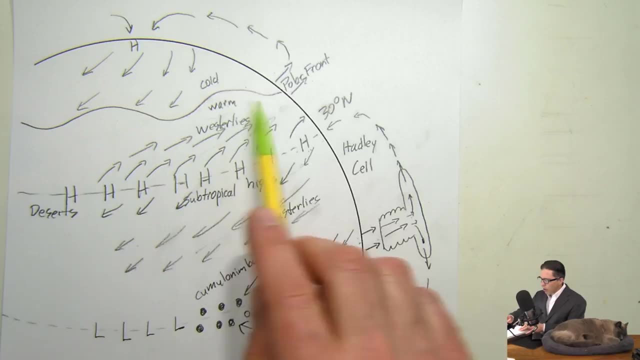 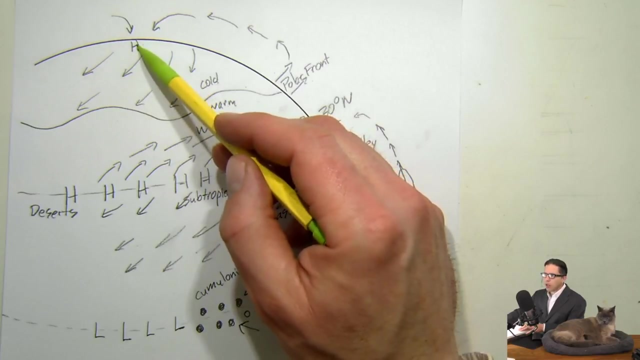 settles down along the north pole. okay, so there's a. you know this is happening all the way around. you know again, this is happening all the way around the earth here. so it's not just rising in this one spots all the way around and sinking down around the north pole, creating a high pressure clockwise. 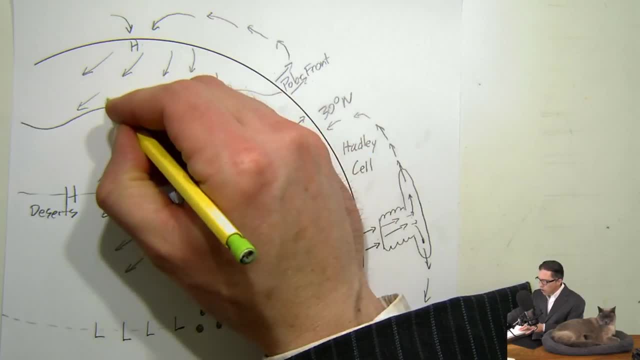 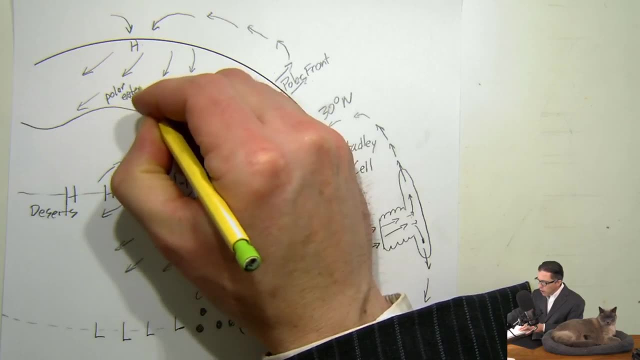 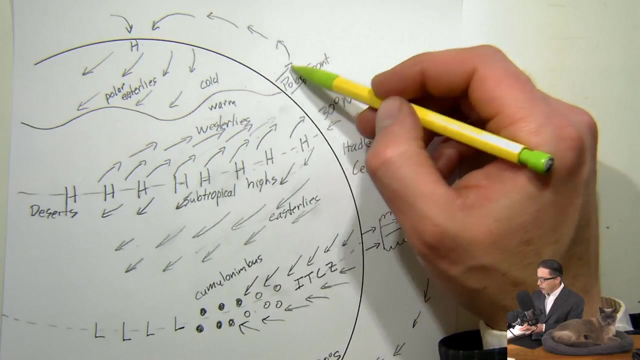 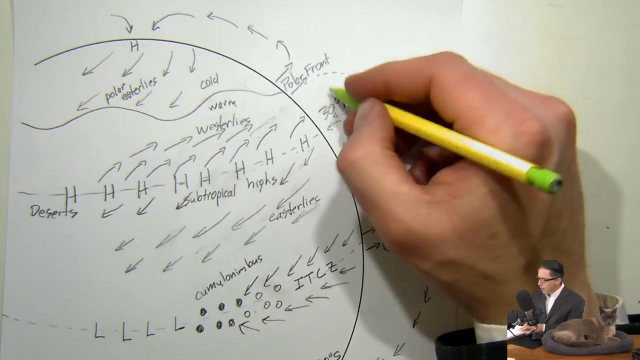 rotation around a high. you get these winds that we call the- uh, polar easterlies. you can read that: polar easterlies, all right, so air is rising from mid-latitude cyclones usually up here, but we can see this little loop here. it's sometimes drawn and this isn't called the ferrule cell. 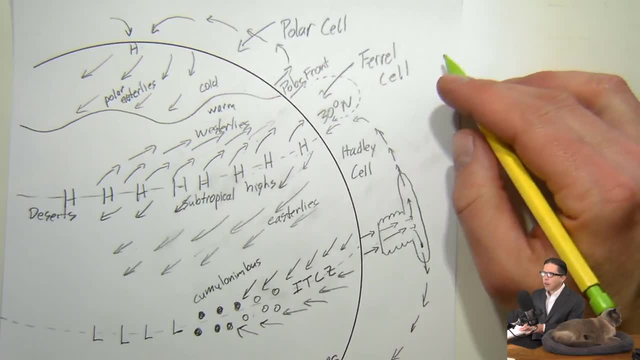 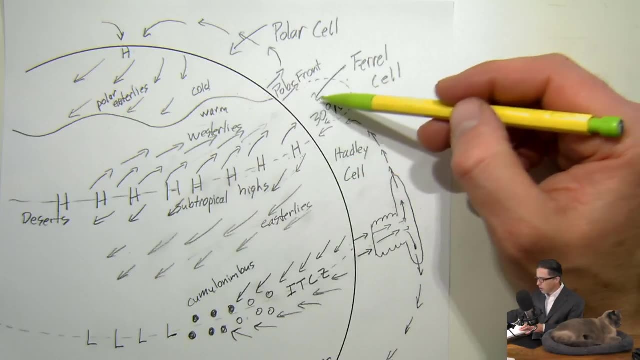 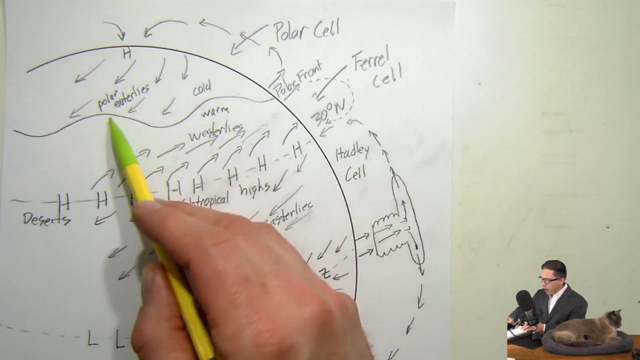 and this is called the polar cell, and we're not really emphasizing these two things. uh, the hadley cell is really the the important one in this class, but you may see this from time to time. these two cells, so Well, the other thing we could draw is those mid-latitude cyclones are going to form right through here as we mix up the air. 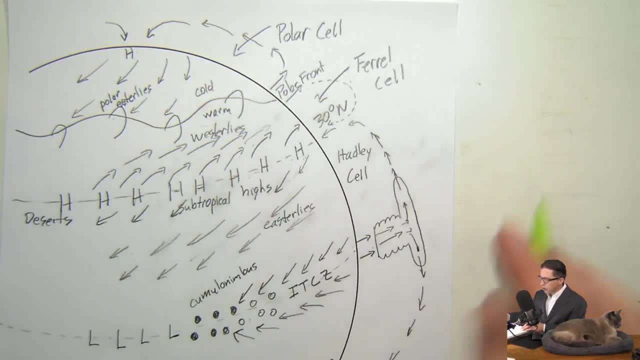 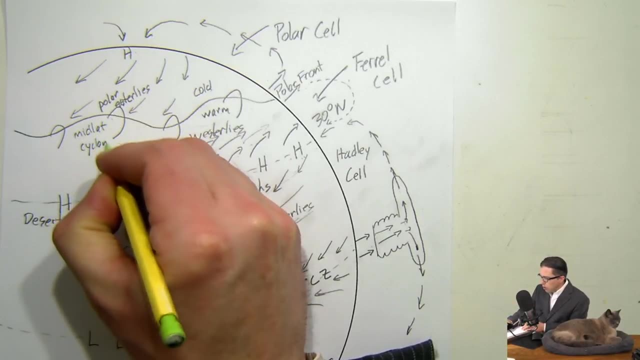 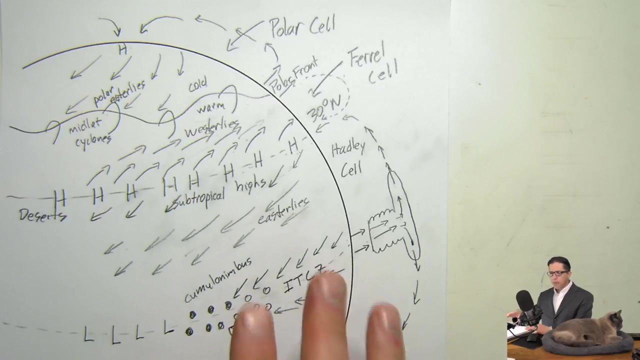 So I'm just going to draw some kind of comma-shaped things just to illustrate that that that's where our mid-latitude cyclones are going to form there. So we kind of have a mess here. but in general, this is the circulation pattern of the Earth's atmosphere. 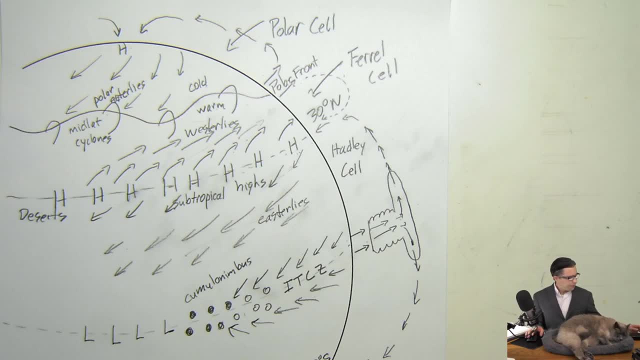 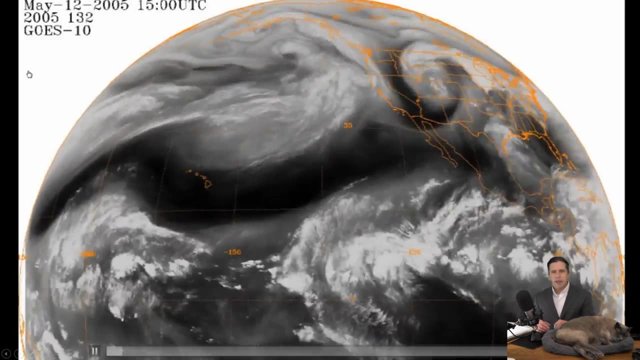 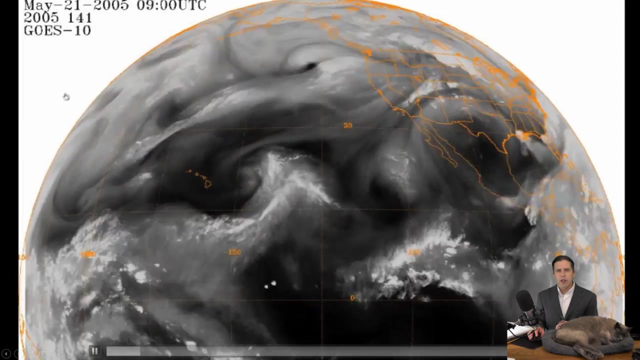 Now let's look at a couple little movies here. So this one, we're looking at not just clouds, but also water vapor. So the gray that you see is water vapor. The really bright white are clouds, And you can see that the clouds are not just clouds, but also water vapor. 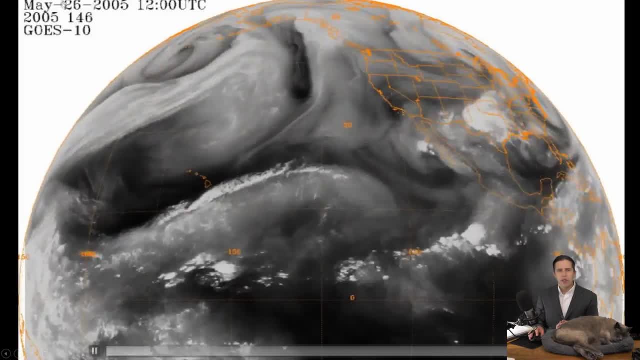 And you can see that the clouds are not just clouds but also water vapor, And each frame is every three hours And you can see the days go by up here. So every three hours there's another frame And you can see some of these features. 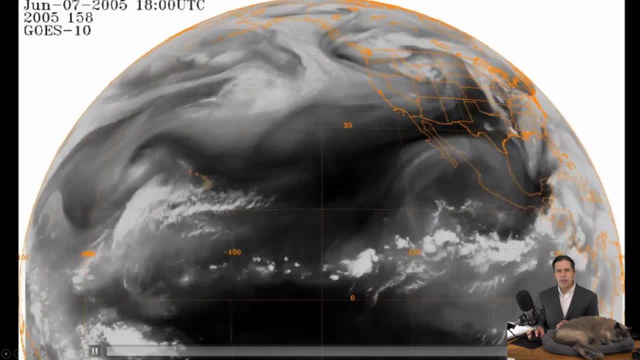 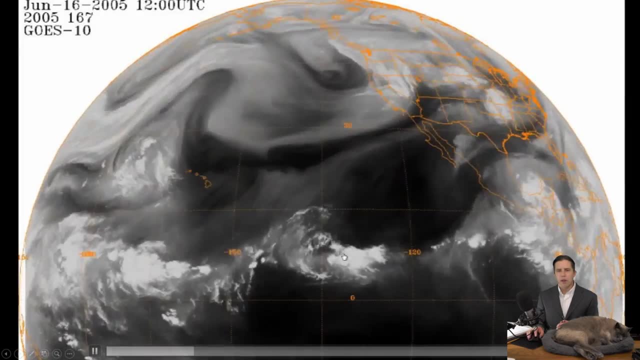 So right through the middle there you can see the ITCZ. So it's just cumulonimbus, day after day after day after day, And you can kind of see the difference between day and night. They'll appear during the day, then they disappear at night. over and over and over. 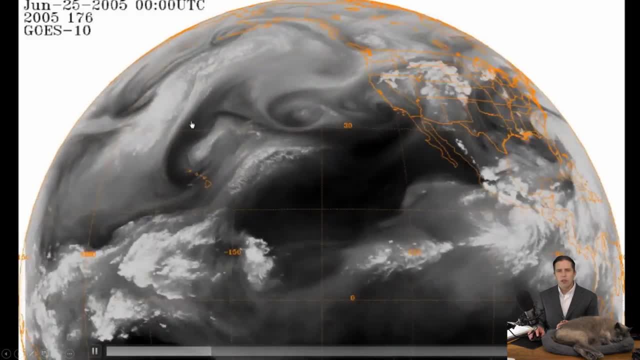 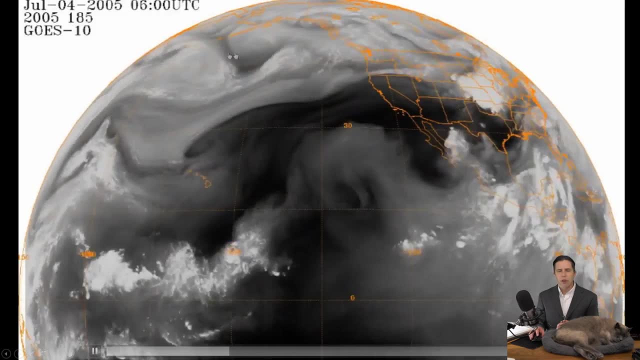 You also see that counterclockwise spiral. There's another one, These little spirals that we get, those are the mid-latitude cyclones. So you'll see the counterclockwise spirals out here, mid-latitude cyclones, the ITCZ down here. 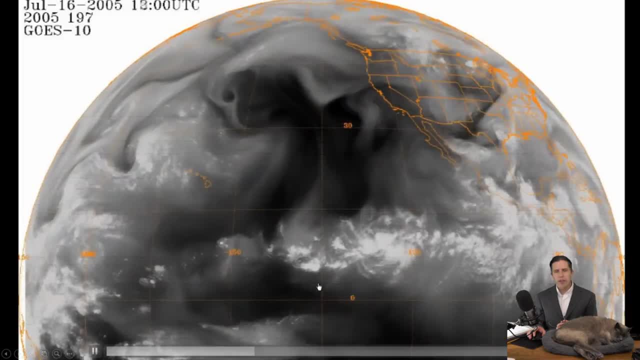 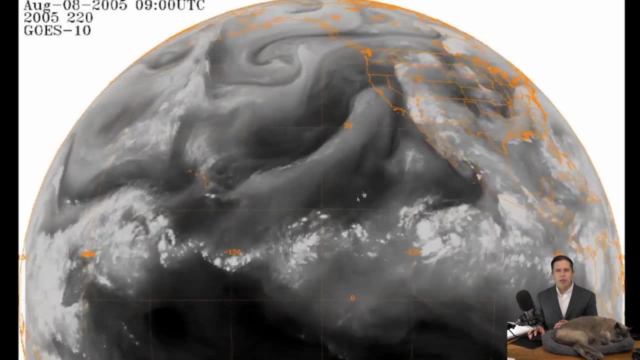 Now, in this image the black is dry air, not near the surface but up in the upper part of the troposphere. And the reason you have: if you watch this for a while, you'll see that there's kind of constantly this black right out in here. 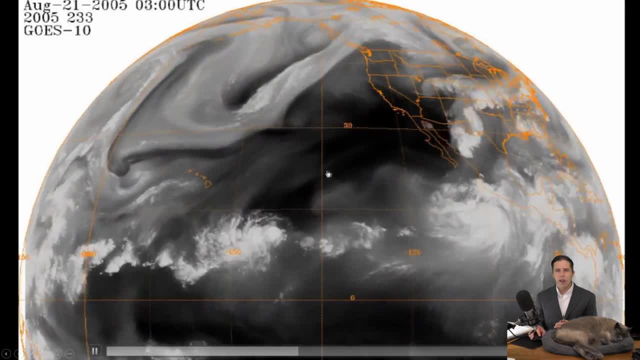 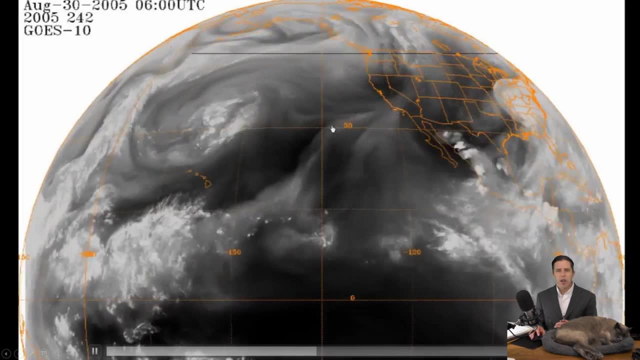 And that is our Pacific Subtropical, That's our sinking air from the Hadley cell, So that air coming down is dry and you can see it gets mixed up from time to time but it'll keep reforming This dark blob of air that's dry, sinking air from the Hadley cell. 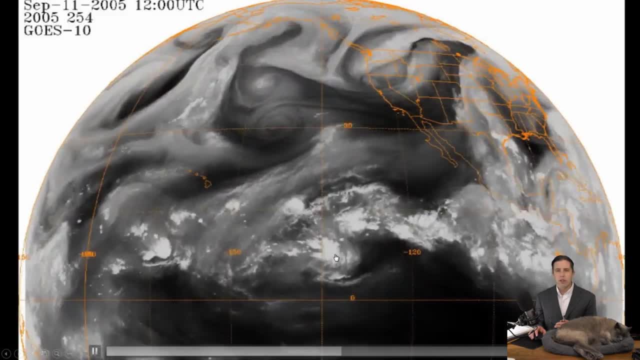 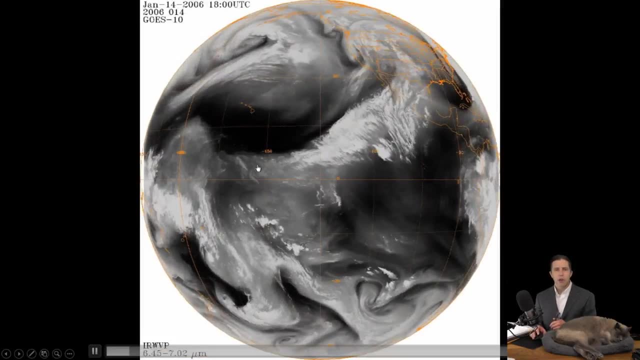 Very few clouds forming in this area, right because of that dry, sinking air. We can also look at it, the whole Earth. Now, this one I made a little slower, but it's the same idea. Every frame is every three hours. 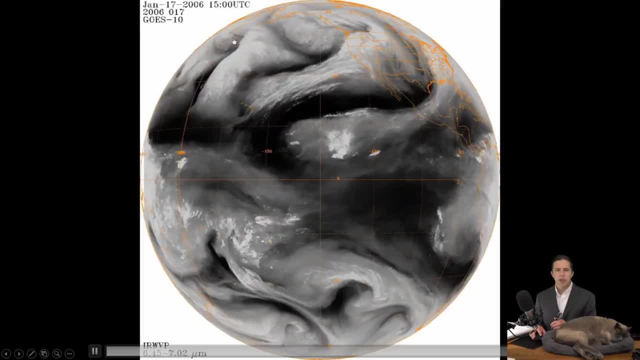 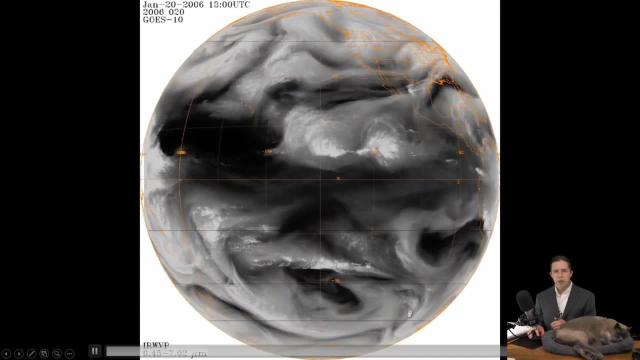 There is a mid-latitude, There's a mid-latitude cyclone, There's a mid-latitude cyclone. Now, down here, you've got them, but they're spinning the opposite direction, So that one right there is spinning clockwise. 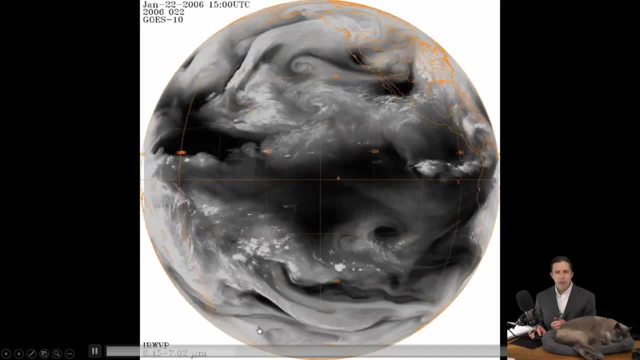 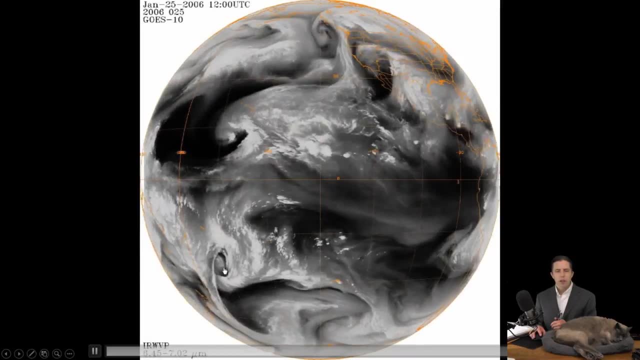 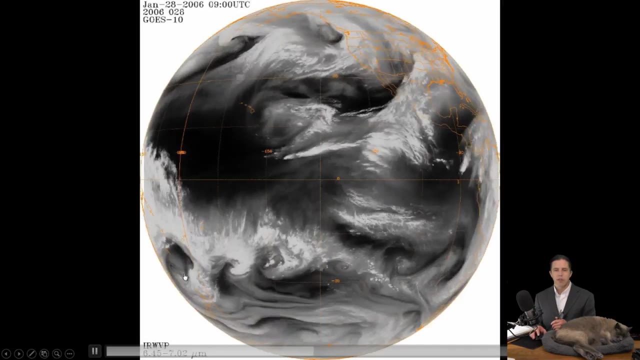 Mid-latitude cyclone. Okay, we're getting trying to find another one. Okay, here's another one. You see these white flashes. that's a lot of times the something happens when they download the data off the satellite and they don't get all of it. 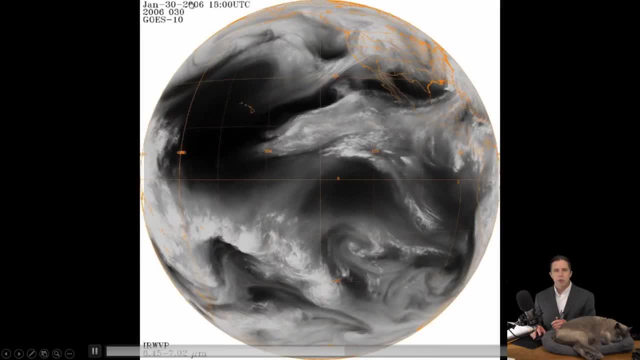 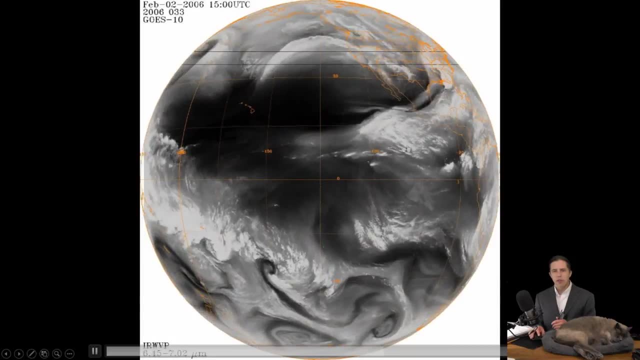 So that's why it's blinking like this. So here and this one's in the winter, the last one was starting in the spring and went to the through the summer. But again you can kind of make out: this is the ITCZ kind of through here. 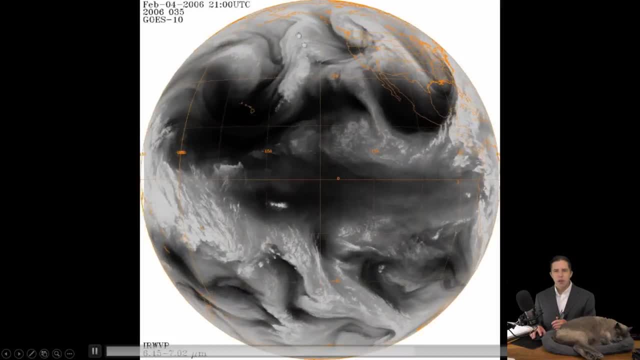 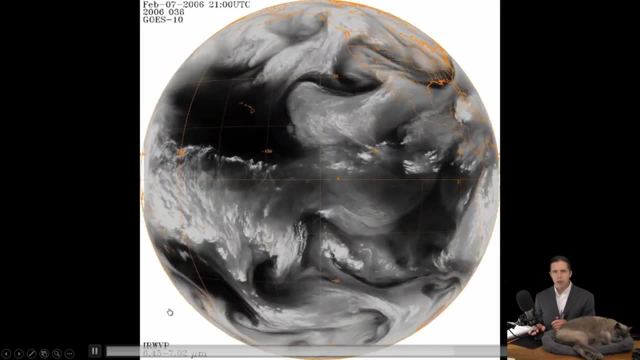 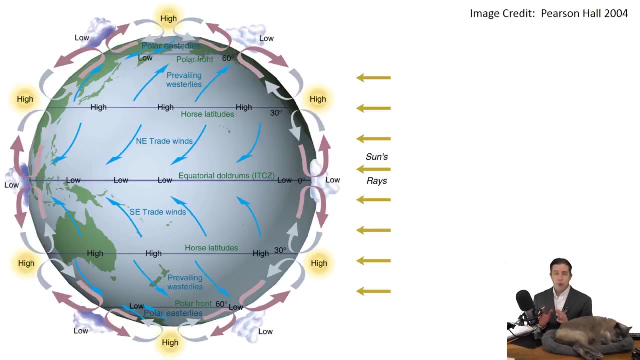 Not as well formed as the last movie. You got mid-latitude cyclones up here. You got mid-latitude cyclones down here, Okay, so that's kind of the global picture. Now, if you see this in a book, it's always shown as a much simpler thing. 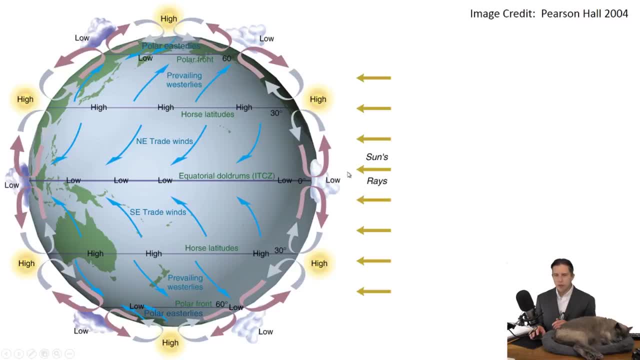 So here's an example of a text, sorry, an image out of a textbook, And what you can see is they show: okay, here's the ITCZs, this nice, perfectly straight line. And then the highs: the subtropical highs are a nice, perfectly straight line. 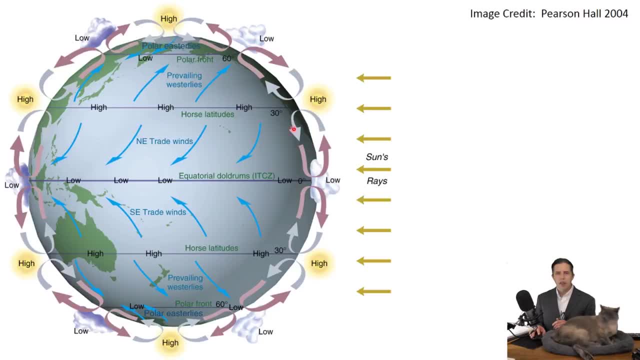 And there's the trade winds, and there's the westerlies, Okay, and then here's the the cells. So this is the Hadley cell, the Farrell cell And the polar cell there, right, So it's nice and neat. 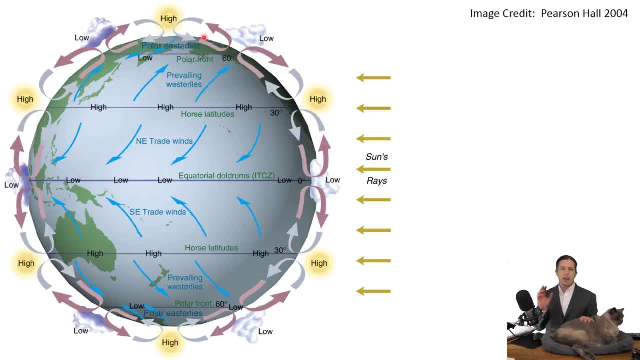 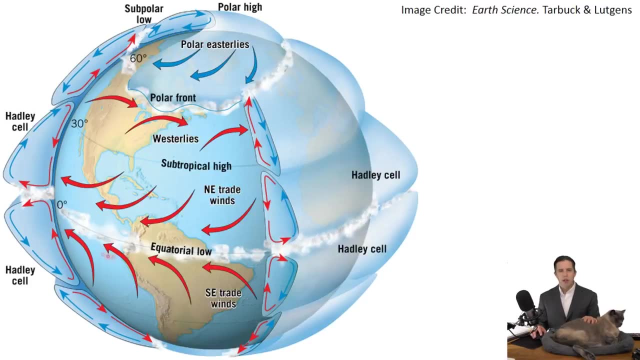 But one of the points I'm trying to make is that it's not nearly as nice and neat as you might read in a textbook. So here's another one. This is more three-dimensional. So here they're showing the ITCZs this nice little band of clouds there. 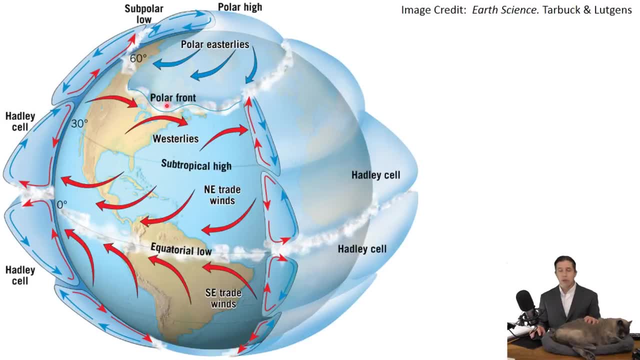 And then along the polar front another band of clouds. Again those are from the cold fronts and warm fronts, And you know there's the westerlies, But again it's not Nearly that nice. If you averaged it over the whole year, it kind of looks like this: 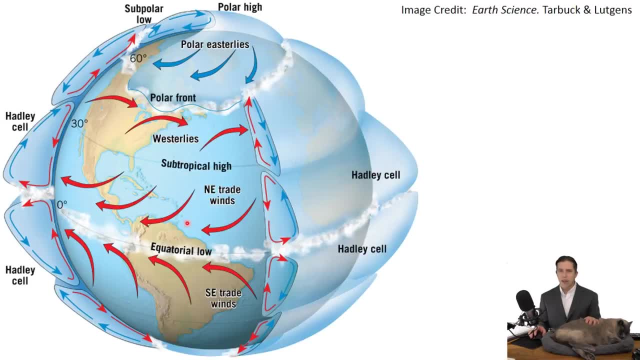 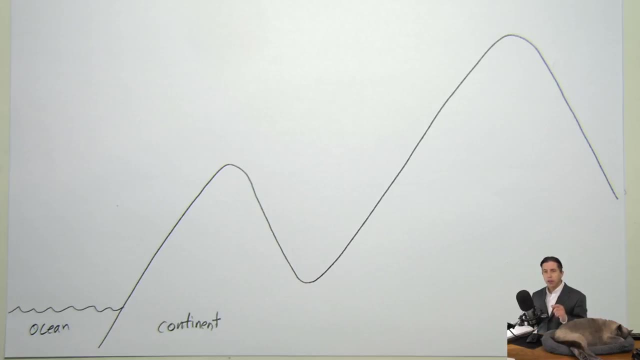 But, as we saw in those movies, it definitely looks very chaotic right. So these are just average patterns, averaged over a long period of time. So one of the small scale things that can have a big effect on your climate is the topography, especially when it comes to precipitation. 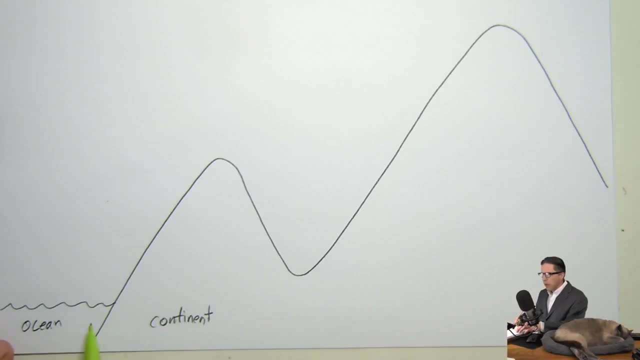 So let's imagine this scenario: We've got this ocean and a continent and we've got a storm that's coming in And I'm going to draw my storm as this little, tiny baby cumulonimbus cloud, But it represents something much more complicated, like a storm system. 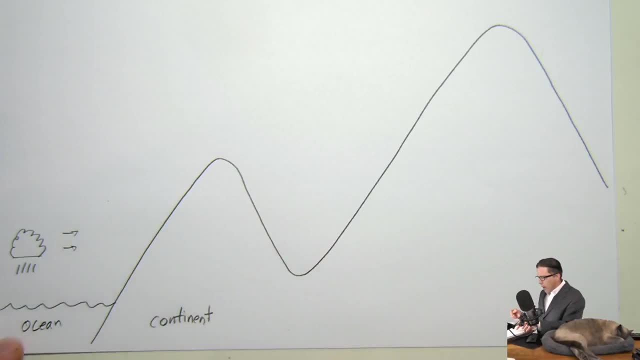 And it's coming inland, And so let's just say it's raining. It's raining out in the ocean And when it hits the continent, one of the things that's going to happen is that that storm is going to intensify. And the reason for that is the continent is usually warmer than the ocean. So the storm's coming along and suddenly it gets a little boost of warm air from the continent And that makes it grow right. So it starts raining more. But now this storm has to go uphill. 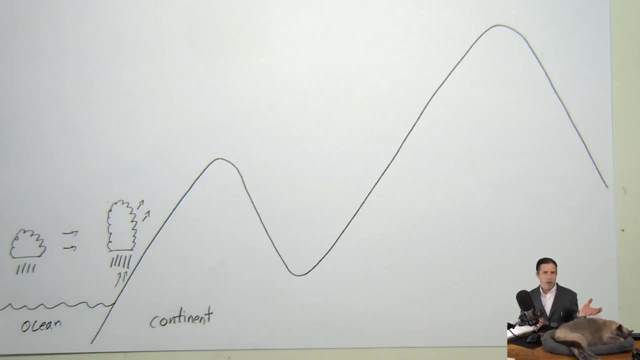 Now, when we talked about convection, we said that if you can make air go up, air that moves up, expands It, cools, eventually hits the dew point, makes a cloud. If it continues to go up, you can eventually make ice, creates precipitation. right. 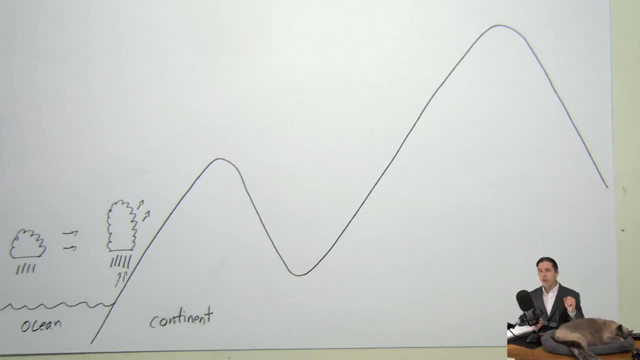 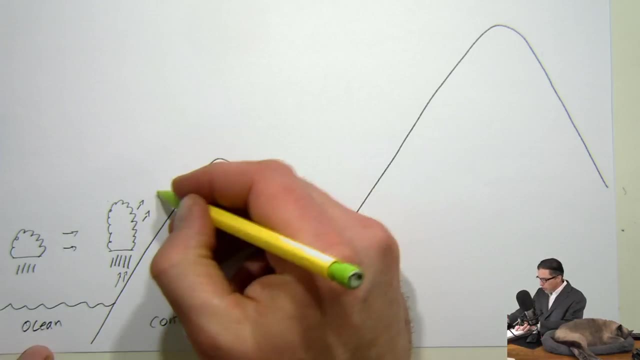 That's how you get precipitation, that whole process. What if you already have a storm and you make the whole storm go up? The storm will intensify. So this storm that I'm drawing as it goes up the mountain will grow and become stronger and stronger as it grows. 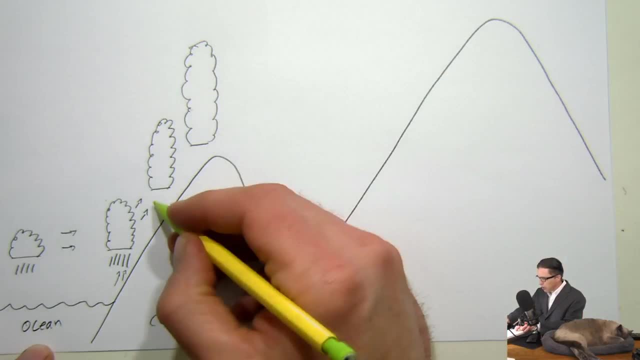 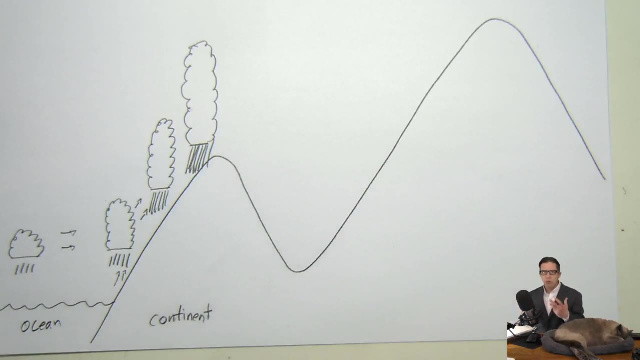 And I'm again simplifying by just- I'm just drawing cumulonimbus clouds here, But as it goes up the mountain, it produces more and more precipitation as it's forced further and further up. Right, okay, so this is the storm going up. But what happens when the storm goes down? Well, sinking air fights cloud formation. Take a storm and make it go down, and the storm will get weaker. It's going the opposite direction that it needs to go. So what happens is, as it goes down the hill, it becomes weaker. 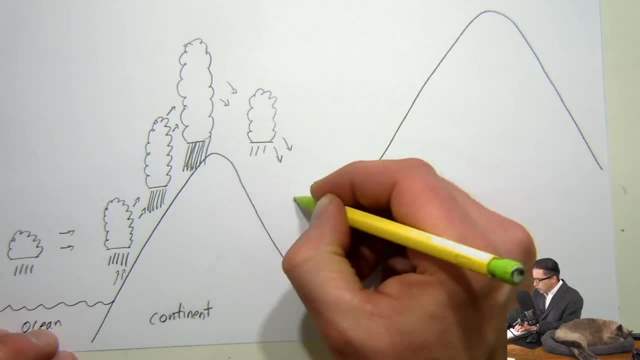 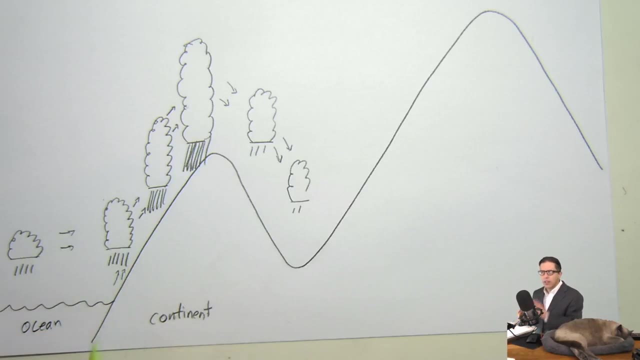 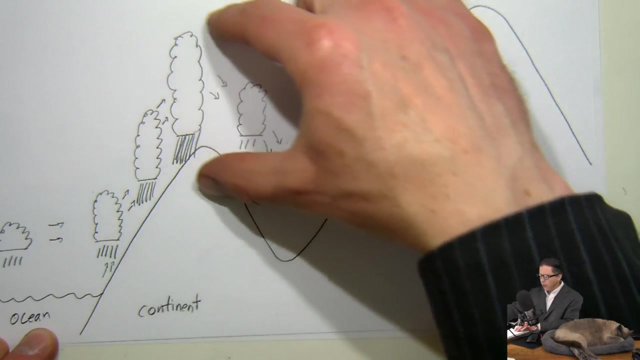 However, it's not exactly symmetrical to the other side, because it's now lost some precipitation over here, right Once it left the ocean. it doesn't really have a source of humidity anymore. So as precipitation is occurring, you can think of this entire column of air. the dew point is going down as the air moves inland right. 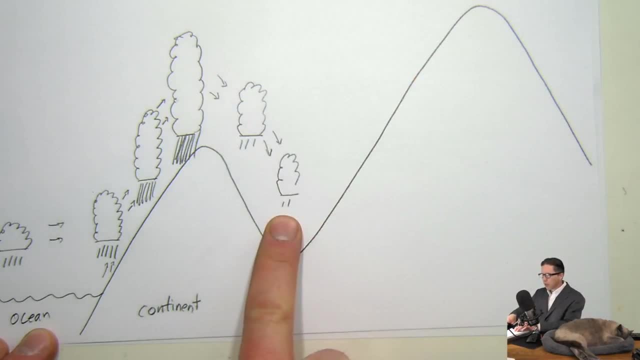 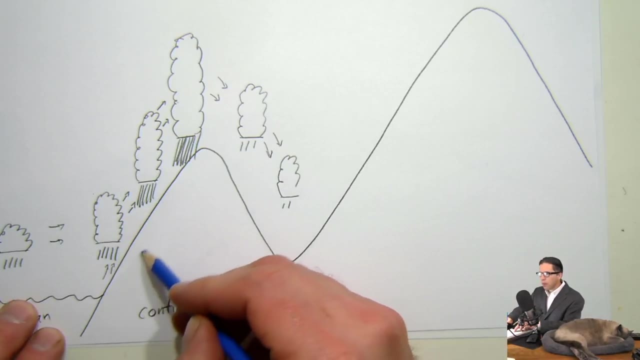 It's losing water as it goes, So this is not producing as much precipitation as it did on the other side. Okay, so this means that if you were to go up the mountain here, you would experience more and more precipitation on the way up. 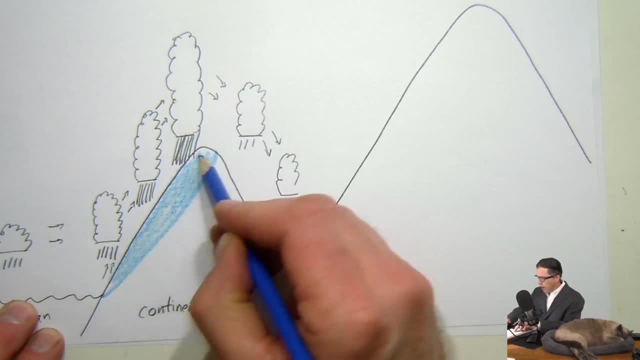 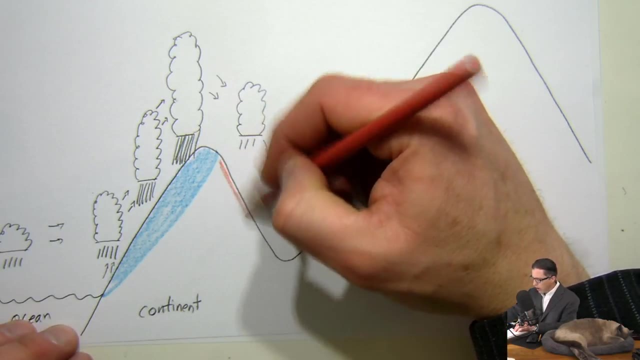 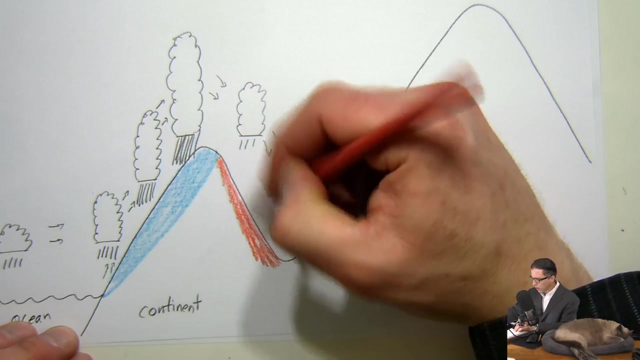 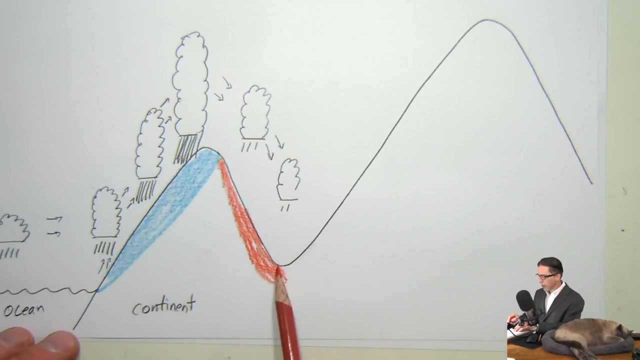 So we have a wet side of the mountain And then on the other side we see a side that's considerably drier as it goes downhill And gets drier and drier Towards the bottom, Something like this: And so by the time the storm gets to the bottom of this hill, this is the driest point so far. 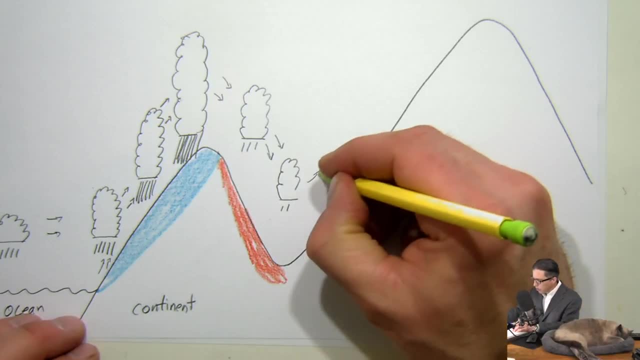 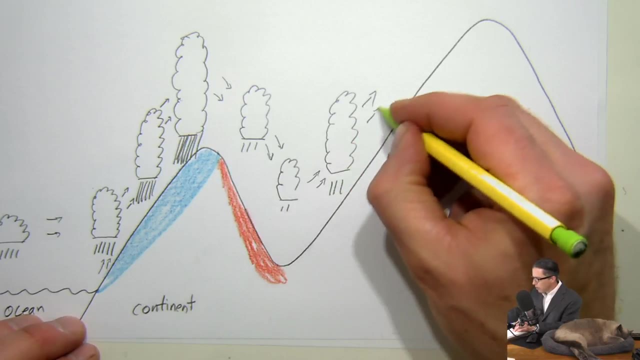 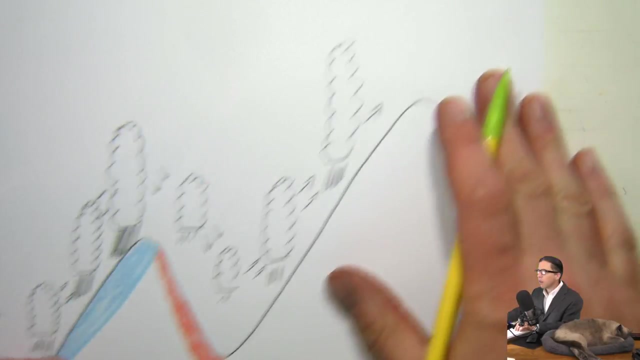 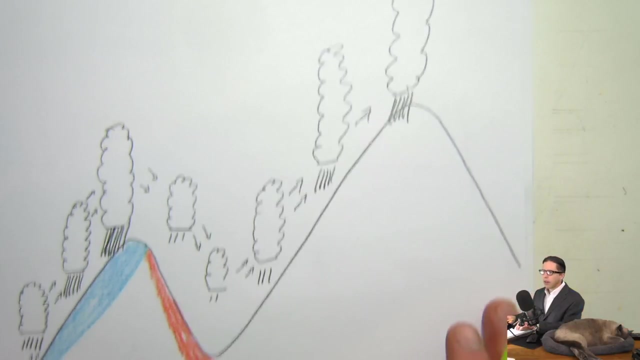 But now it's going to go back up, right. So now it's going to go back up this next mountain. So, once again, the storm intensifies. Now it's going to rain more as it grows And, like the little mountain it's now, the precipitation is going to increase as it goes up this second mountain. 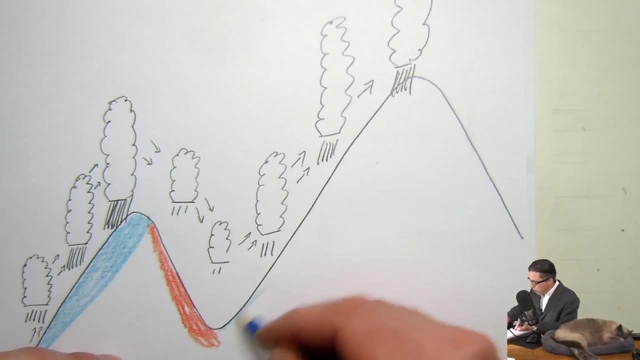 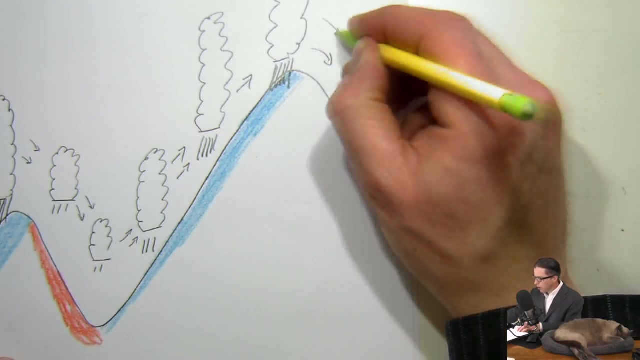 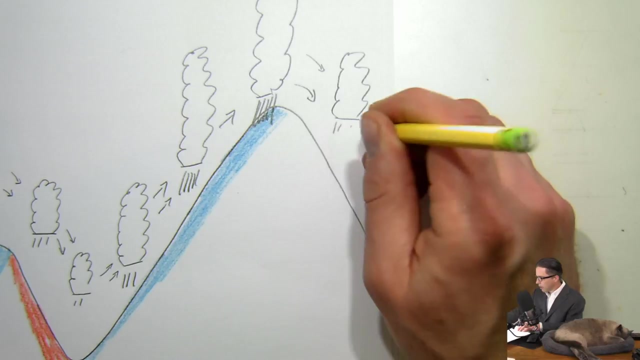 So now we get another zone that increases with height, A wet zone, right. So we get that. Now it comes down the other side And now, as before, this storm is on its way down And it weakens, And it weakens a lot. Because now it not only has lost all of the precipitation coming up the first mountain, it also lost precipitation going up the second mountain, And now it's got a long ways to go downhill. So this mountain, this side of this mountain, is going to be even drier on this side. 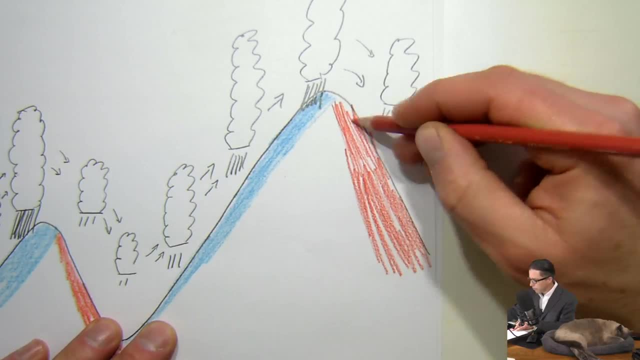 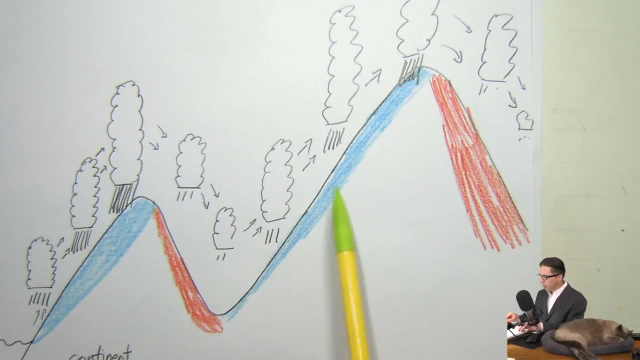 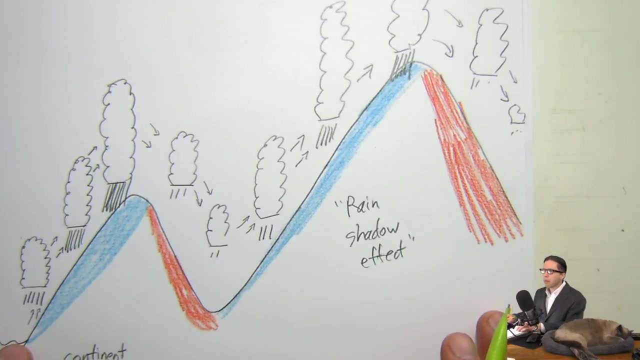 Than the first one. So these mountains have very different climates. You've got a wet side and a dry side, A wet side and a dry side. This is called the rain shadow effect, The rain shadow effect. So if you live in a place where there are mountains, 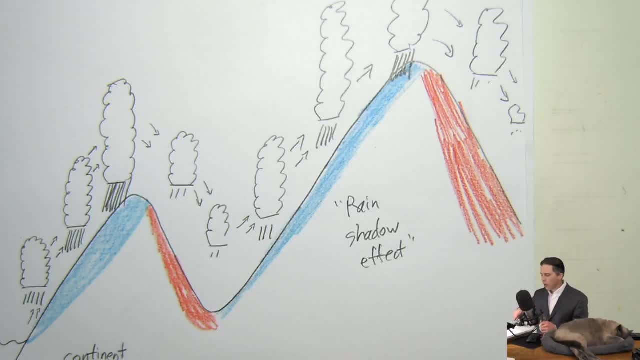 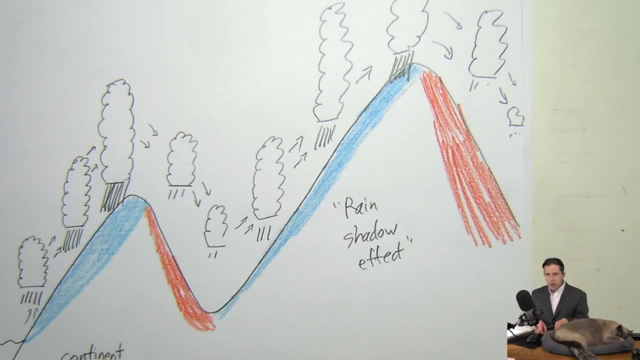 and there's a preferred direction that the storms come from. you might live on the wet side or you might live on the dry side And you'll have completely different climates. So this goes on a lot in the western part of the United States. 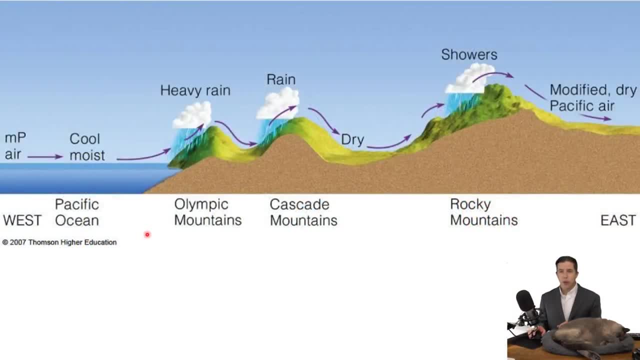 So this is a diagram out of a textbook showing the rain shadow effect as a storm moves in over Washington State. So they come in over the Pacific, go up the Olympic Mountains, which are on the west coast, So they intensify as they go up. 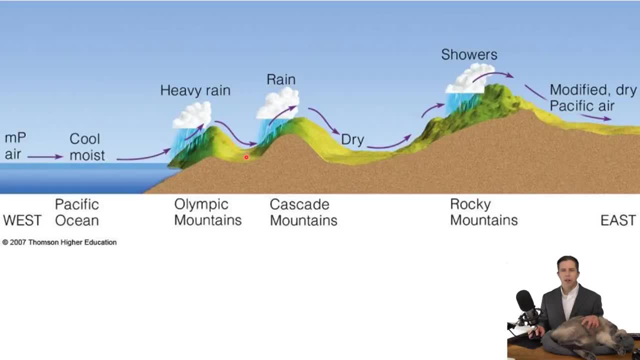 They weaken as they go down. You have a relatively dry spot here. Then they go up the Cascade Mountains, which are a chain of volcanoes, And they intensify on the way up And then dry on the way down. Then it's pretty dry, as we'll see in a second, across eastern Washington State. 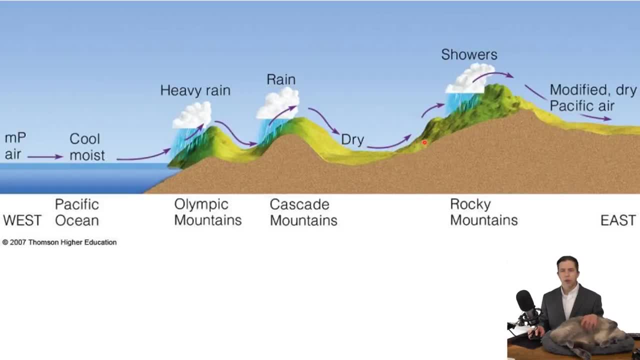 And eventually they get to Idaho And in Idaho they go up the Rocky Mountains and intensify again And you get a little bit more moisture before coming down the other side And it's really dry again. So we can see this on a map of precipitation of the US. 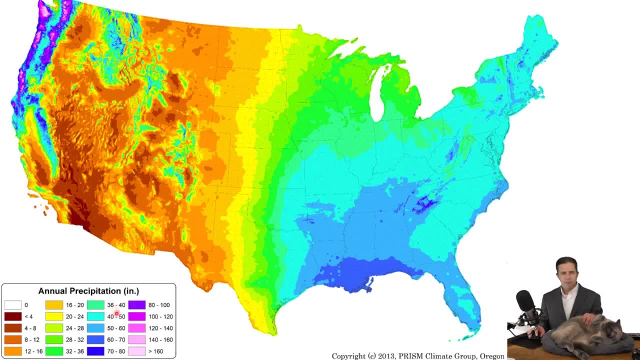 So these colors represent annual precipitation. Here's a scale down here, And if we look over here on the west coast we can see there's kind of a purple stripe right there And another purple stripe right there And those are two stripes of really intense precipitation. 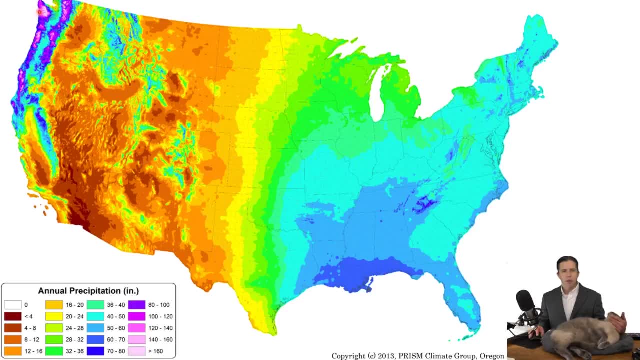 So storms come in. So there's Washington State. So right there, that's the Olympic Mountains. They come ashore and intensify, go uphill, dump a bunch of rain. Now how much rain are we talking here? So over 100 inches. 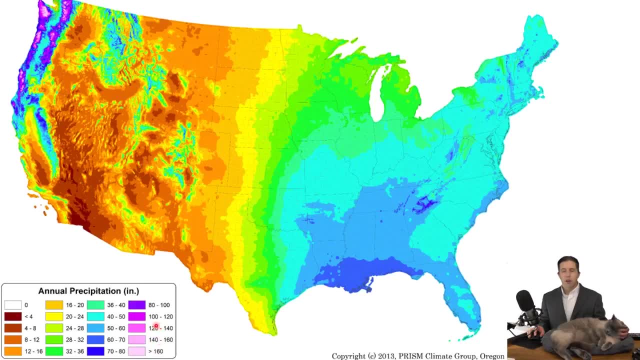 So that white area 150 inches or so of rain Again. this also can fall as snow, but rain equivalent. So if you're from New Mexico, you know 150 inches of rain just does not compute to our brains, So it's hard to imagine that. 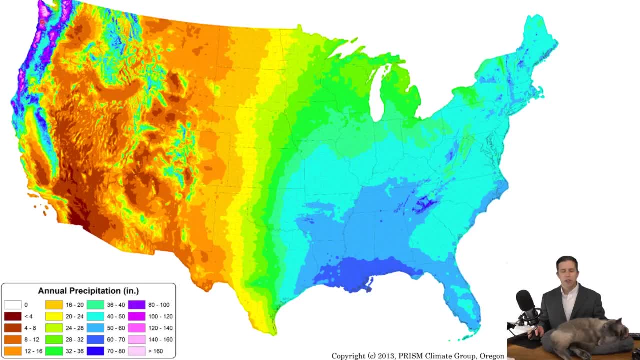 But you have all this rain coming out on this mountain range here to the west. If it goes downhill, you have a relatively dry spot here. Then it goes up the Cascades and you get another wet stripe. So you've lost precipitation here and you lost precipitation here. 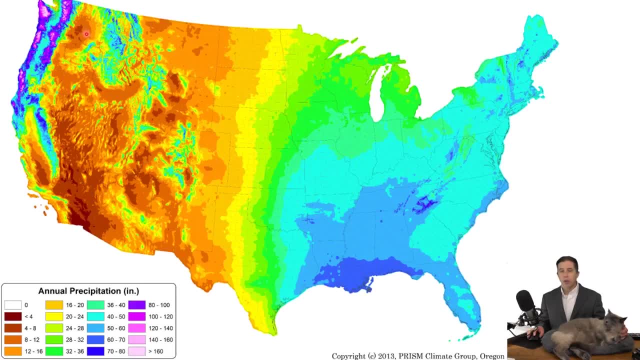 And now the storms are going downhill And suddenly Washington State gets really dry. Washington State is a pretty extreme example of the rain shadow effect. It's called the Evergreen State. That's their logo, So over here it's rainforest. 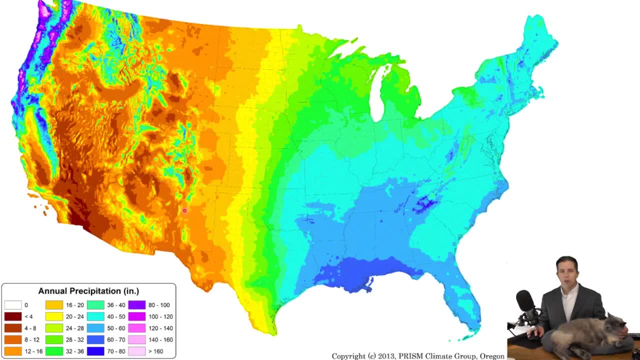 Over here. That's the same as most of New Mexico. There's actually areas in eastern Washington State that are drier than New Mexico, So you've got desert right next to rainforest, not that far apart. That's the rain shadow effect. 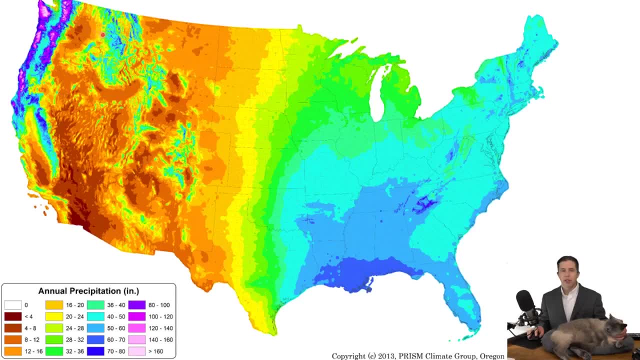 Storms come downhill, downhill, downhill, And then they finally get to the Rockies. They start to go uphill again And you get intensification over here in Idaho. Then they go back downhill again, And so now it's really dry again over here in Montana. 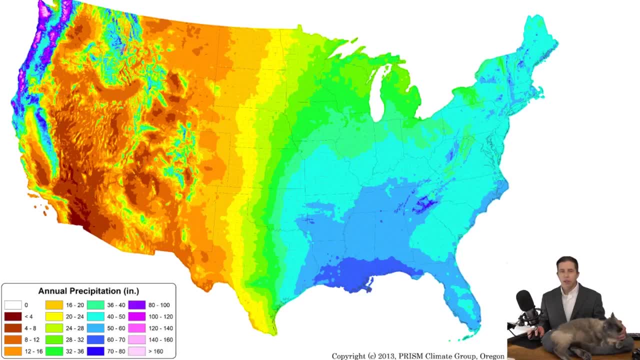 So that's an illustration of the rain shadow effect, Which really affects all of the western part of the United States. So you can see this effect all the way down here into California, Where you've got a lot of precipitation on the western mountains. 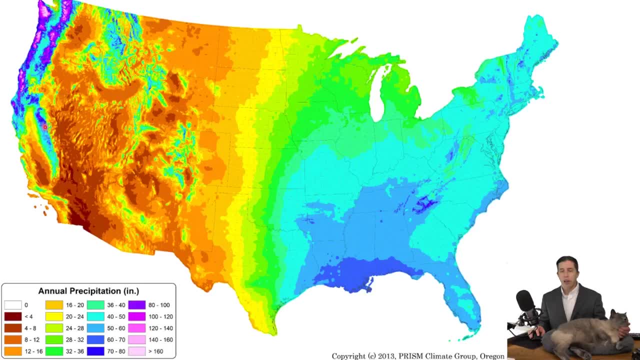 And then you've got a little break. And then here, for example, that's the Sierra Nevada mountains. Same idea: The storms come in, They hit the coast, They dump, They get into Central Valley, They weaken, They go up the Sierra Nevadas, They strengthen again. 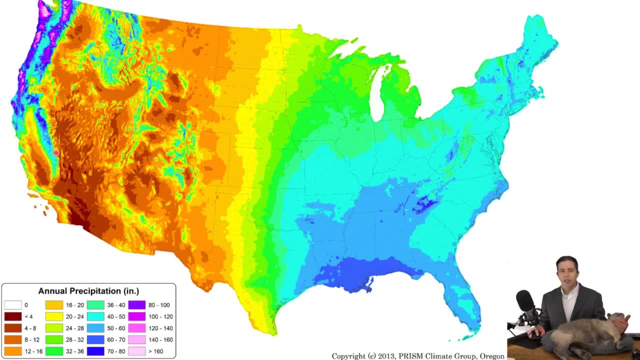 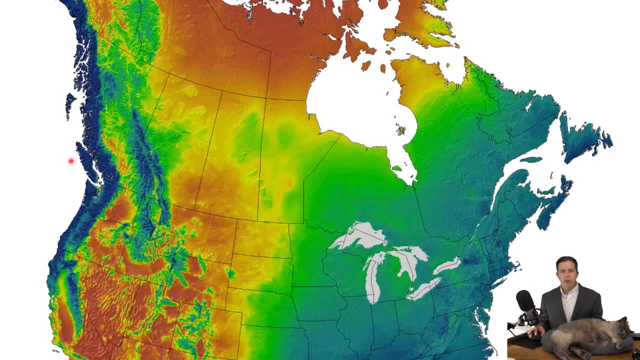 They come down the other side. Now it's in rain shadow again, So it's super dry over here in Nevada. You can also see this on a bigger scale. So if we extend this map up into Canada and Northern Territories, Here's this blue stripe. 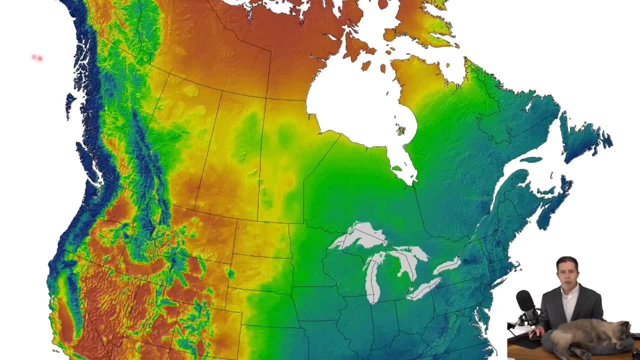 This is the wet west coast, And so even up here in Canada This is all mid latitude cyclones. They're coming in, They're dumping precipitation along the west coast here And then as they move inland It's drier. You get that rain shadow effect. 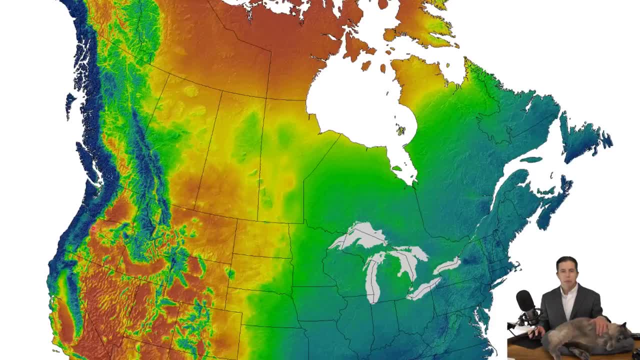 And they have a very dry inland part of the continent. Another thing this shows is that you can see where the mid latitude cyclones kind of stop. So during our summer, mid latitude cyclones are coming across up here. We're not aware of them. 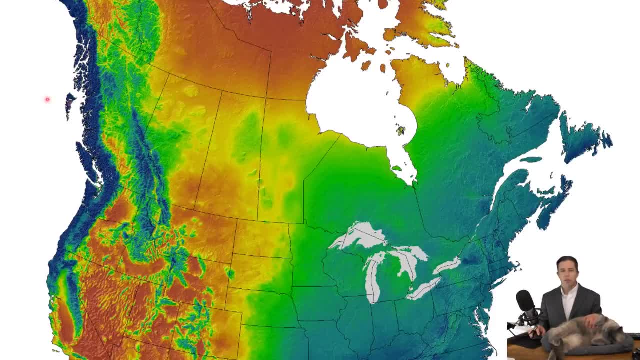 That's why we call them winter storms. But they're still hammering the coast up here And then in our winter They come down and get down into right about the middle of California. That blue color disappears. So mid latitude cyclones are rarer and rarer the further south that you go. 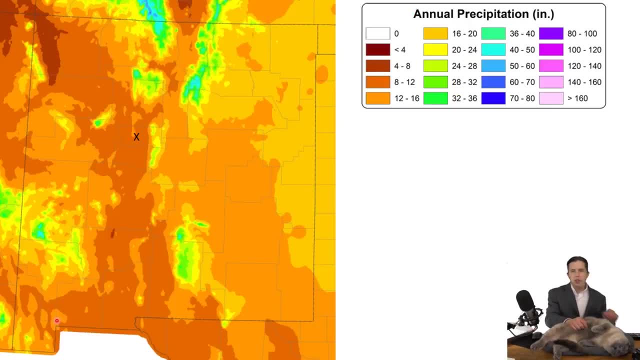 Okay, let's see here. So let's look at a map of just New Mexico for a minute And you can see that. So there's the outline of the state, right, You can kind of make it out there. And there's Albuquerque. 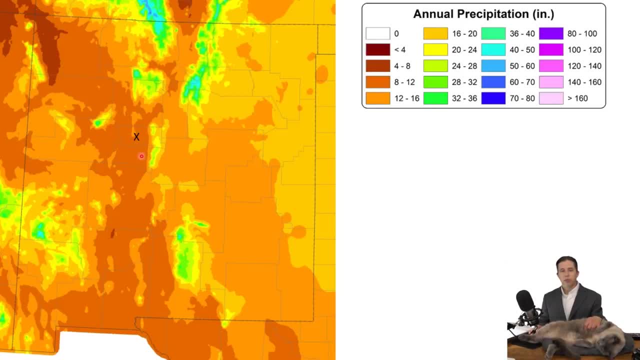 We're the X And you'll notice that Albuquerque Is really in almost the driest part of the state. There's a little bit something dry right there, But really this color, this orangey color, here It's among the driest parts of the state. 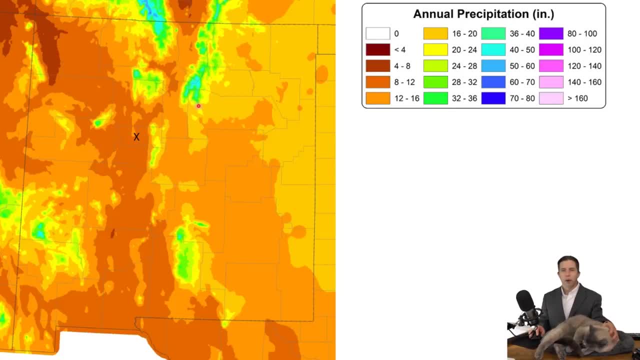 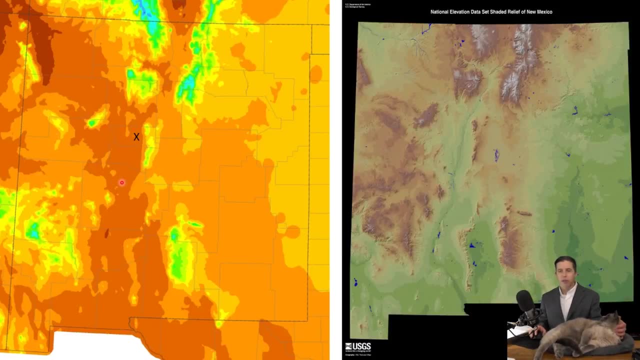 So if you go in any direction, You'll run into parts of New Mexico that are wetter. Okay, so why is this? Well, I'm going to throw up another map here of elevation And we can compare these two things. So Albuquerque is right in here. 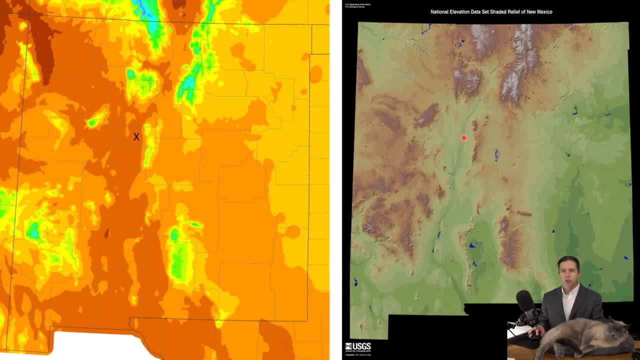 And this is the Rio Grande Valley right. It comes down through here And it's at the lowest elevation locally. So we live in a spot that's among the lowest elevation in the state. So if you're a storm coming from the west, 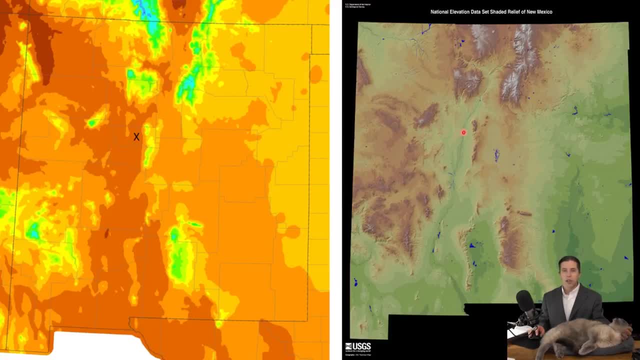 You got to go downhill to get to Albuquerque, Which means you're weakening as you go downhill. If you're a storm coming from the north, You're weakening as you go downhill. Coming from the east or the northeast- Weakening as you come downhill. So, no matter which direction a storm comes, Unless it's coming directly from the south, It's got to go downhill to get to Albuquerque, So it weakens as it approaches us. So this is what happens all the time. You may have had this experience. 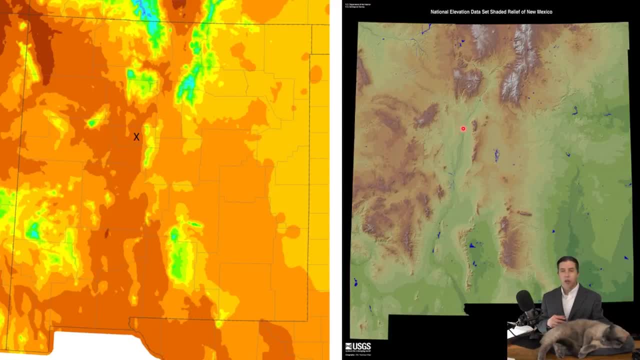 We have a winter storm warning, for example, And you're like, oh boy, maybe it's going to snow, We'll have a snow day tomorrow, no school. And you wake up in the morning all excited And you look around and you see snow everywhere around us. 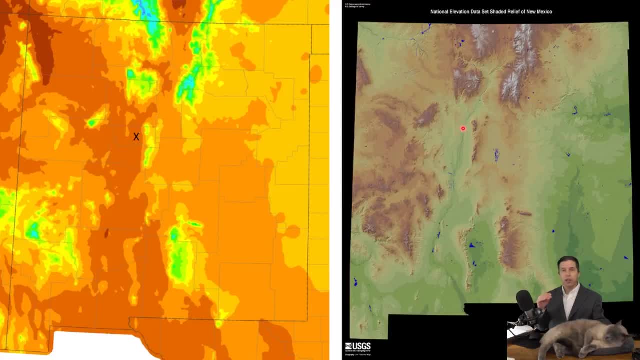 But not here in Albuquerque. Why? Because we are at locally a pretty low elevation, So that storm that may have dumped snow all around us Weakened as it approached Albuquerque, And you can see on this map also That this, the Rio Grande Valley, comes down this way: 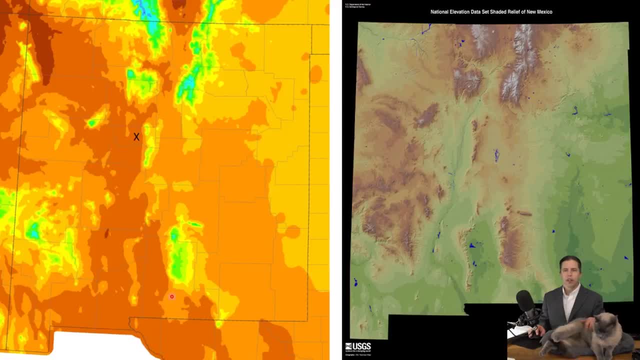 So all of this is really dry Because it's a low elevation And this blob right here, Right, This is pretty wet Because this corresponds to this mountain, This little wet blob here corresponds to this mountain, This little wet, you know, this wet blob right there. 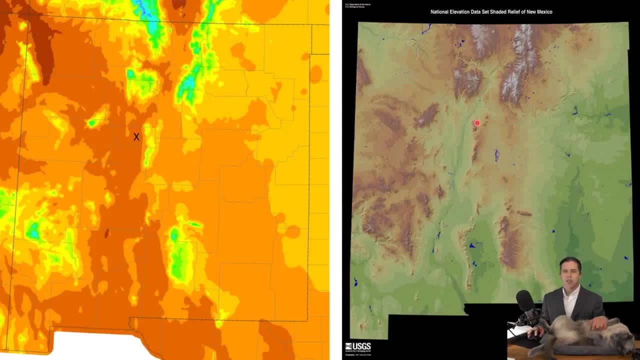 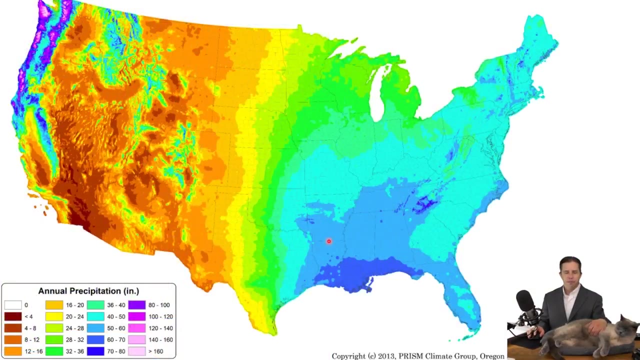 Corresponds to this mountain, etc. So places that are of high elevation get more precipitation Because storms are forced up over them, Which enhances the precipitation. Then they come down the other side and they're dry again. So let's return back to this map. 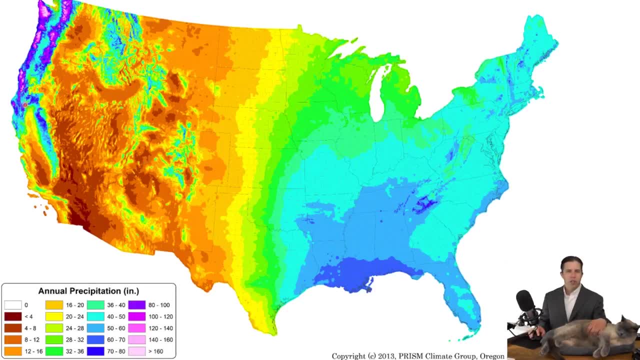 And talk about a couple more things. So we talk about rain shadow effect here. This is pretty dry down here And there's more than one reason for that. We do have lack of mid-latitude cyclones. They don't get that far south. 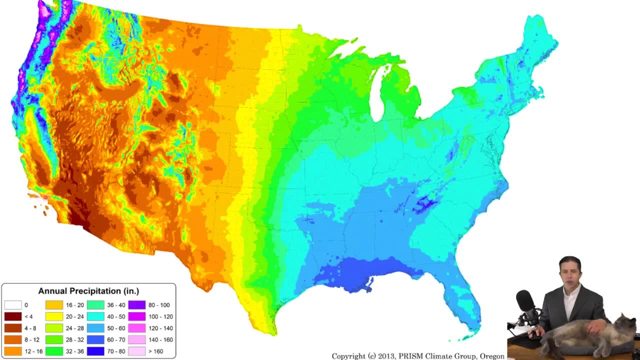 We have rain shadow effect, So the ones that actually get this far south, They lose their moisture on the coast. But we also have the fact that we are under the influence of the Pacific Subtropical High. Pacific Subtropical High sits right out here. 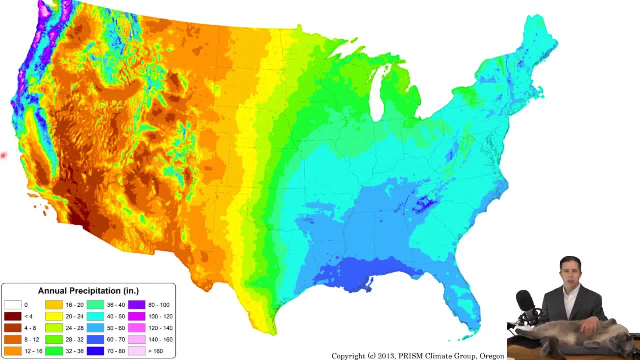 Out in the ocean And influences this part of the country kind of right in here- Southern California, parts of Nevada, Arizona, New Mexico, So all those things combine to give us a very dry climate. Notice something weird happens kind of right in the middle of the country. 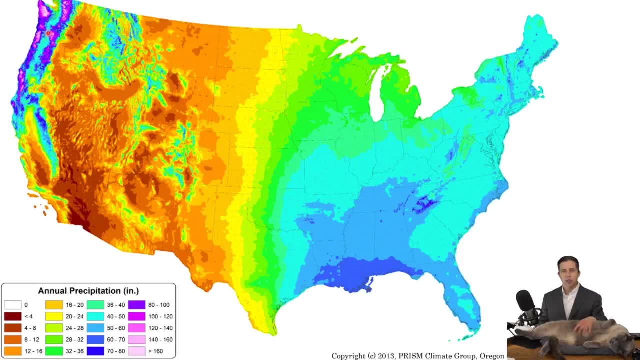 If we're a mid-latitude cyclone and we're coming in and we dump our precipitation on the west coast on the mountain ranges, Then we have that rain shadow effect and it's pretty dry. Then we come down out of the Rockies, Then it picks up moisture. 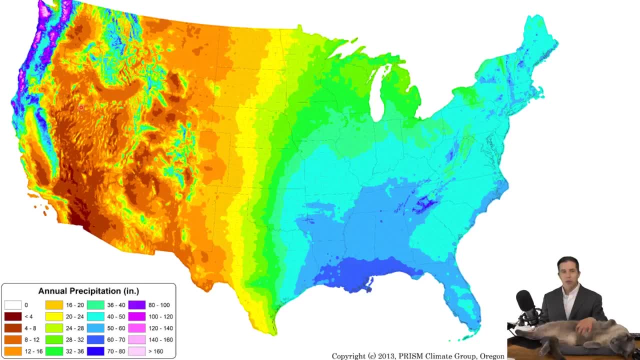 And we see an increase of precipitation. Now, how could that be? Well, if you're a mid-latitude cyclone coming across, you've lost all of your moisture as you came across here, If you think of it in terms of like dew point of the air. 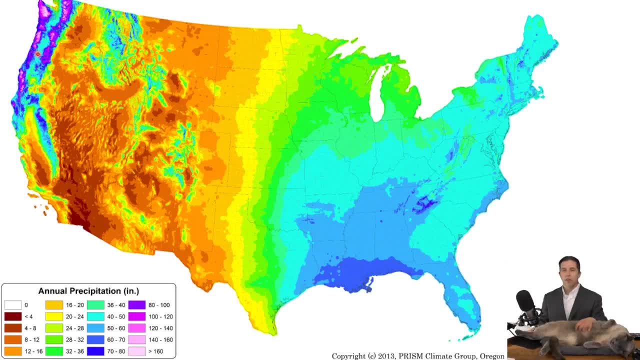 The dew point of the air was the highest when it started And you've lost water, you've lost water. you've lost water all the way across. So you've got really low remaining dew points when you get to here. But if you're a low pressure system and you moved, let's say, into this part of the state, that part of the country, 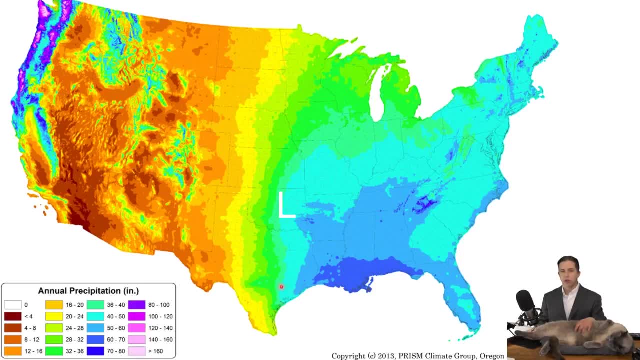 If you're a low pressure, that means you've got counterclockwise rotation going around here, right. So that means you can bring up moisture, say from the Gulf of Mexico, Bring it in and revigorate your mid-latitude cyclone. 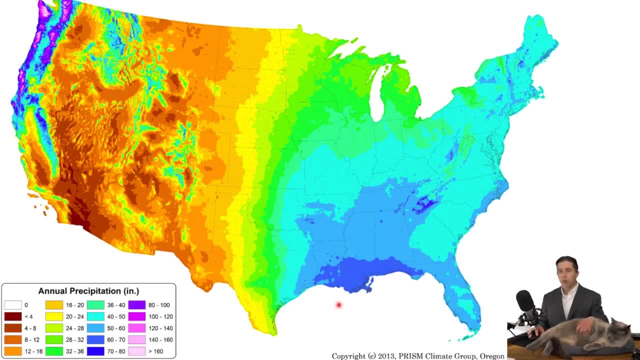 A mid-latitude cyclone- that's kind of all out of moisture- can pick up new moisture, maybe out of the Gulf of Mexico, maybe from the Atlantic, and generate new precipitation. So that's why we see this half of the country suddenly much wetter than the western half of the country. 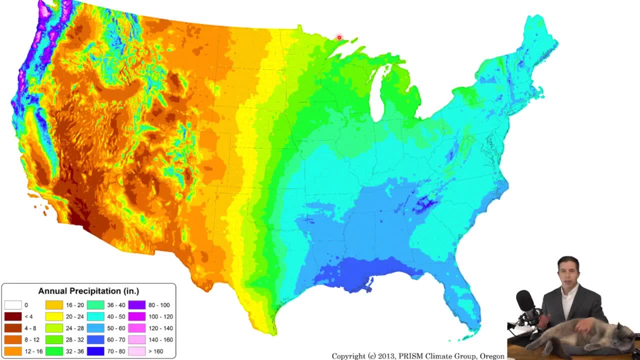 Mid-latitude cyclones can come in from many different directions and we're not getting that deep into it in this class. They may come down from the northeast, called the nor'easter. They may kind of drop in this direction, But they've got many moisture sources out there. 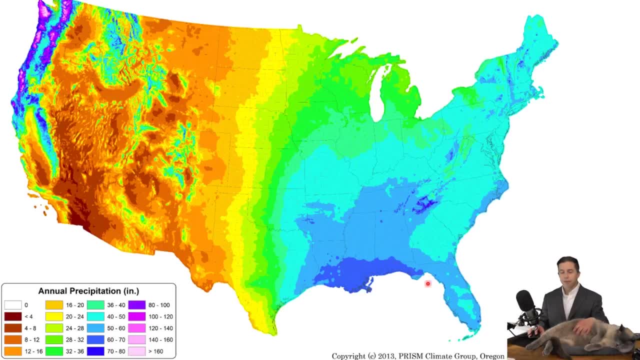 They can pick up moisture from. So overall there's a lot more moisture that can generate a lot more precipitation, both in the winter and the summer. In the winter mid-latitude cyclones, In the summer summertime thunderstorms. They can pick up all that high humidity air down here. 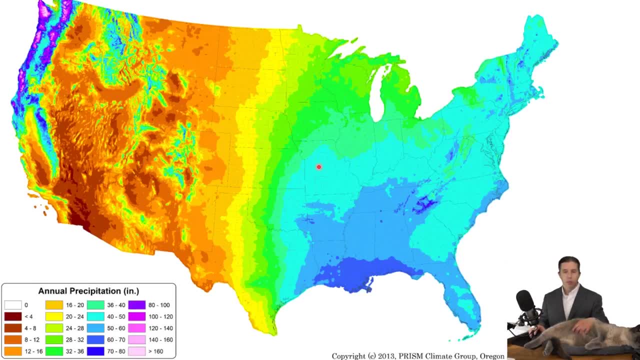 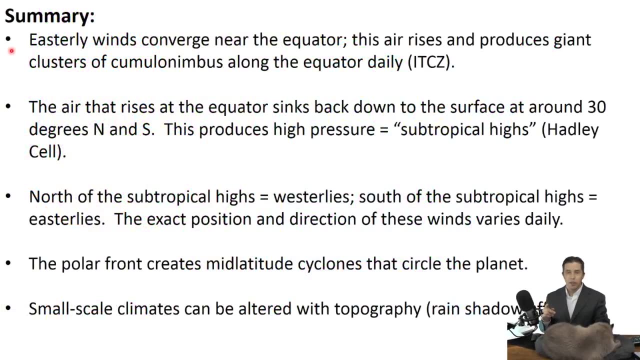 We talked about the tornado alley, That really unstable air forming this part of the country in a lot of summertime thunderstorms. So to summarize, Near the equator we've got easter leaves. There's some north of the equator. 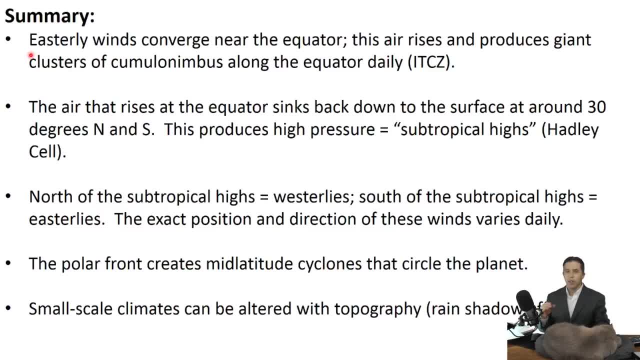 There's some south of the equator, But they're on the collision course usually, And when they collide the wind has nowhere to go but up. When it goes up, it makes a cumulonimbus cloud. When the air gets to the top of the cumulonimbus cloud, it has nowhere to go. 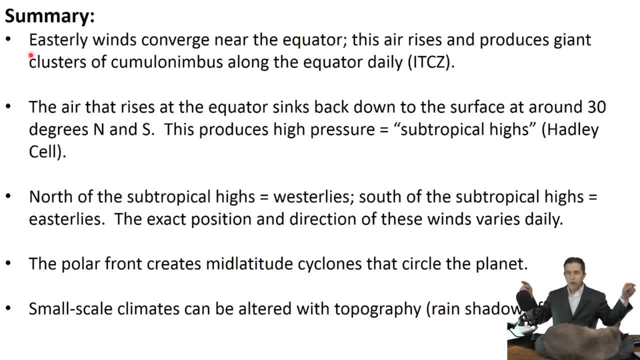 It can't go in the stratosphere. So it goes north and south And it spreads out along the globe until it gets to about 30 degrees north and 30 degrees south. Then at that point It sinks back down to the ground. 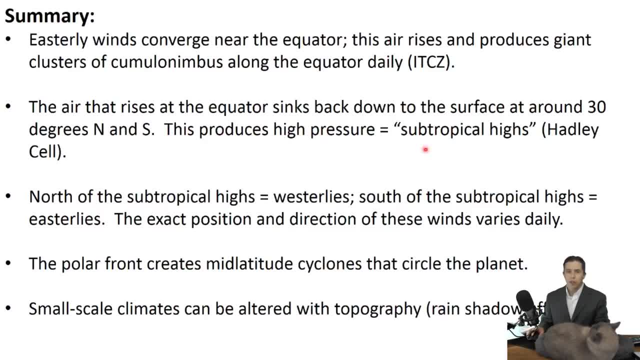 Down to the surface of the earth. That makes high pressure And we call those high pressure areas subtropical highs. That whole loop Rising at the equator, Moving 30 degrees, Coming back down, Returning back to the equator. Eventually that's called the Hadley cell. 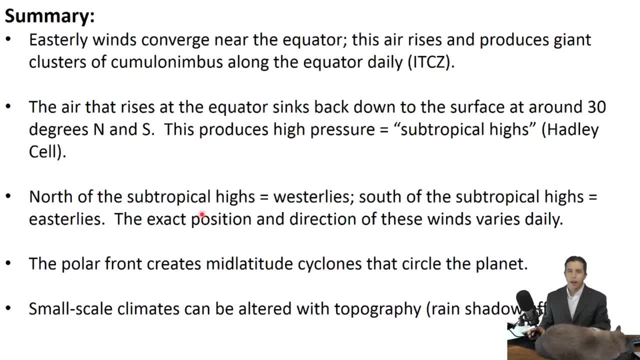 Now, all the winds north of the subtropical highs are mostly coming out of the west- The westerlies. Most of the winds south of the subtropical highs are normally coming out of the east- The easterlies. It's not as simple as it is shown in a lot of textbooks.